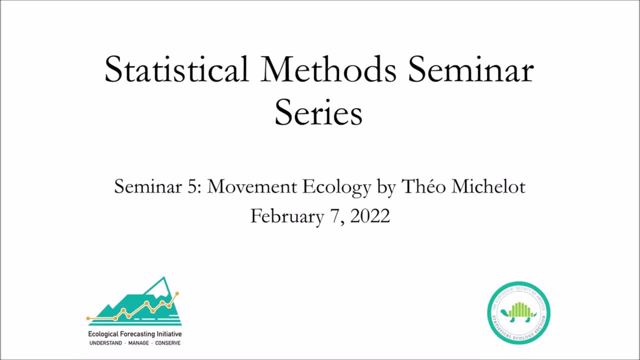 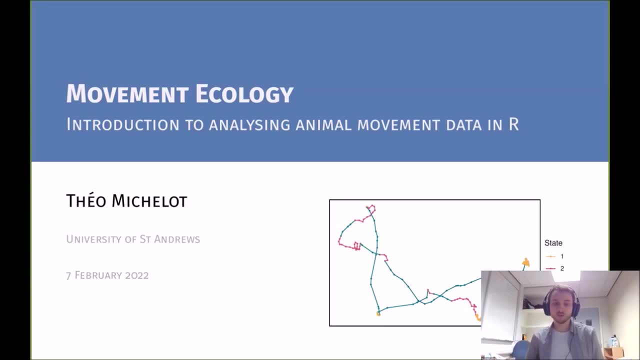 Cool. Thanks everyone for joining, Thanks for the introduction, Thanks for the invitation as well, from the Ecological Forecasting Initiative and ESA. I'm really excited to be giving this talk today. So the general topic I was told to present was movement ecology, And I guess 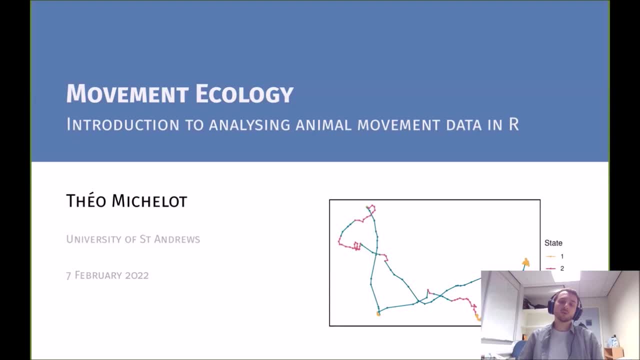 my work really only covers a very small subset of that, And so I'm going to talk about analyzing animal movement data using statistical modeling. I'll go through some slides I have- maybe- I don't know- 20-ish slides that I'll use to present some kind of background about the 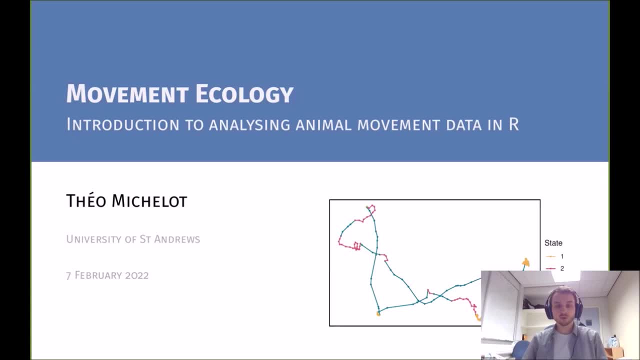 topic and some background about the specific models that I want to talk about today- head Markov models- And then after that, hopefully that won't take more than 20 or 30 minutes, And then after that I'll move on to running through the code that's uploaded on the GitHub. 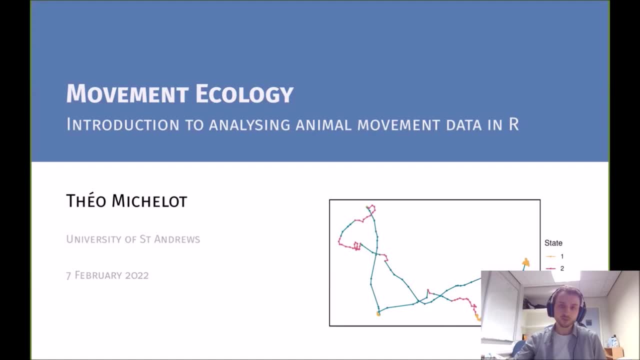 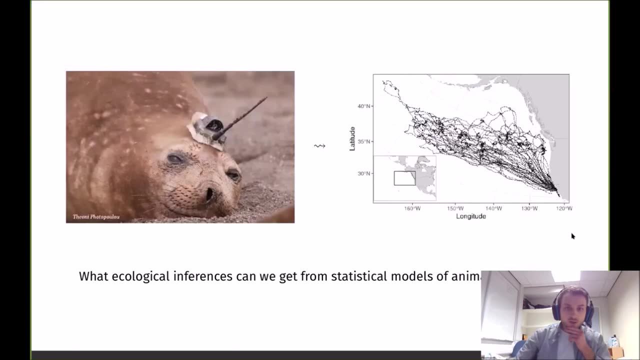 repository and kind of talking you through, Through some of the challenges and practical considerations. Okay, Okay, So a very quick word of background. I'm guessing I don't need to set the stage too much for this crowd, but I work with biologists who go in the field and put tags on animals. Could be an August. 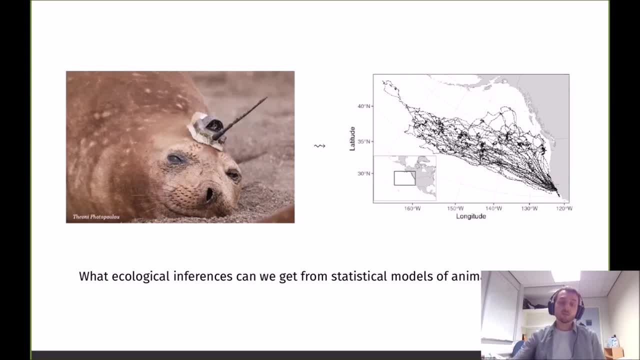 tag could be a GPS color, something like this, And then the type of data that I work with the most often. can someone tell me if you can see my house? I think you should be able to. Yep, Okay, Yeah, this is the type of data that I work with the most. It's kind of trajectories in. 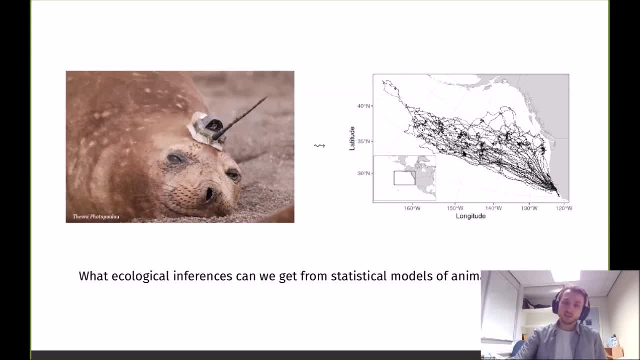 two dimensions, so longitude, latitude and space, and that shows us where the animals went through time. Okay, And maybe I don't really need to motivate you know animal movement modeling or animal movement analysis for you cause? I'm guessing that probably. 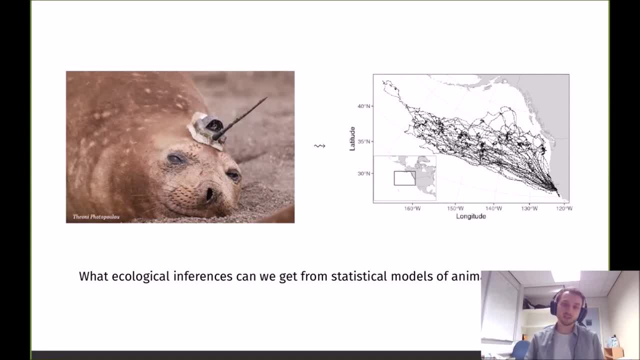 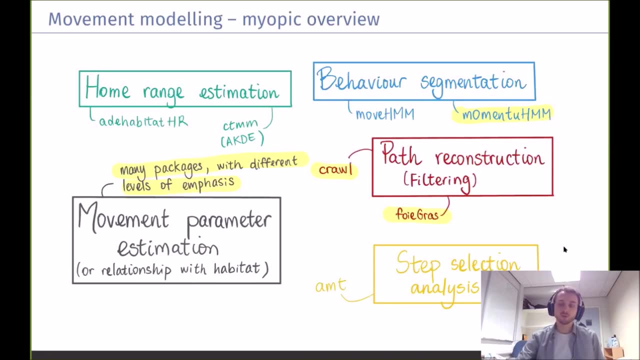 many of you actually like put tags on animals or have at least seen data like these, But there's a lot of things we can learn from these. Yeah, to give a very brief overview of the kind of stuff that statistical modeling can be useful for: 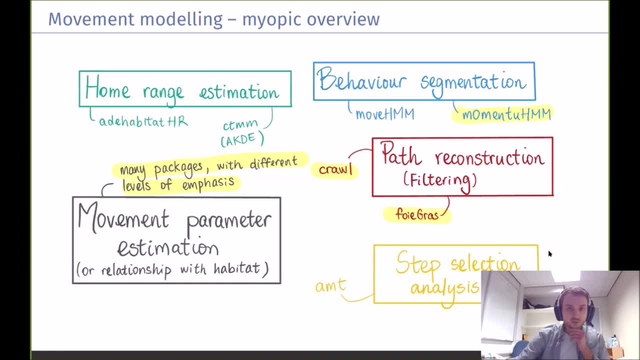 in the context of animal movement data. So this is a very non-exhaustive list of things that you could want to learn about when you have these data and you're using a statistical model. So one possible area of interest is home range estimation, which I think has a 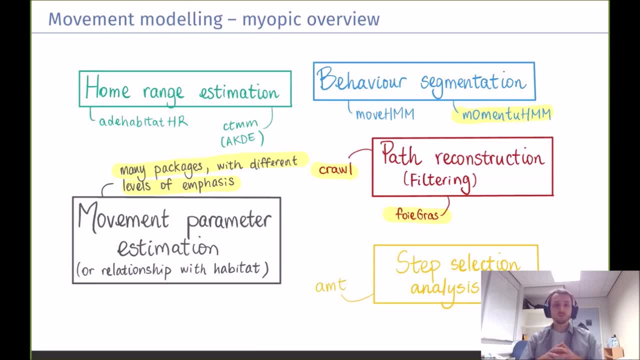 very long history So you could look at this data. you have locations of animals through time and you want to know from these data that only cover kind of a finite duration and you only have observations, say every hour or something. you want to estimate the home range of the animal, what. 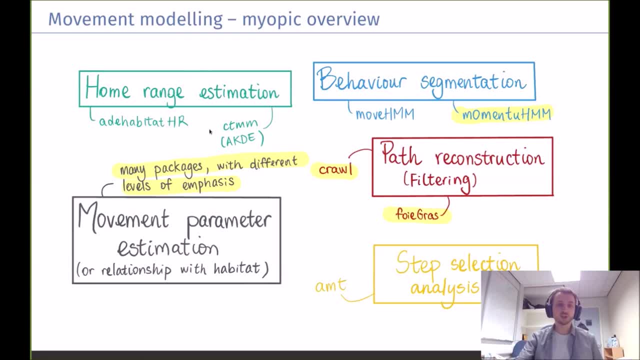 area it occupies, And there's a couple of packages in R to do this. here I'm just mentioning AD, habitat, HR and CTMM. Another kind of unrelated question that you could have is about what I'm going to call behavior segmentation. 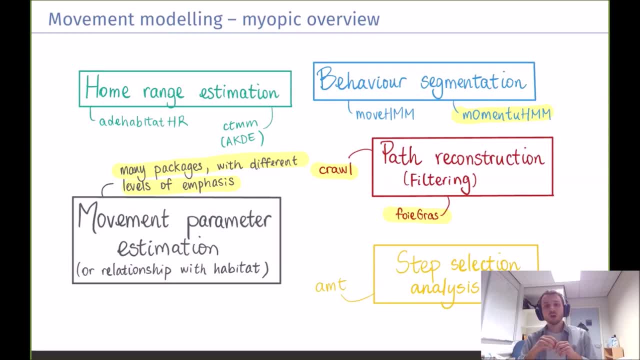 So you have these trajectories of animals and you might be interested to know what behavior the animal was in at each time step through this time series, And this is what models like hidden Markov models can be really helpful for. So that's one topic I'm going to focus on quite a bit throughout. 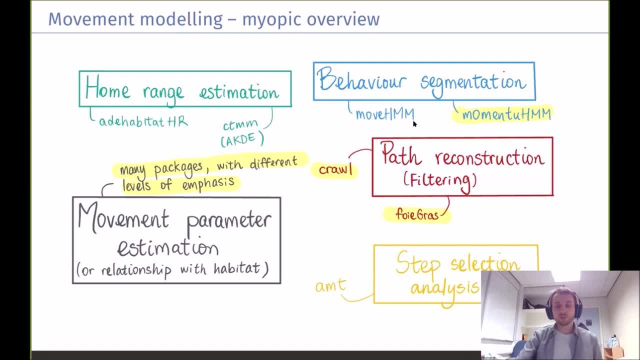 this talk And there's several packages to do this in R. The two that I was going to mention are moveHMM and momentum, and, in particular, I'll focus on momentum today in my presentation. So I'm going to focus on momentum today in my presentation. 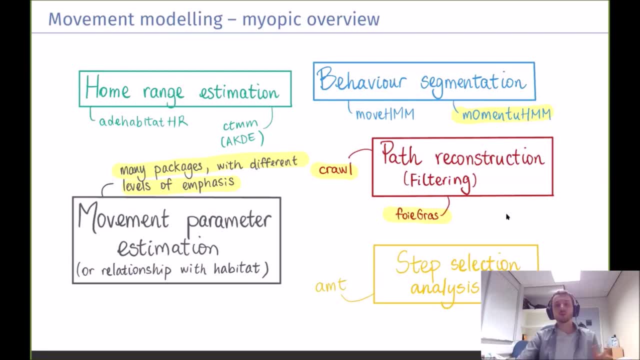 So I'm going to focus on momentum today in my presentation. Another possible question you could have is: how can I reconstruct a path from data that are irregular or that are noisy? So let's say, you have an Argos tag on an animal, so 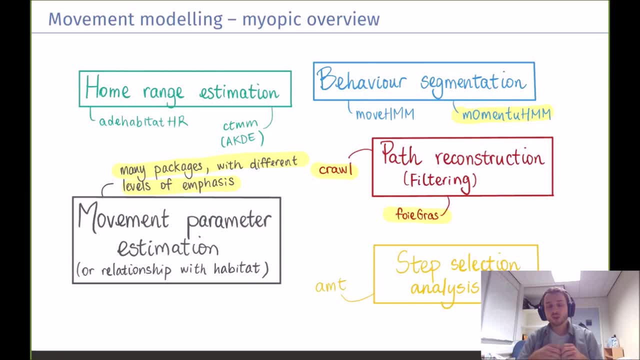 you get points, you get locations from this, but you know that there's measurement error, And so you're going to want to somehow estimate the true location, the true path, reconstruct that true path of the animal from the noisy locations that you have. 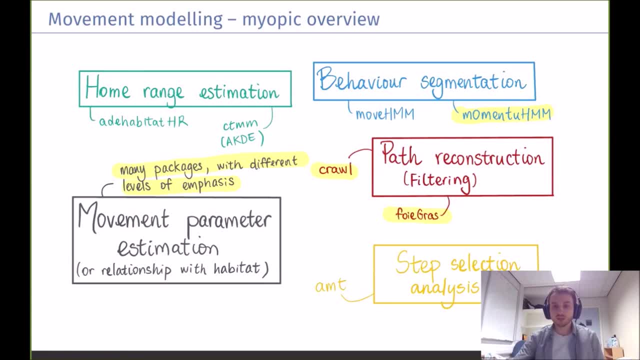 And this is actually a problem that's quite common in statistics in general, especially in signal processing, and that's often called filtering. You want to filter out the noise and just keep the signal, which in our case is the trajectory of the animal, And I'll talk about this a little. 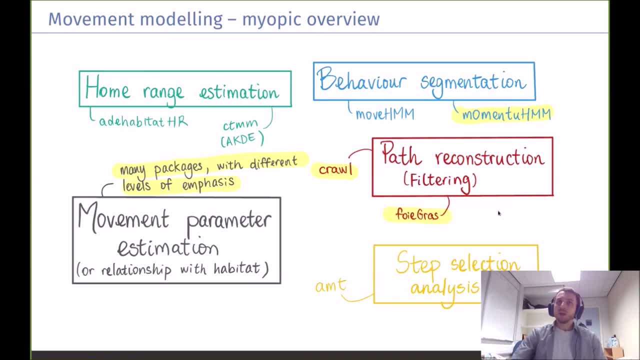 bit as well, more kind of as an aside, to hidden Markov model analysis, because often this is needed as a kind of first stage of analysis, And I'll talk about crawl and foie gras, which are two R packages to do this. Yet another method for. 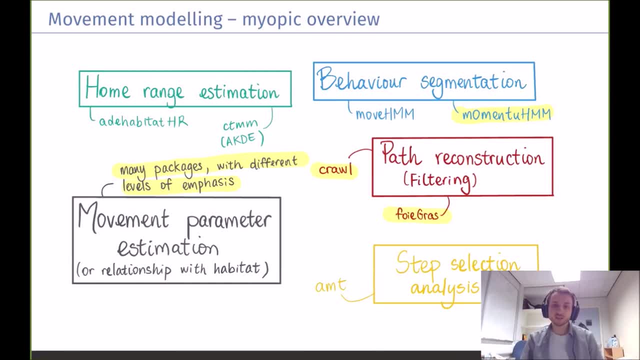 the analysis of animal movement data is a step selection analysis, And here the idea is to try to understand, to combine animal movement data and environmental data and try to understand how animals make movement decisions based on the habitat features around them. And I'm not going 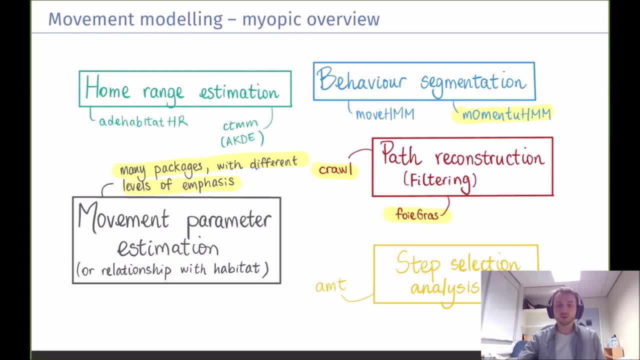 to say any more about this, because I think the next webinar actually in this series will be by Tal Afgar, I think, on this very topic. So I strongly encourage you to attend that one as well. AMT is the package in R2 to do this, And this is a little bit of a kind of a catch-all or. 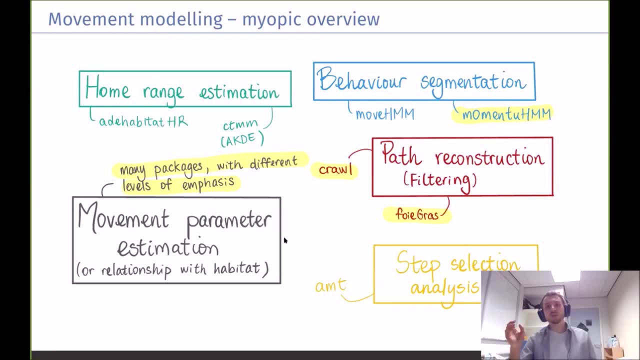 something box: movement parameter estimation from your data. So you have these trajectories. You could want to fit a statistical model to estimate something like you know, the mean speed of the animal or something about how tortuous the movement is or something like this. 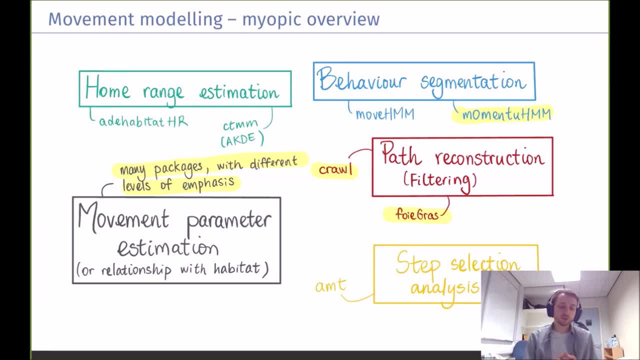 And sometimes those aren't really of interest in and of themselves, but then they're of interest if you're trying to estimate them in relationship with the habitat or in relationship with behavior or something, And we'll talk about this a little bit as well. Okay, 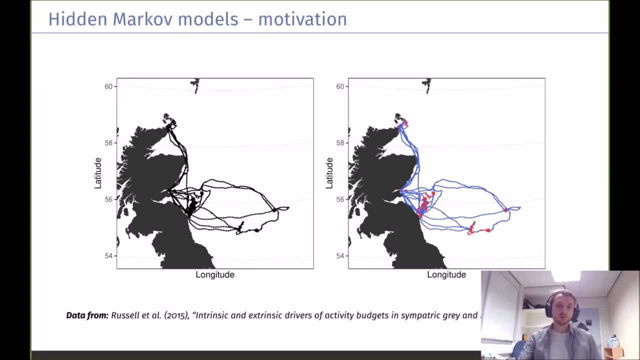 Okay, So that was my very kind of myopic review of a few things you might want to do with statistical modeling, And now I'm going to give an introduction to hidden Markov models specifically for the analysis of animal movement data. Okay, So this is a track of grey seal of the 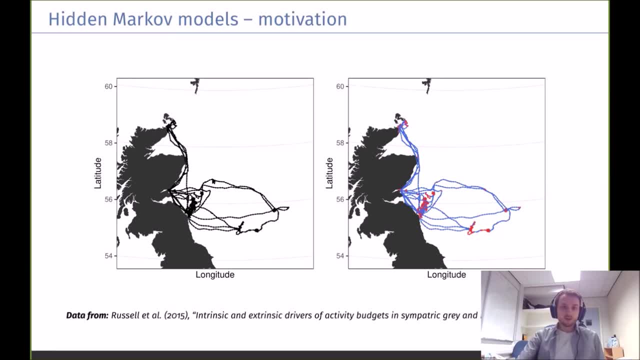 East coast of Scotland And we're just looking at the data here on the left and you could notice that there's different types of movement. So in kind of modern data sets that can span, you know, weeks or months or even years, the data isn't really homogeneous. 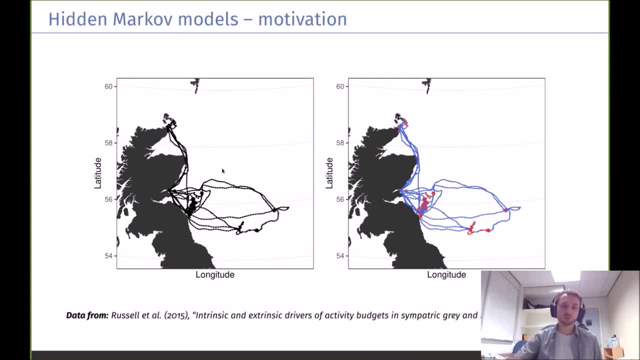 through the movements or isn't really homogeneous through kind of these long time series. So sometimes the animal is going to move more like fast and directed, Sometimes it's going to slow down and move in a more clustered way And, from a biological perspective, the intuition behind this, 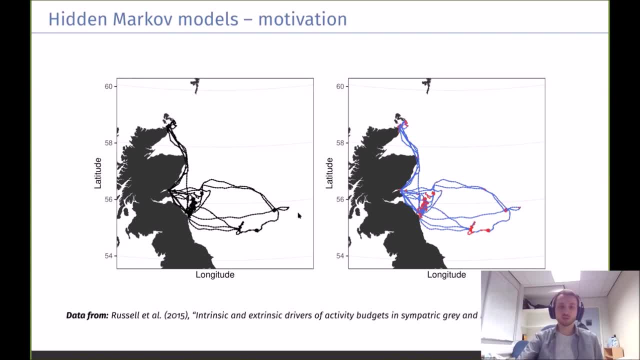 the animal over the course of a couple of months, which is what this time series lasts. it's going to switch back and forth between different behavioral states. sometimes it will be foraging, sometimes it will be resting, sometimes, you know, traveling or something, and clearly these different behavioral states are going to give rise to different movement patterns. 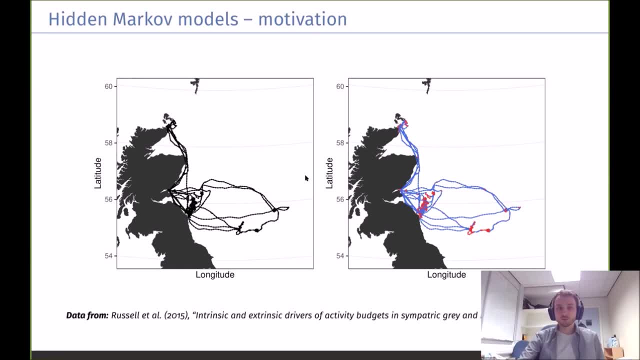 and so this is the, the starting point, the motivation for hidden markov models. we want to try to model animal movement patterns um arising from different behavioral states, from different kind of types of movement. and here on the right i'm showing a possible kind of um estimated classification into two, two, two states, where one of them is kind of fast and 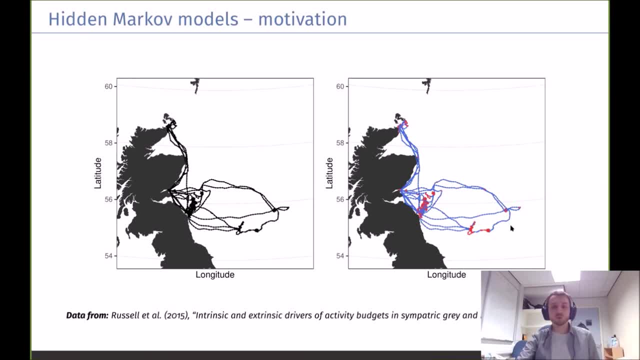 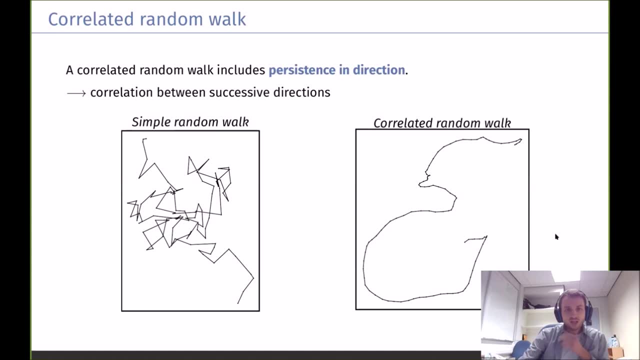 directed. the other one is slower. maybe the slow one could correspond to something like foraging or resting or a combination of those. okay, okay. so, before we come back to these kind of behaviors, i wanted to give um a short introduction as well, about the building block, uh, or the. 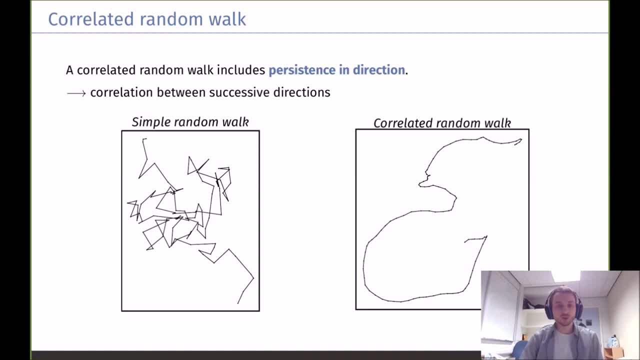 most important part of the building block, uh, or the most important part of the building block most common building block for these models, which is the correlated random walk. so, within each behavior, we're going to assume that the animal follows a correlated random walk and a correlated random walk is a pretty simple statistical model, but it's quite convenient for. 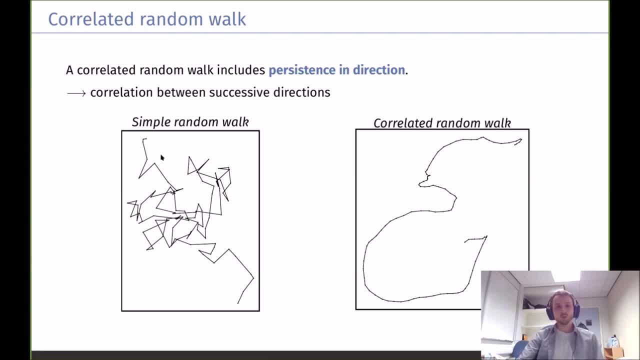 us because it includes persistence in direction. so on the left here this is kind of a simple random walk that doesn't have correlation in the direction of movement and you can see it's kind of all over the place and this is a correlated random walk and it looks a little bit more like what we would. 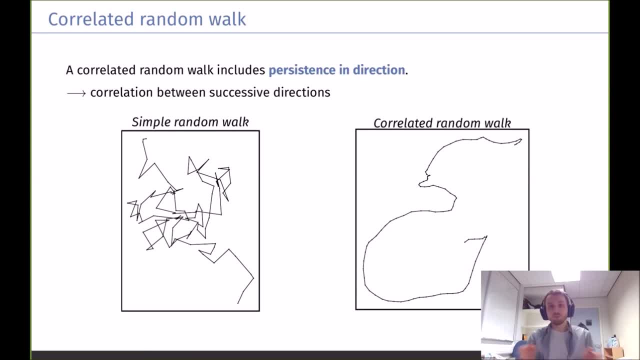 typically observe in animal movement data. animal movement data often because, like on the gray seal example from the previous slide, because animals tend to persist in direction, you'll often have things like this, where there's a persistence in in the movement and- and this is where the correlated random walk helps us capture okay. so how do we model correlated random walk? there's. 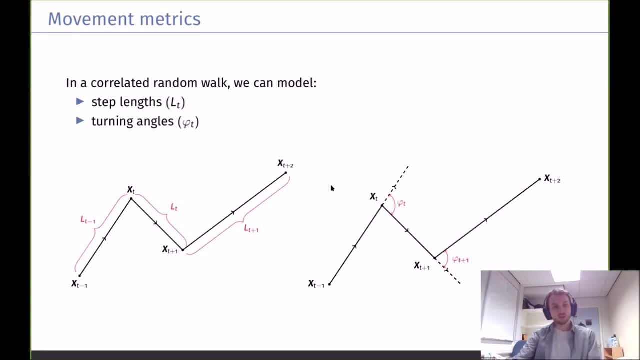 several ways to do it. um, one common one that i'll talk about in this talk is, uh, using step lengths and turning angles. so step lengths are distances between successive locations, right, and it's a measure of something like the speed of movement. a longer step corresponds to faster movement, and we can model: 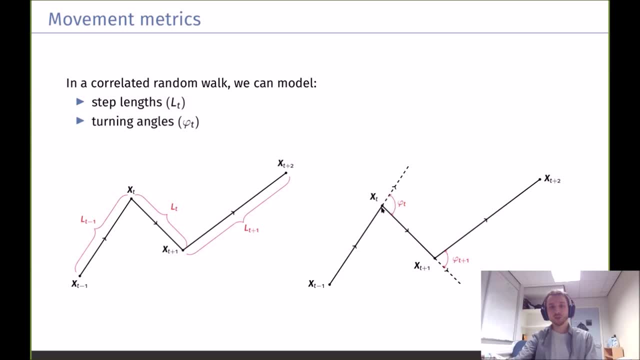 the turning angles, which are the changes in direction. so if you think about two successive steps, two successive segments in that trajectory, the angle between them is the turning angle and it's a measure of how, how i guess torches, how sinuous the movement is if the turning angle is very small, if it's very close to zero. 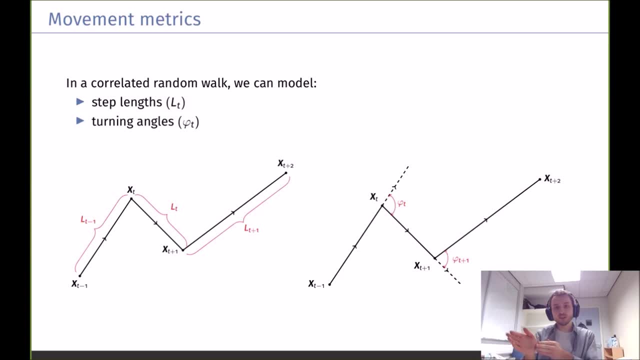 it indicates that the animal is going to persist, persisting in its current direction, and so it's going to be strong persistence, whereas if you have a lot of large turning angles, it means the animal keeps kind of going back and forth and it's kind of what gives rise to those most. 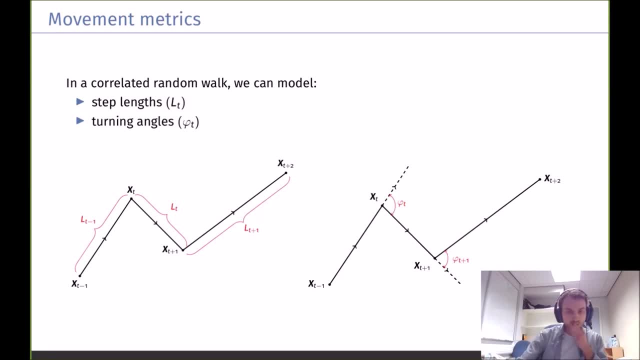 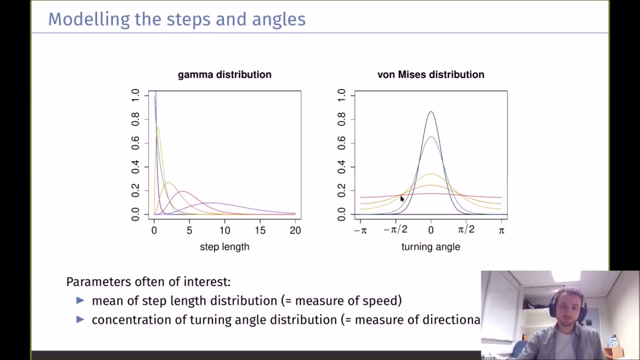 clustered movement phases. okay, okay, so step lengths and turning angles. so in practice we're going to model them with probability distributions. so a step length is, um is a positive number, right, or at least a non-negative number, and so we can use something like a gamma distribution to model step lengths. and here, 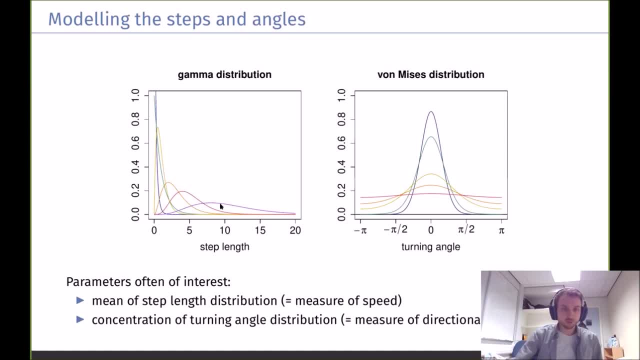 i'm showing a few examples and the densities of gamma distributions corresponding, i guess, to different distributions of step length. so, for example, the purple line here suggests that most step lengths would be between- like i don't know- 5 and 15 kilometers or something that captures. 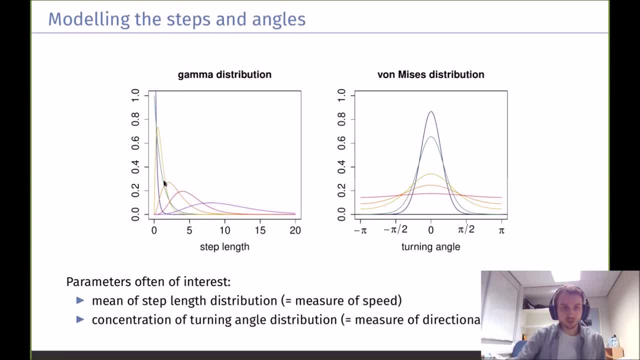 kind of long steps, whereas if you look at- i don't know- this yellow line over here, it suggests that most of the steps are going to be somewhere between, you know, zero and three kilometers or something, so it corresponds to slower movement. okay, so by changing this distribution of step lengths, you 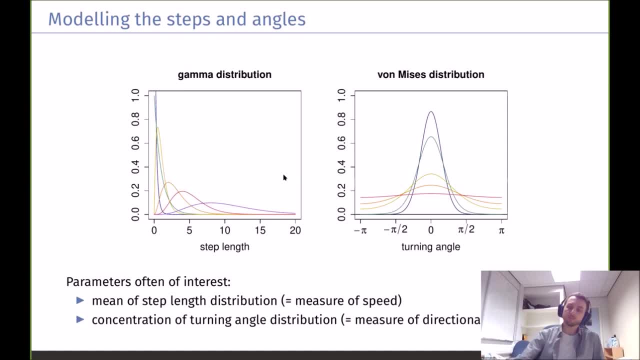 can capture different uh kind of speeds of movement and then turning angles. so turning angles are defined between minus 180 and plus 180 degrees- right, that's kind of on a circle- or between minus pi and pi, and so we can use something that we call a circular distribution. these are probability. 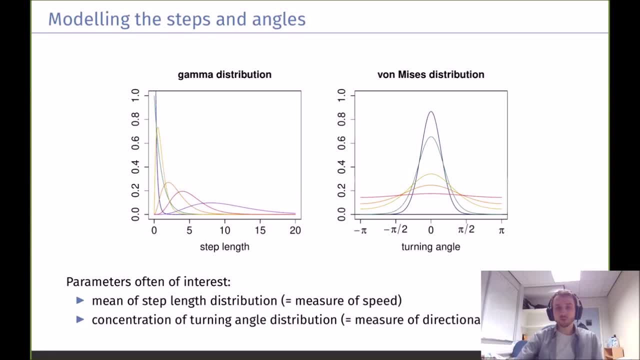 distributions defined on the circle, and one example is the von mises distribution that i'm showing here, and this captures something about how directed the movement is. so, for example, the the dark blue line, here it's quite peaky around zero, so it means that most turning angles are going to be close to. 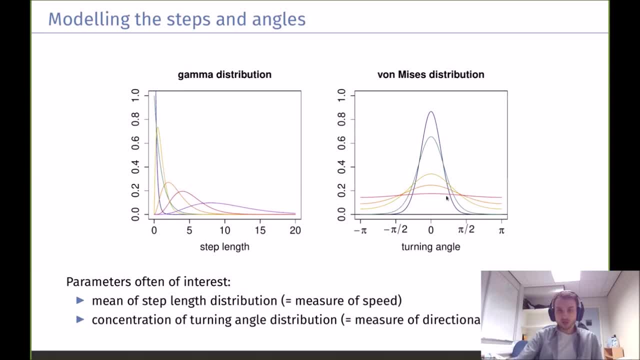 zero. so it means strong directional persistence. on the other hand, the red line, that's kind of flat here. it means that there'll be just as many turning angles that will be, you know, like pi as minus, pi as zero. it means the animal has kind of the same probability of going in any direction. 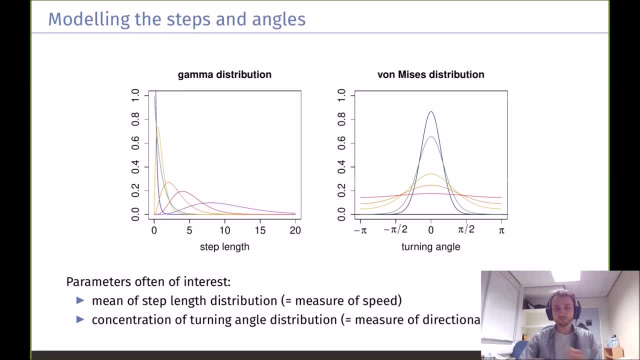 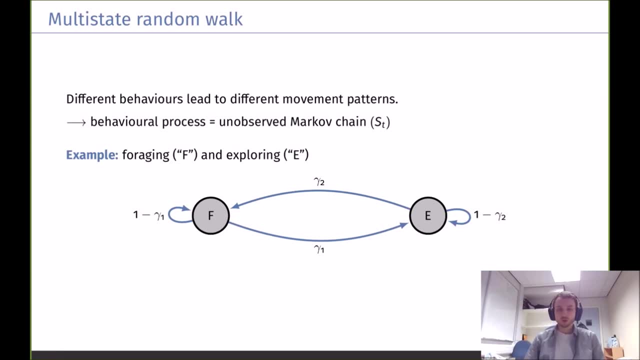 at any time point. so there's no persistence in direction, okay, okay. so that was kind of the very brief overview of correlated random walks and how we capture the speed of movement and the the persistence in direction. i know i want to quickly come back to the, the hidden markov model component of it, like the different behaviors that we observe. 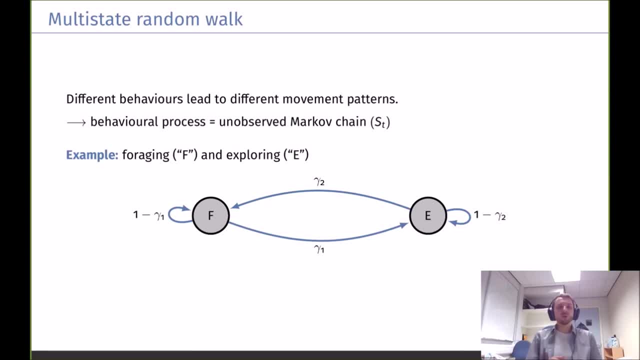 so, as i mentioned, the starting point is to say that we want to assume that different behaviors lead to different movement patterns. the animal isn't going to move in the same way when it's foraging and when it's moving. it's going to move in the same way when it's moving and when it's. 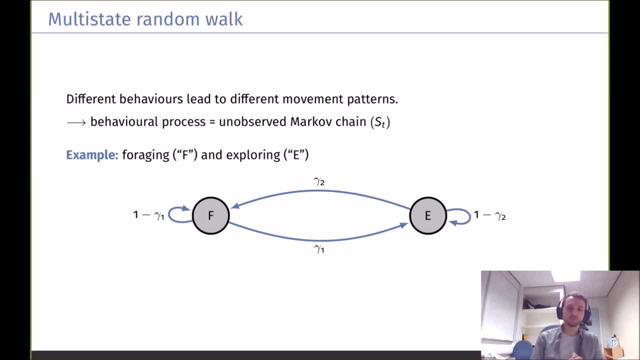 resting and when it's traveling or something, and so, mathematically, what we use to model this is a model called the markov chain, and this markov chain is a process, a temporal process that's going to model the behavior of the animal or be a proxy for the behavior of the animal. 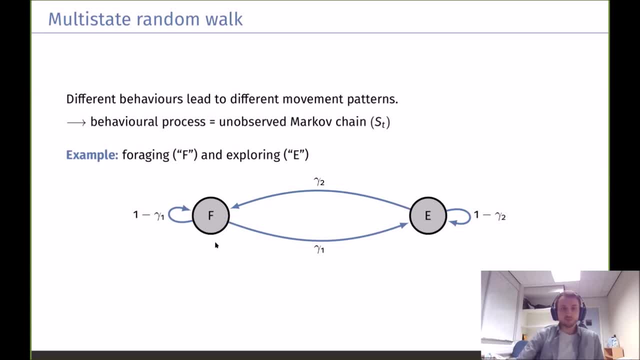 so here is a simple example of how a markov chain works. so it's an example here with just two states. we could have potentially more, we could have three, four or five states, but here we just have two of them: foraging and exploring. markov chain then models the transitions between those states. 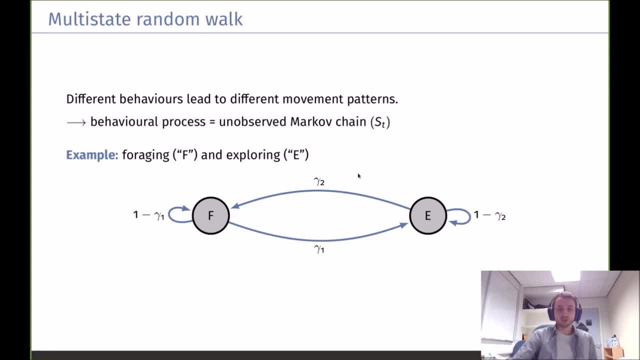 using transition probabilities. that i'm denoting here is gamma one and gamma two. so let's say that the animal is foraging, then it has a chance gamma, a probability, gamma one in the next time step, so say in the next half an hour or something, to transition to exploring and and if it, 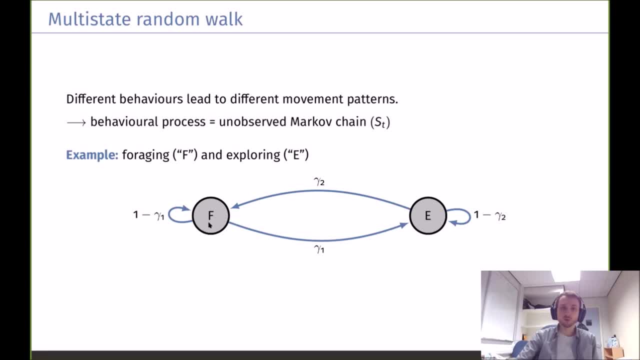 doesn't, then it's just going to stay in the foraging state, so it might be foraging for five, five, five hours and then at some point it will transition to exploring and be exploring for one hour and then transition back to foraging, and this is how the model works, okay. 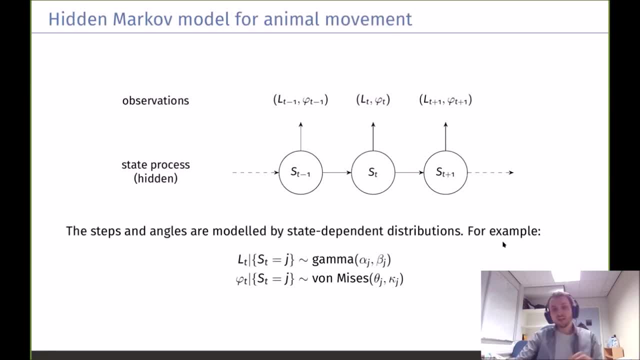 so now that we've presented kind of the building blocks, this is the, the structure, that, the way that the structure, the overall structure of a hidden markov model is often presented. so what this graph here is showing are two processes. the first one is the state process. 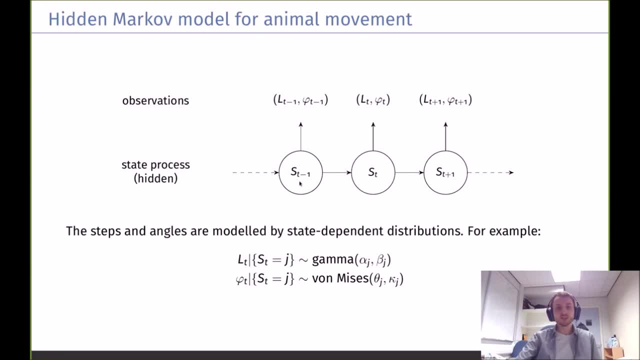 that's here at the bottom and this one is the proxy for the behavior of the animal. so it's like this could be foraging, foraging, foraging, then exploring, exploring this the the arrows show should time here. this is: state at time t minus one. state at time t state. state at time t plus one: okay. 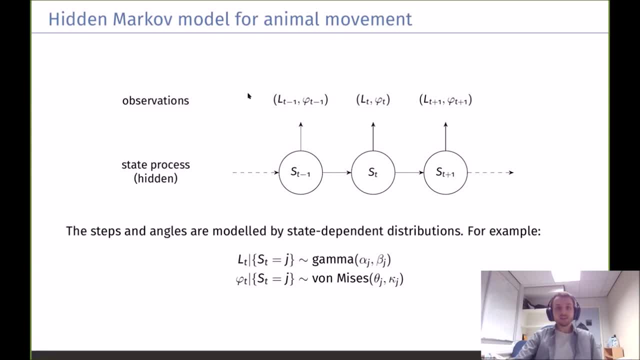 and then these, uh, these here at the top show the observations. so in this case it's one step length and one turning angle for each time point. so these are the step length and turning angle at time t plus one. and then these are the step length and turning angle at time t plus one. 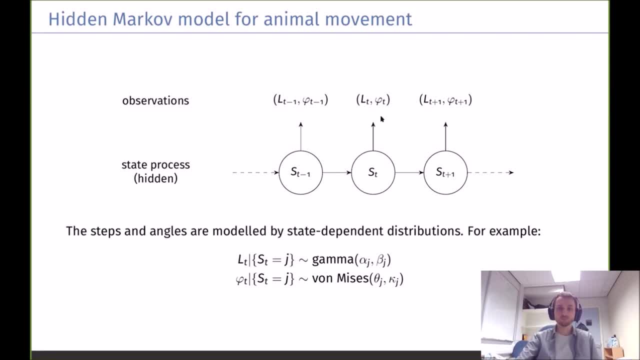 t minus one step length and turning angle at time t, etc. And these arrows here suggest that or represent the assumption that these observations at time- well, let's look at these. These observations at time t depend on the state at time t. So if the animal is foraging, 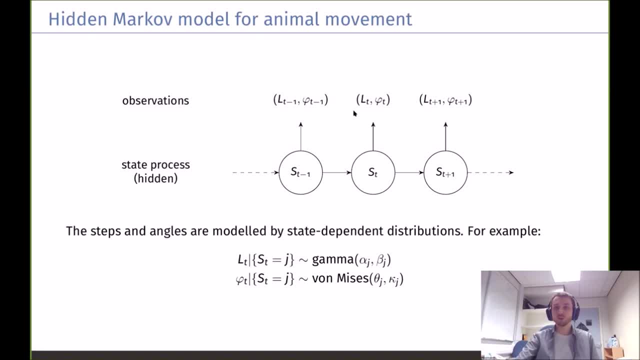 or if the animal is exploring at time t, it's going to affect the distribution of step lengths and the distribution of turning angles. okay, And the way we model this is using state-dependent distributions. So, for example, if we say that the step lengths follow a gamma distribution, 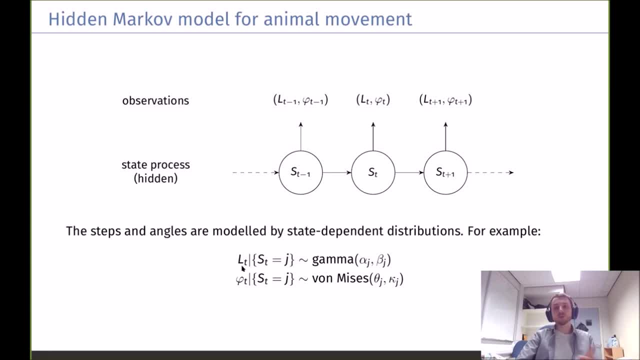 now what we're saying is that it follows a gamma distribution, but a different one in each state. So the distribution of the step lengths- given that we're in state j, j could be exploring or foraging- say- is gamma distributed and these parameters depend on j, So it's going to follow. 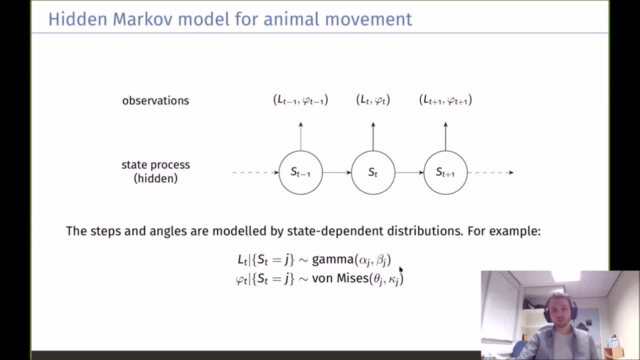 a different distribution in state one, state two. Okay, Same thing for the turning angles. The turning angle at time t, given that the state at time t is j, follows von Mises' distribution with parameters that depend on j, And so this: 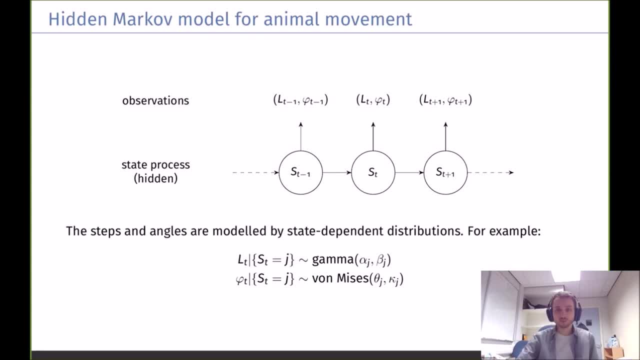 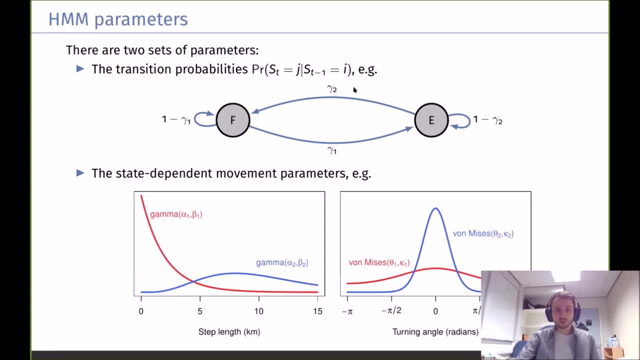 makes it possible for us to model different movement patterns in the different states. okay, Okay, so now we have a model with two sets of parameters: The transition probabilities. so these are the gammas tell us how we're switching between the two or between the. 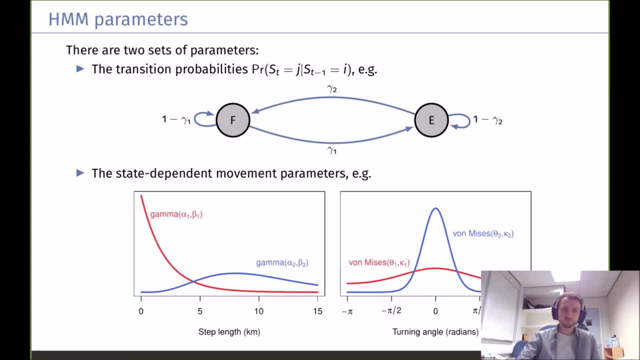 two or three or four behaviors. And then we have a model with two sets of parameters, and we have the movement parameters, which are the parameters of the distribution of step lengths and turning angles. So, for example, we could have some parameters for step lengths for state one. 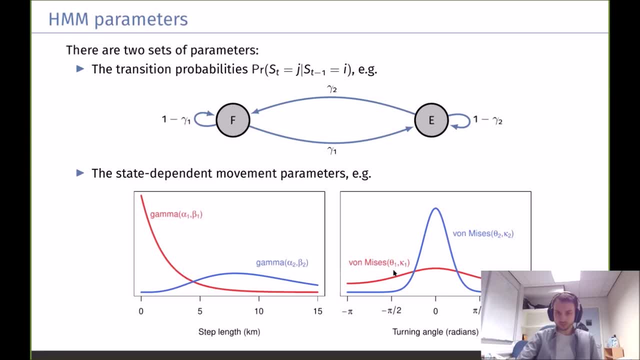 for state two. so these define two different distributions and some parameters for the turning angles in state one and state two, also defining different kind of distributions of turning angles. Okay, And all of these we can estimate from animal movement data when we fit. 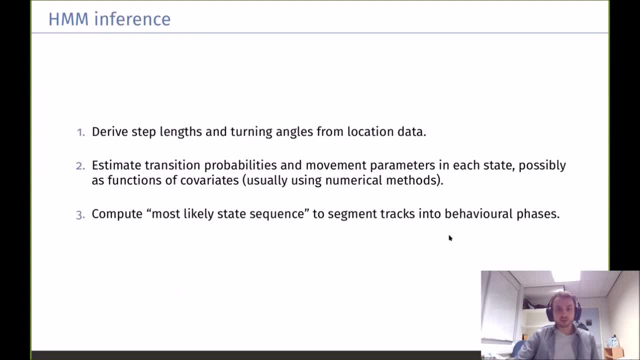 the HMM. So this is kind of a very kind of a core summary of the workflow for these HMMs. You would start by deriving the step lengths and turning angles from location data, and this is straightforward. You can do that. there's kind of geometric formulas to do that. Then you would estimate. 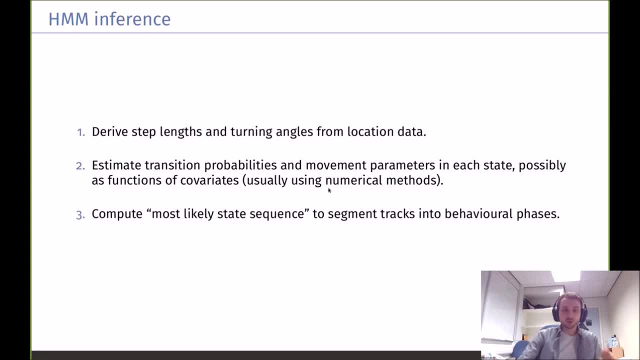 you would fit the model to the step lengths and turning angles and in so doing you're estimating transition probabilities and these movement parameters, possibly as functions of covariates. We'll see that's kind of an extension, And this is usually done using numerical, numerical methods, numerical optimization. 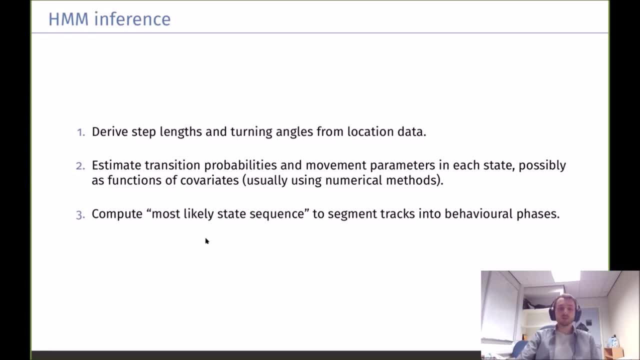 And then often what we can, we can be interested in at the end, once the model is fitted, is to calculate what we call the most likely state sequence. that tells us for each time step what's the most likely state that the animal could have been in So it can you know. we can use that to. 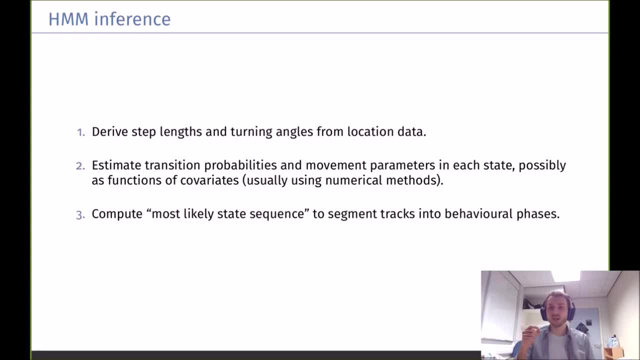 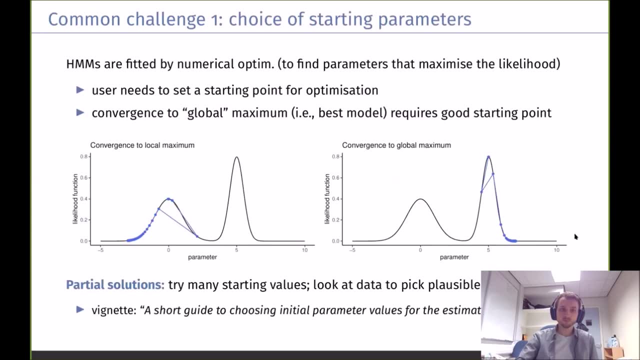 create, for example, that map of Graciel movement that I had in the beginning, colored by the kind of predicted or estimated behavioral state. Okay, Okay, So, Uh, I wanted to briefly talk about a couple of common challenges in applying these. 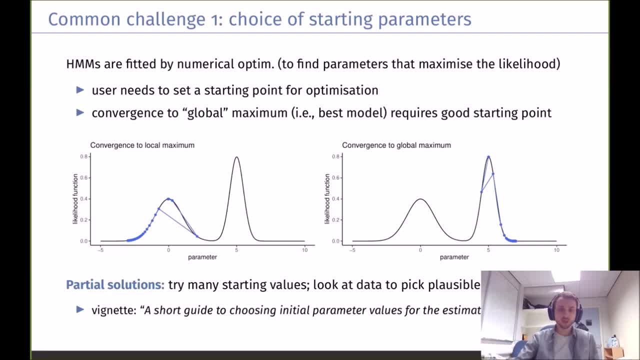 models before I get into the code Um. I'm realizing that I'm going quite fast overall This. I hope that's fine, I hope. I hope it's still kind of making some sense and I hope they will make sense once at least- once I go over the code in more details and talk about these things again. 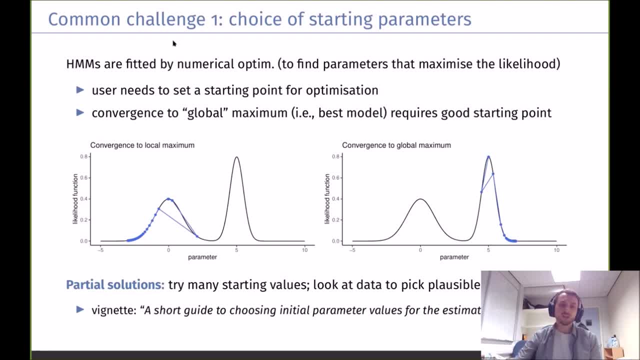 Okay, Okay. So, uh, first challenge, that uh practical challenge that a lot of people have when applying, is the choice of starting parameters, and I'm going to explain what I mean by this. So these hidden Markov models we fit by numerical optimization, so it means we're evaluating a. 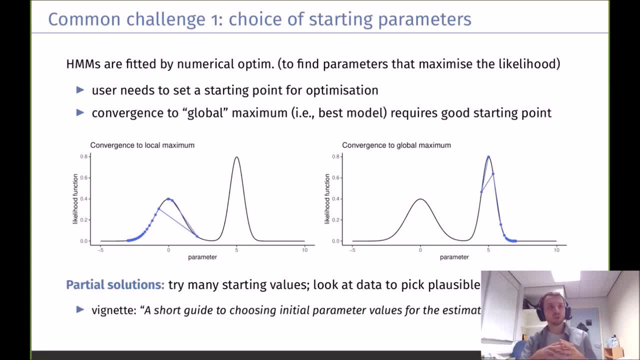 function that we call the likelihood, and the likelihood measures how plausible the data are for a given set of parameter values, and then the what R, or what the software is going to do, is that it's going to try a whole bunch of different parameter values and try to find. 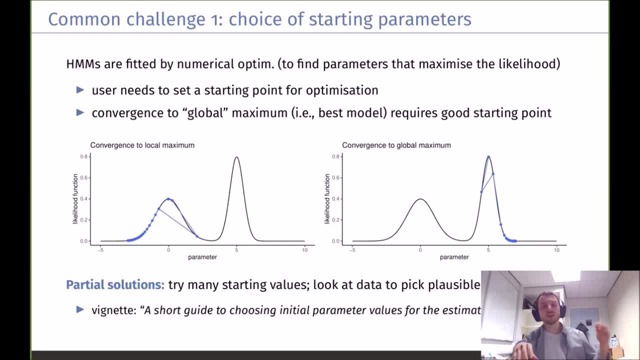 the parameter values that maximize that function, that make the data look the most plausible, right? Michael bayerinya, Teraks Democracy Lab. And to do that we need to use a numerical optimizer. and what numerical optimizers do is that they start somewhere, they choose. going into the calculator, they use some kind of 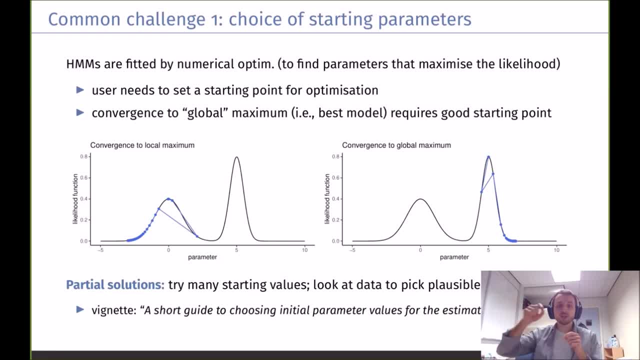 sophisticated rules to decide where to go next and how to explore parameter values in such a way that they'll find the maximum. The problem with this is that they're not guaranteed to work, and here I have a kind of a little toy example. so let's say that this line here shows the likelihood. 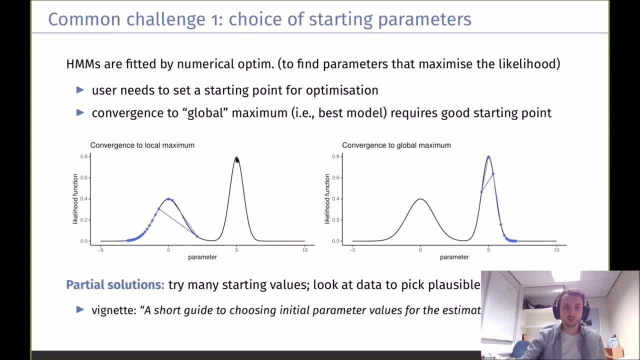 function, and so we're looking for the maximum of the likelihood, which is this point here, and this five would be the value of the parameter that maximizes the likelihood. so this would be our estimated parameter, let's say, if we start off our optimizer here. so we say we don't really. 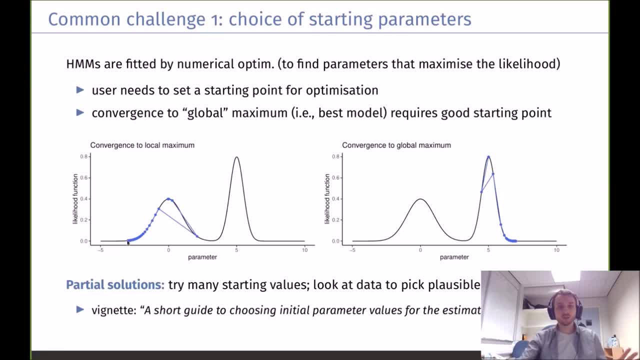 know what the value of the parameter is. so we just say, well, start from here and just try to find the maximum. often, what these optimizers do is that they use the gradient, they use the slope of the function to try to go as high as possible, and then, when it starts going down, they're like 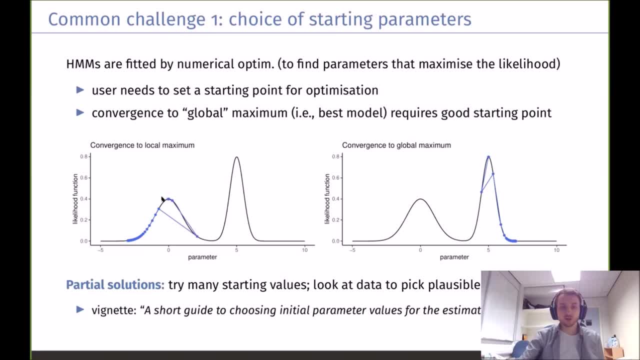 oh okay, i went too far, so i need to go back up. and then they go back up and then they get stuck in the first kind of peak, the first little hill that they, that they encounter. and the problem with this is that now this optimizer here got stuck in this hill when we know that this one was actually 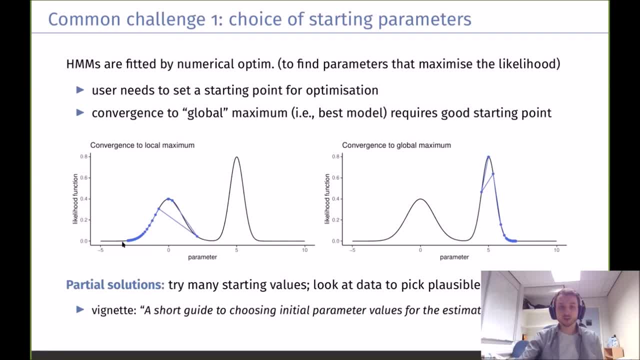 higher. this, this was the actual best model, but this, uh, this optimizer never actually got this far because it just got stuck in this hill. okay, on the other hand, if we started from this side- and why not? right, we could just. if so, just as well, from this side- this time the optimizer would have followed the slope again and then realized it's. 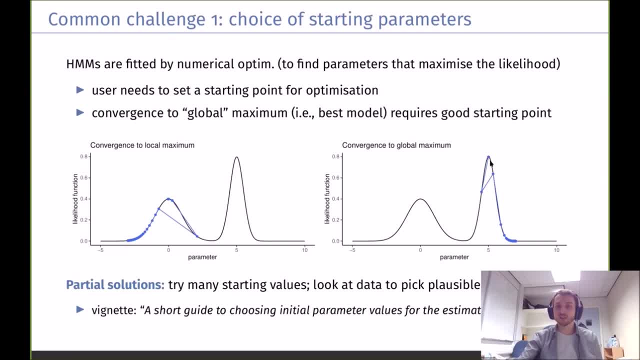 going down and then come back, and then it would have got stuck in this, and that's exactly what we would have wanted. this is the best model. this is the maximum of the likelihood. so in this case it worked and in this case it didn't work. it just depended on the starting value. it didn't. 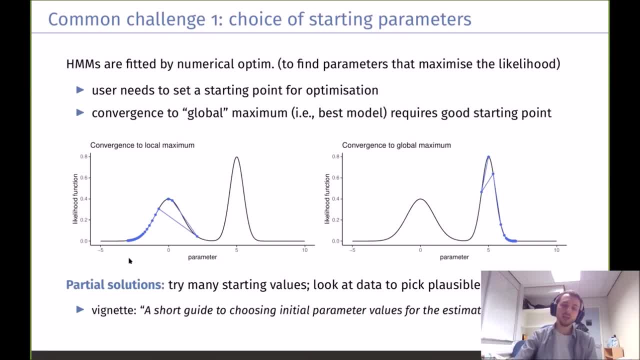 the data are the same, everything else is the same. okay, and there's no general solution to this problem. this is a pretty common numerical problem. a couple of partial solutions: one of them is to try many starting values. so if here we were to try, you know, like every we try setting the, the starting value at every. 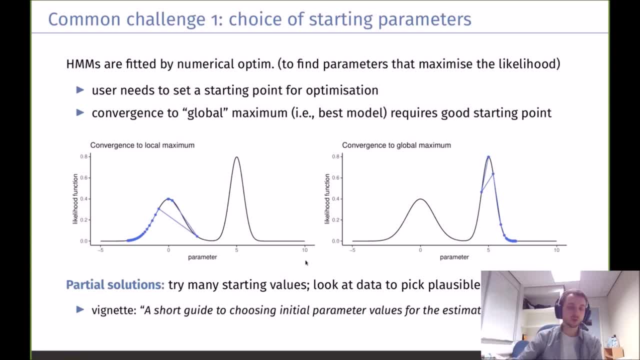 unit or something over this whole range, and then we run the optimizer. of course it's computationally quite expensive, but by the end at least quite a few of them will have found the best model. and then we'll be like: okay, well, we're quite confident that this is the best model and we 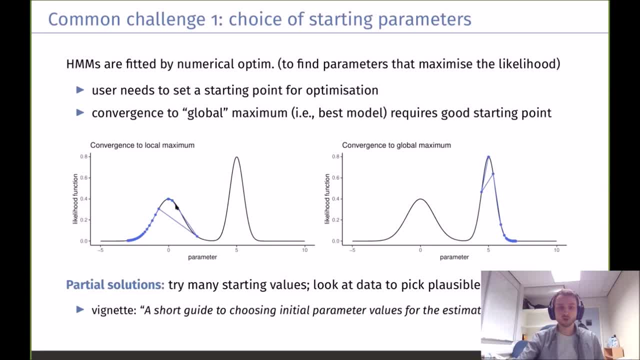 know for a fact that this is this isn't because we found, uh, another parameter that has better likelihood. okay, so that's one thing that's often recommended, and another is to to look at the data and to do that. you want to pick plausible values, you want to try to to pick an initial value. that's. 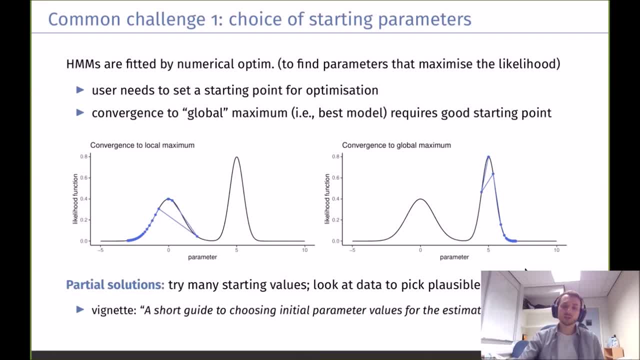 as close as possible to the, to what will end up being the estimated value, and to do that. there's kind of ways to look at the data, kind of exploratory data analysis to do this, you know, in a clever way, and i'm not going to really give much more detail about this right now, but i wrote a. 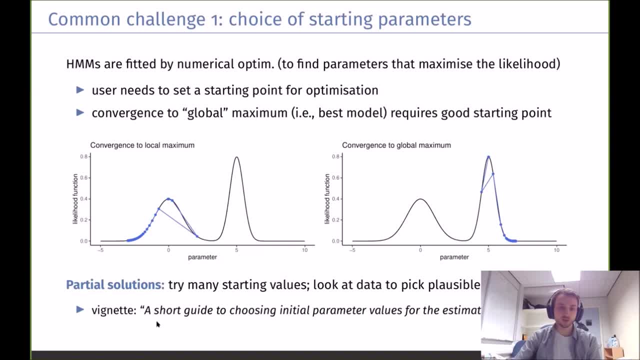 vignette a while ago for the package move, hmm, to do this, and this is the title. you can just google it and you'll find it. and um, it's for a movie, to mem. but it applies just as well to the data as well to momentum. so, regardless of the software you're using, you could have a look, okay. 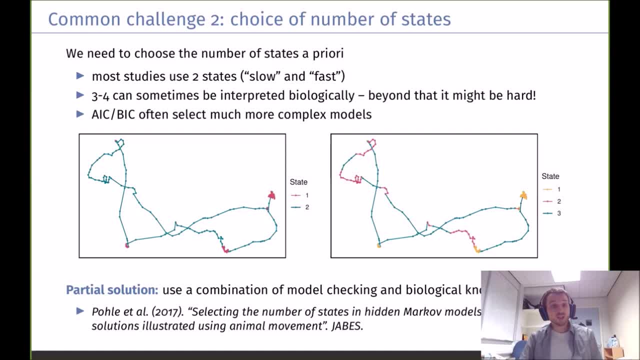 okay, so that was the first challenge, um. another quite common challenge is um is the choice of the number of states. so i mentioned that. you know, the example i took had two states, but you could have three, four, and there's no, uh, there's no general rule for choosing the number of states. 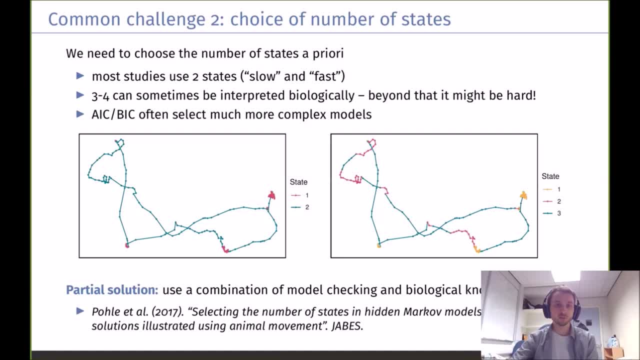 it needs to be kind of user defined before fitting the model. most studies- i think the vast majority of studies- uses just two states, which often end up being kind of slow and undirected movement and fast and directed movement, and i think the reason for that is that, no matter what your data looks, 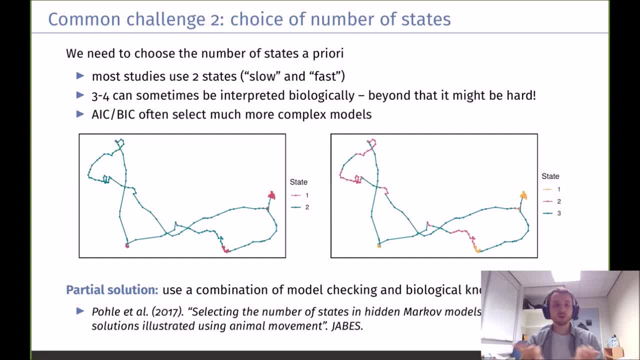 like it's probably it's quite likely that the hmm will pick up two very distinct states that will have kind of convenient interpretations and stuff. but in some cases, i know, with like kind of higher resolution data and stuff, it's not unrealistic to fit models with three, four, maybe even up to like. 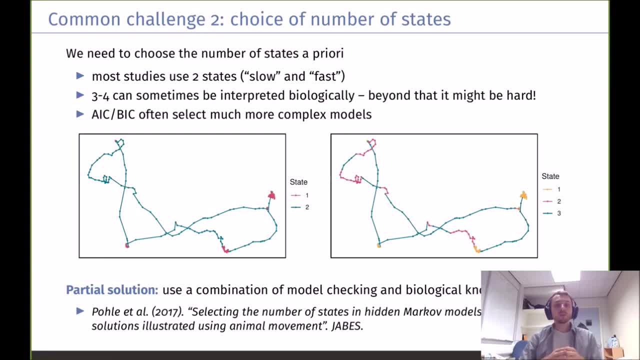 five um states, but it's not unrealistic to fit models with three, four, maybe even up to like five states, and the only problem is that then it will become more and more difficult to interpret. and models with like you, there's almost no way you could, you could, you could interpret, you know. 10. 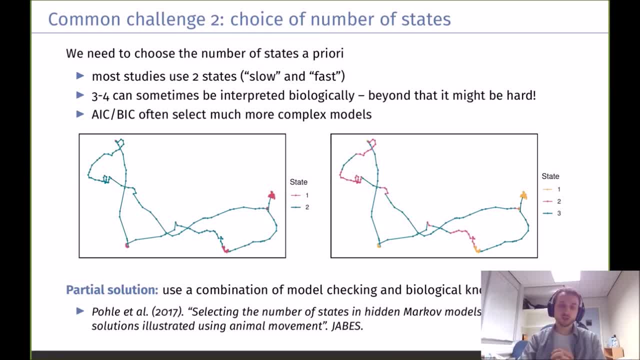 or 12 or 15 states, even though in principle, you could fit a model with that many and one. one reason that this is such a practical problem is that, uh, standard model selection criteria like the aic or bic often select much more complex models than what we would actually want in. 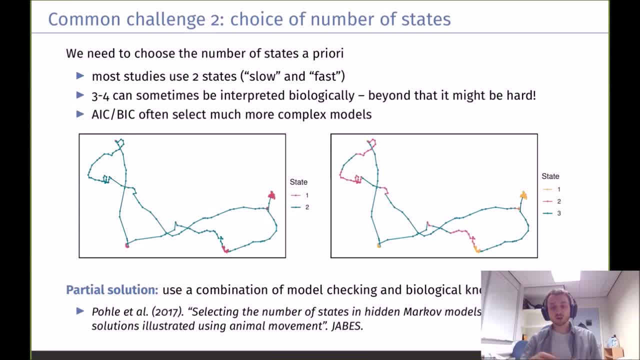 practice, and the reason is that, statistically speaking, when you in include additional states, you explain more and more and more uh patterns in the data, and so aic or bic is going to say, well, that's great, we're like getting better and better at explaining the data. 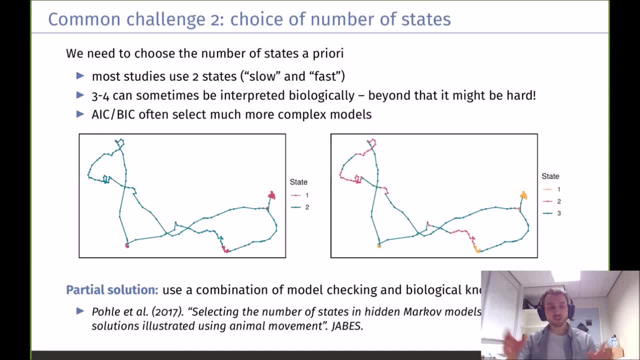 but the cost of that is that then you'll get you know seven or ten or or 15 states, and from biological or ecological perspective you'll have no idea what they mean. so there's just kind of no way you can actually work with those. so the um, a paper came out a few years ago in 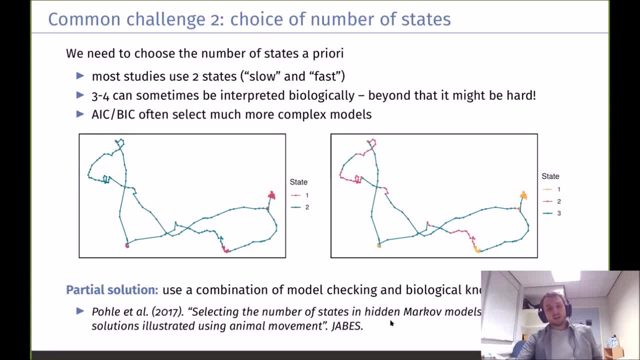 the labes about selecting the number of states in hidden markov models and the. the approach that the the authors recommend is to use a combination of model checking and biological kind of expertise. so the biological expertise is to to choose, you know, if you know that your animal, the animal, 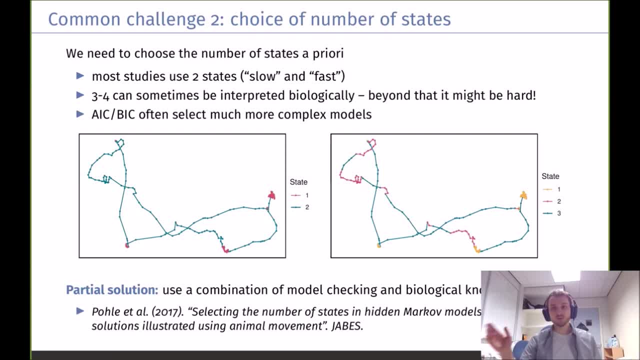 that you're, you study has you know three very stereotypical behaviors that you you think you can pick up from from the movement patterns. then maybe you should just use a three-state model, because at least you'll be able to interpret it correctly. you should probably still use model checking. there's ways to to check that the model fits. 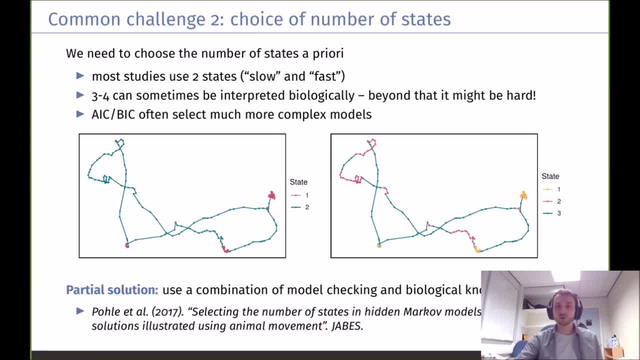 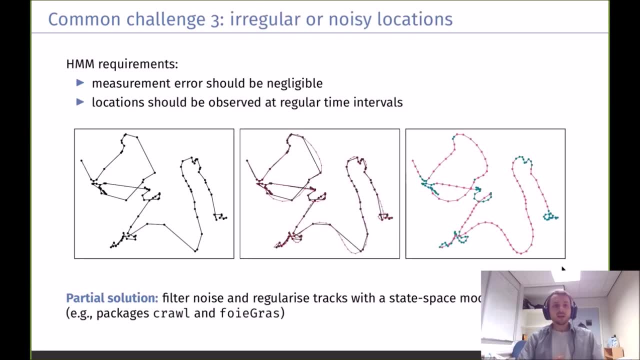 at least kind of decently well, and if it doesn't, you might want to increase the number of states to capture patterns in the data a little bit better. okay, okay. and then a third common challenge. the last one that i'll talk about is irregular or noisy locations. so 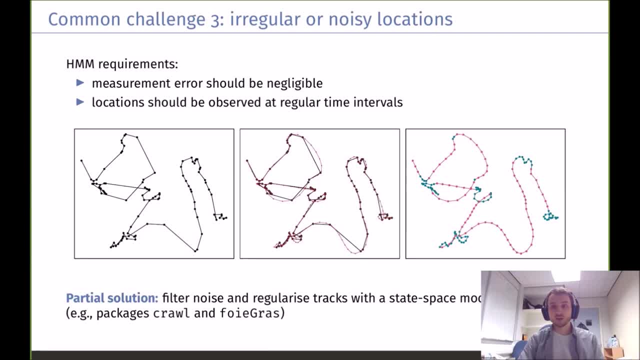 one assumption behind hidden markov models is that there's no measurement error in the locations, because we need to be able to get step lengths and turning angles without error, and that locations should be observed at regular time intervals. and this isn't always the case, especially, i think, for marine biologists. often, you know, you can only observe the animal when 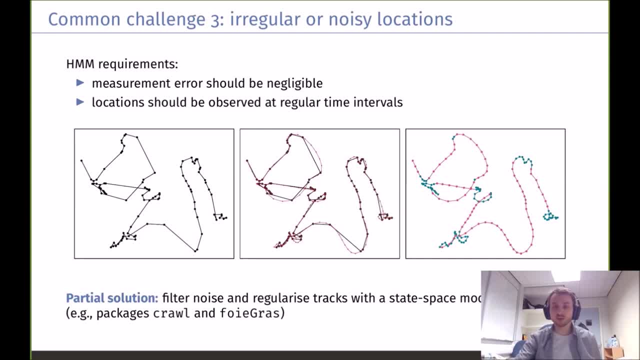 it's surfacing and you don't control how often that is, so you might not have kind of regular time intervals, and the most common solution, or partial solution, to this has been to use first another approach to filter the noise and regularize the track, and usually this is done with 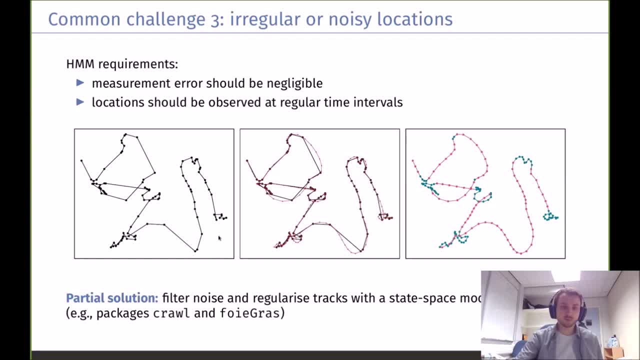 states-based models in packages like crawl and foie gras. so this is your, for your irregular data could be noisy as well. first, the first stage is you use some- um, some state space model to predict it on a regular time grid right, and then you treat that red line, the predicted red line, as data. in the second stage, 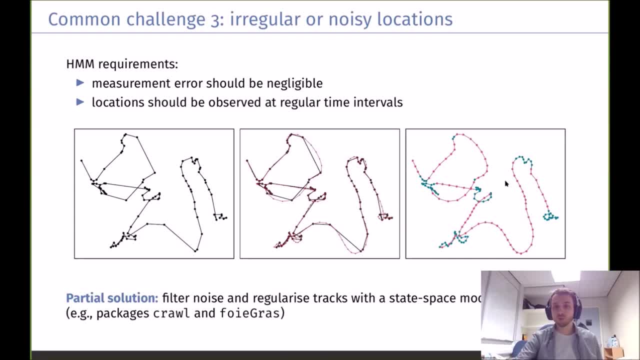 and this is using the hmm to estimate the, the behaviors. okay, one problem with this is that then you're treating that red line as if it was data, as if you kind of knew where the animal was like during this long gap, for example. you assume that you know that it was along this line, but you 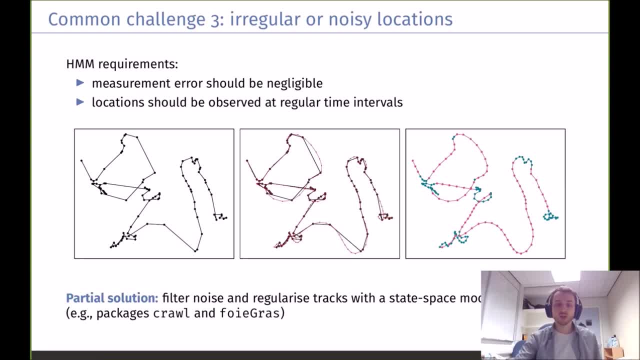 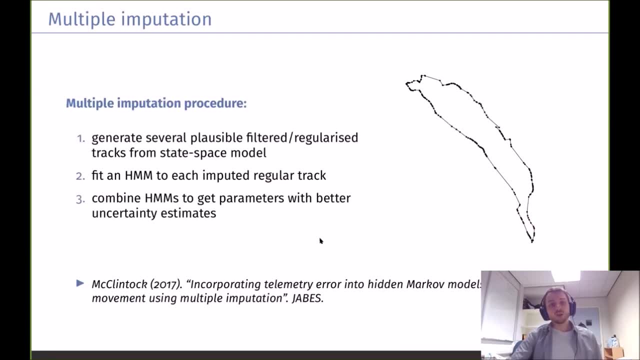 don't actually know that for a fact, right, it's just some sort of like predicted model output that has some uncertainty as well. okay, so, um, another approach, a kind of a slightly better approach that has been proposed recently is called multiple imputation. so here i'm still talking about the case where you have kind of 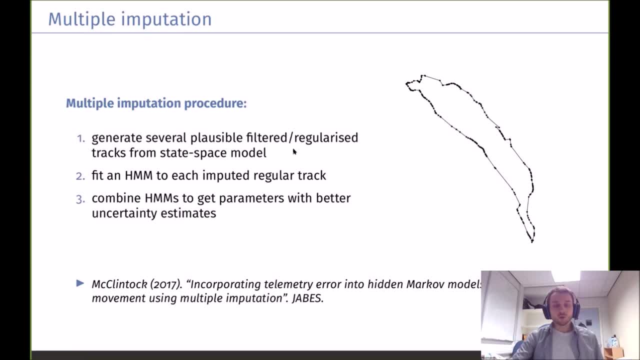 noisy or irregular data and the. the way that multiple imputation solves this problem, or attempts to solve this problem, is by using the hmm to estimate the behavior of the animal and the behavior of the animal, and the behavior of the animal and the behavior of the animal. 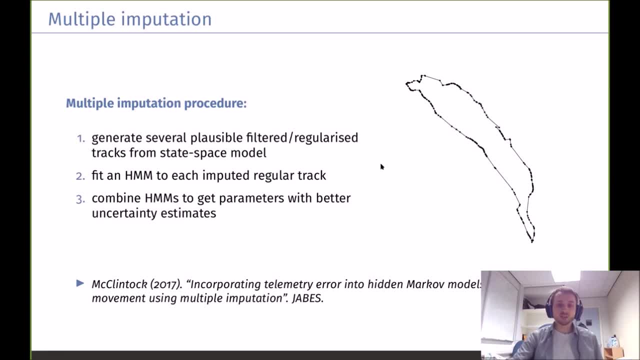 is by generating several plausible trajectories. instead of just one predicted trajectory, you generate several. so here is a. this is a northern first hill trajectory with some gaps, and you can see that in the gaps, instead of just trying to predict one line of where the animal was, we predict maybe 20 lines, and each one of them is going to be kind of a plausible trajectory. 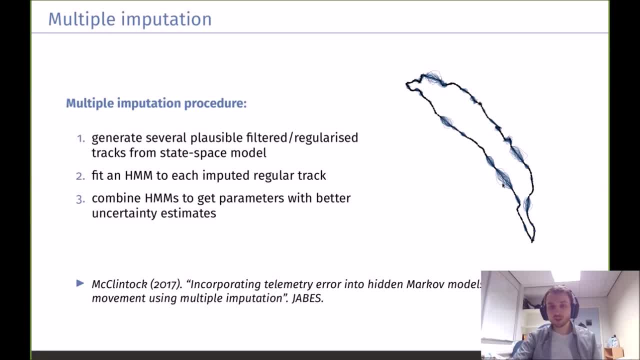 that we'll use it as input for a head markov model. then we'll fit a head markov model to each one of these 20 trajectories. we'll get 20 models, 28 humans and there's statistical formulas then to combine those 28 mms into just one, one set of primary. 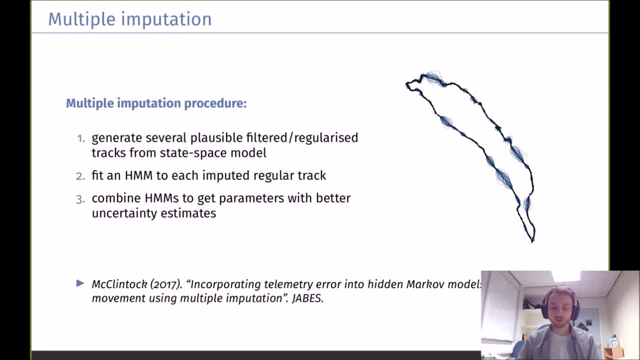 estimates with, with uncertainty, uh, confidence, confidence intervals as well, and, uh, the reason that, uh, we want, we go to the trouble of doing this is that now this con, the confidence intervals, uh, that we get at the end of this procedure, will take into account the, the uncertainty that we had. 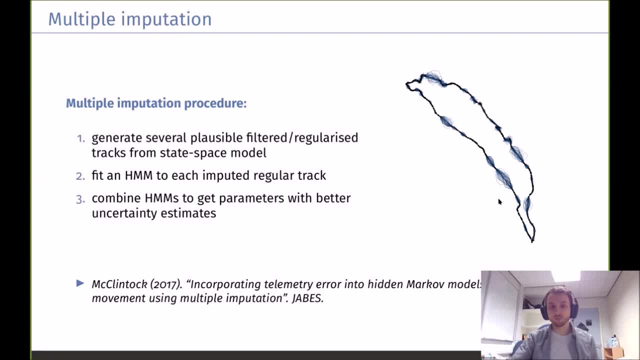 about the location of the animal, uh, in this, in these gaps. okay, it's still not a perfect solution, because we need to have some model to generate those plausible trajectories and if the model that we use for that is not realistic, we're not going to do that very well. we're not going to capture the uncertainty on the location very well. 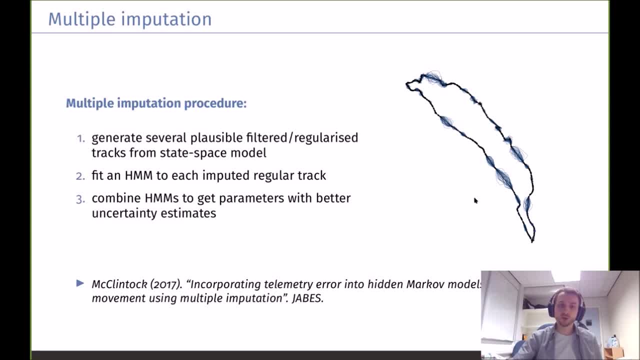 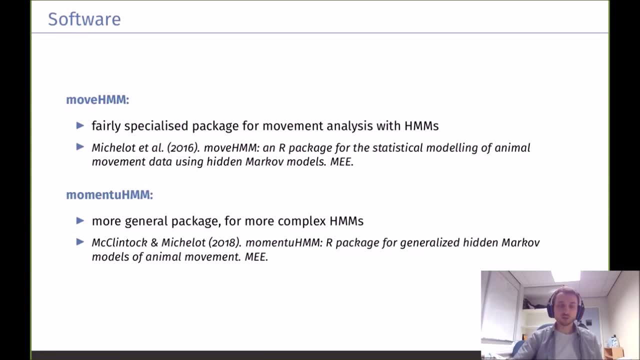 but it's still quite a bit better than just using one trajectory. okay, okay, so this uh takes me to the end of my presentation. i just want to say a quick word about software. um, there's two main packages for fitting hmms to animal movement data in r move. hmm. 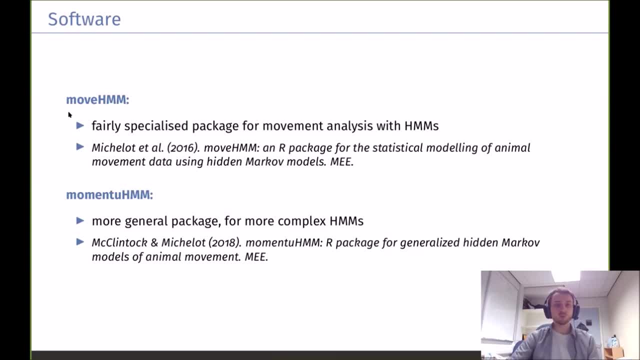 um move hmm, is pretty specialized. we wrote it as kind of a, as simple as possible, the package to fit kind of hmms to animal movement data. so it's quite, i think, quite simple to use. it can still be used basically for all the models that um that i i'm going to present today. so it does have some kind. 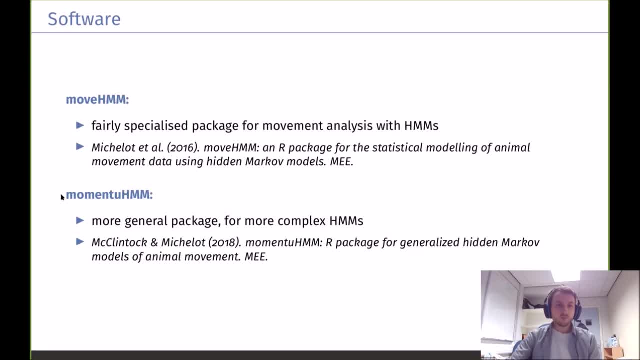 of extensions and stuff um, but momentum is quite a bit more general. momentum was developed as kind of an extension of move, hmm, and it includes anything you can think of. almost is in momentum, so something fancier you might need a momentum, and i'm going to talk about momentum today in the 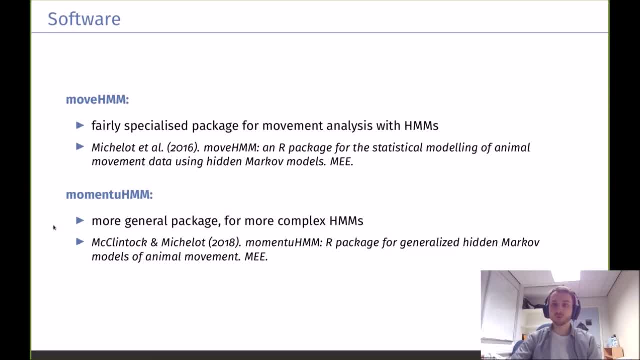 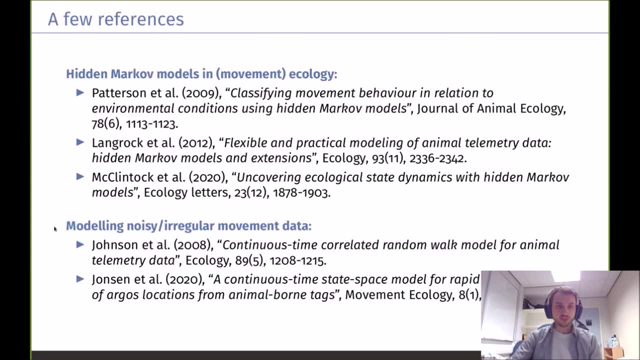 practical session, mostly because it has some integration with with packages that do filtering and prediction. okay, okay, so this is all i wanted to say. uh, this is the list of references. i'm not going to go through them right now, but just in case you want to read more about this, um, you can. 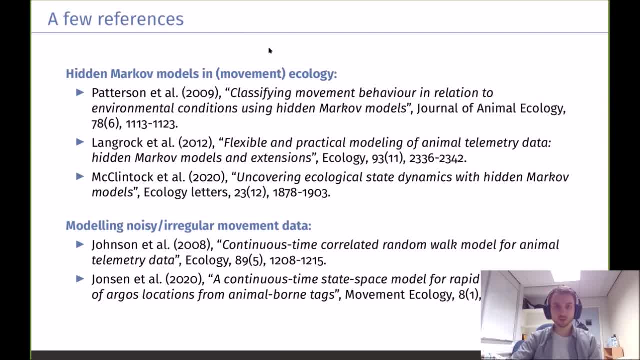 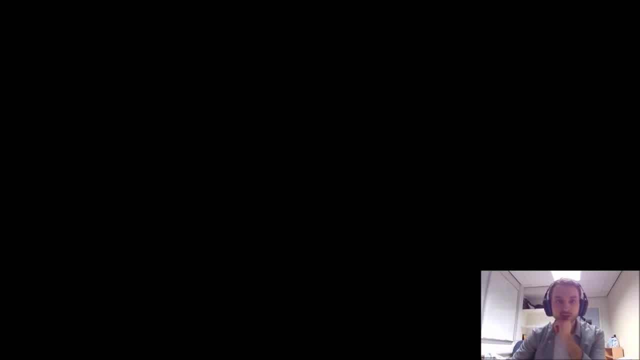 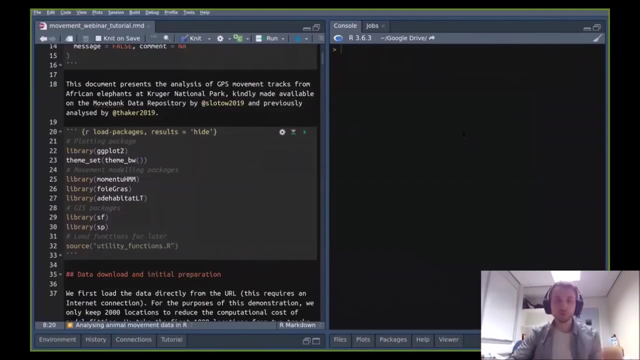 you can have a look, and these slides, by the way, are also on github, so you can. you can get them there, okay, great, so i'm going to stop sharing my slides and move on to the practical session, if that's okay with everyone. so i'm going to try to share our studio. okay, you should be able to see my r studio window. 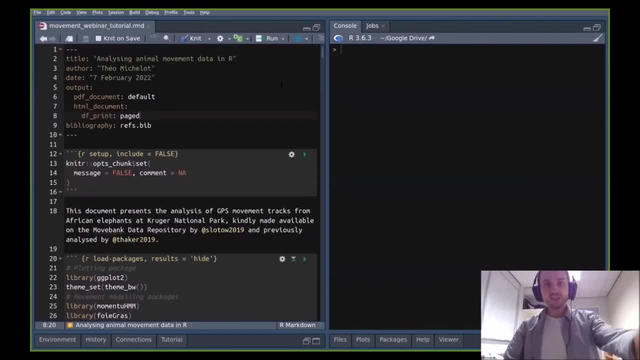 right now. yep, okay, good, so this code is on uh, the github repository. it's in several formats. there's the r markdown document, which is what i'm going to go through myself, like right now, but there's also, uh, just the output of this in pdf format or html format, and there's also just a. 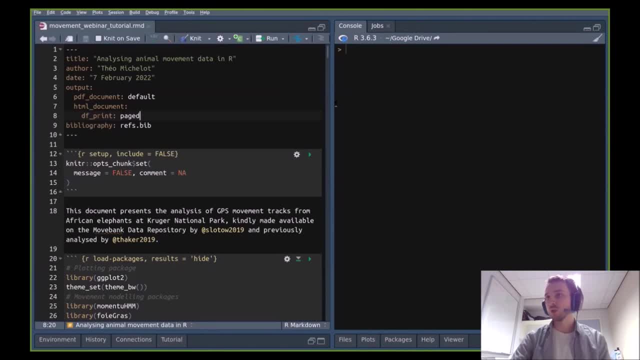 pure r script, in case you just want to um, to have the code without having all the all the text. that's in between. okay, i can give you a couple, maybe one minute, if if people are setting up their r studio- i'm not sure if people are going to be trying to execute stuff at the same time as me- 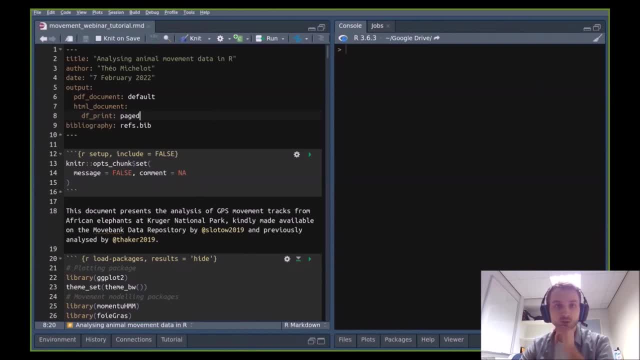 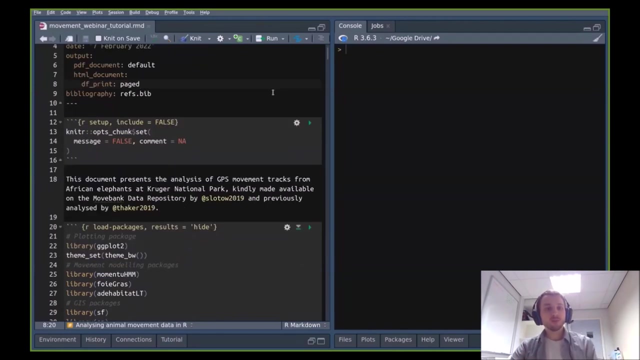 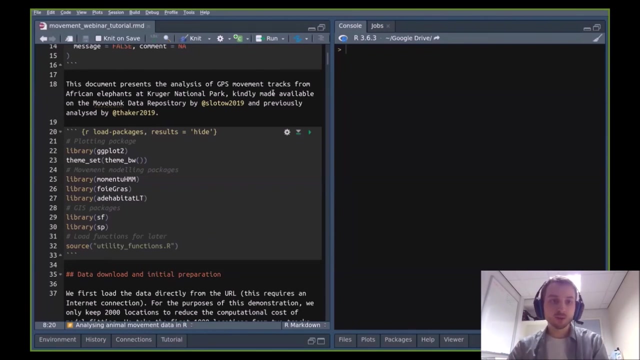 i guess i'll take this opportunity to maybe have it in the chat, okay? so, um, i'm gonna present a pretty what i think is kind of a pretty typical analysis of these data with with head bank of models. um, it's with a data set that i 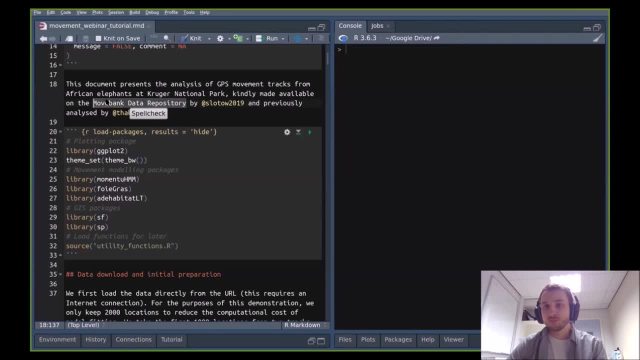 took from the movement data repository, which is kind of amazing. it's a data repository with, with, with open source and kind of free to use a data set, so i'm very grateful to the authors, the i think the data were provided by sloto and co-authors and i think it's 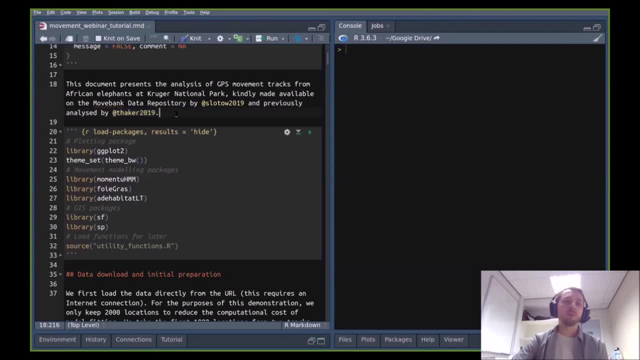 um, a data set that comes from a publication by thacker and co-authors, so thanks to them, it's data on african elephants. as a disclaimer, i don't really know anything about african elephants. i don't really know anything about any animals, so i'm just using this as a kind of example data set. 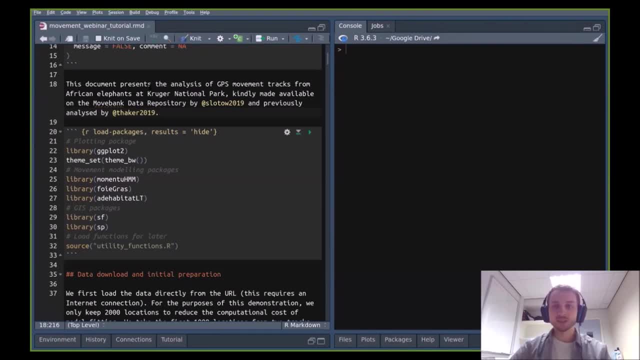 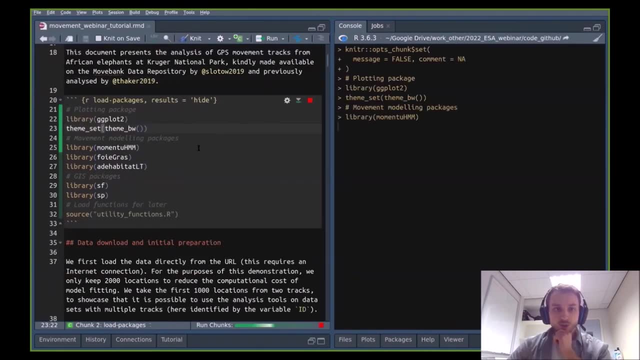 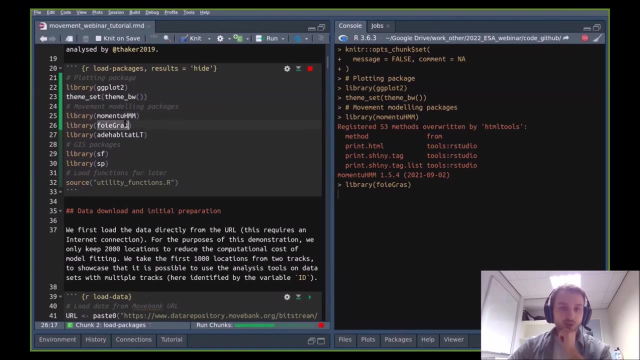 and i'm not really claiming any, any biological insights from this. i'm just showing this to you as a pretty stereotypical analysis using these models. okay, so i'm going to run first, i'm going to run this um to load the packages. so it loads things like momentum and, uh, foie gras that i'll. 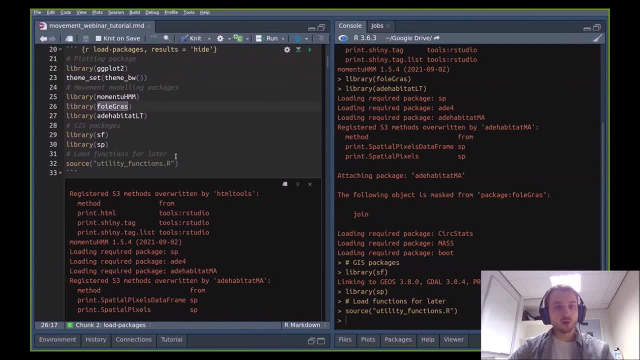 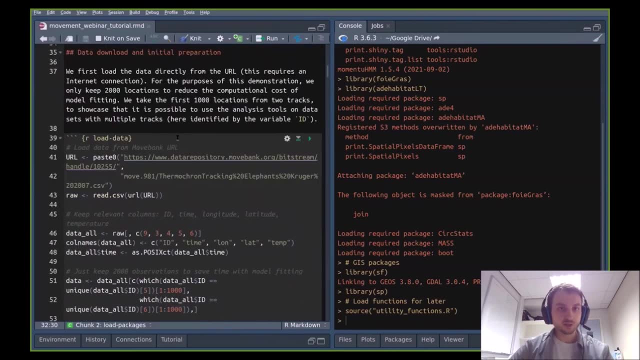 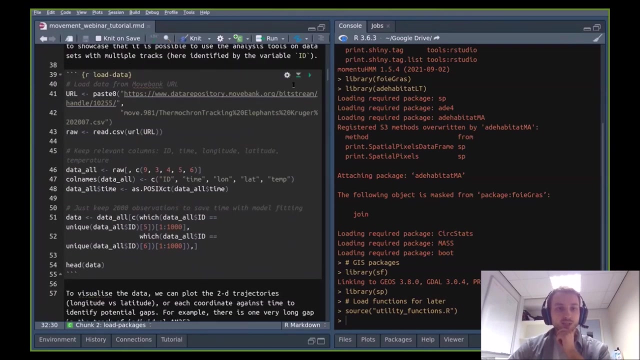 talk about a little bit later. um, it loads. this file has just actually just one function that i'm going to need, that i'm going to need later. okay, so now this is done, we can. uh, what this chunk of code here does is just load the the data from this url. so this is. 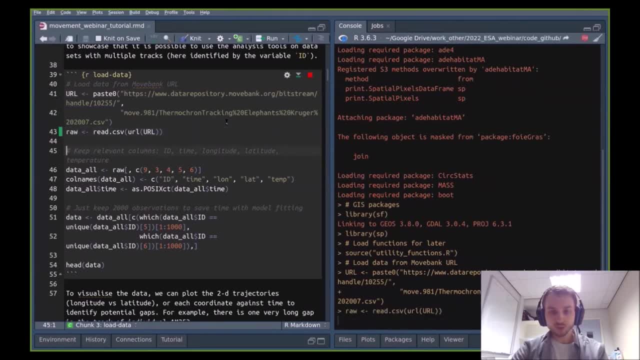 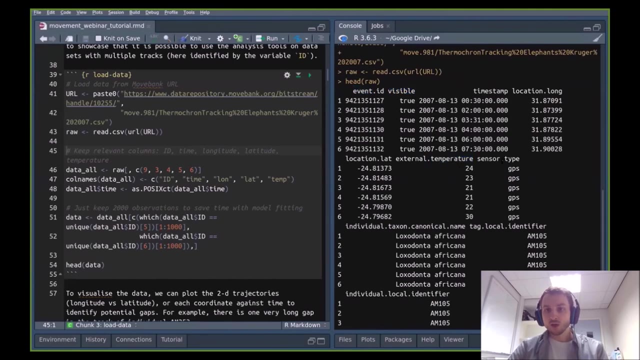 the url of the data on on movebank you can load. it takes a little while you also you need a data internet connection to do this. and then i don't know if you've ever seen a movebank data set, but they have kind of all these those uh columns, uh, we don't need all of these for our purposes. so 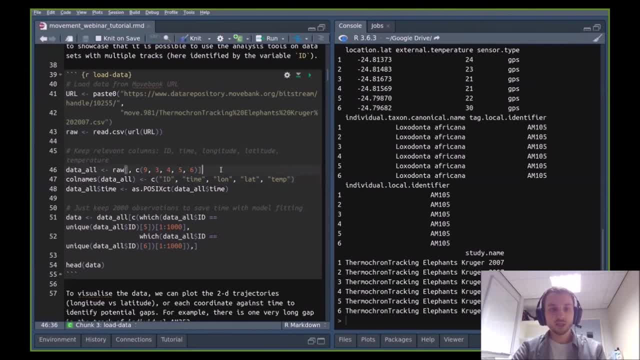 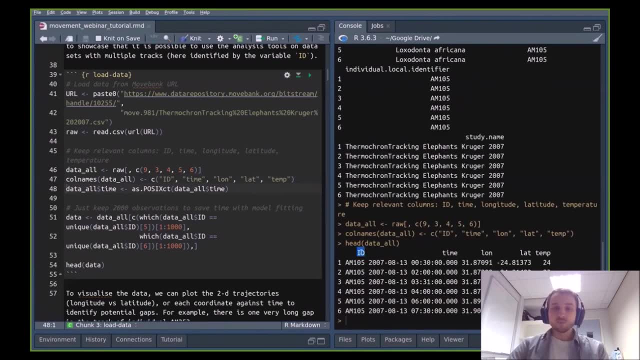 what i'm doing next is is just to to sub some, to subset- sorry to uh a few um variables that we want to keep, and so this is the data set that i get, where id is the individual id of the elephant, because there are several elephants in this data set. 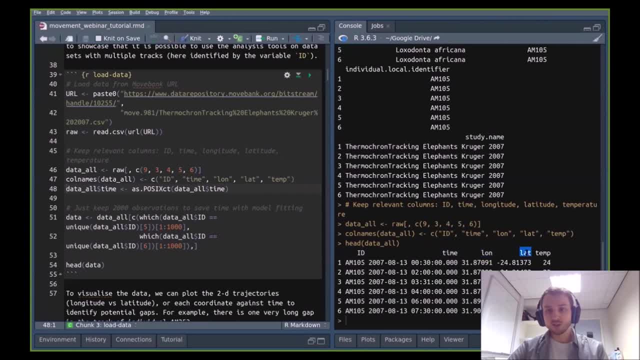 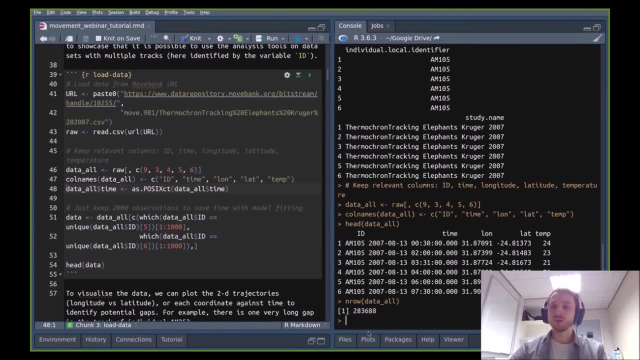 time is the time of the observation: long longitude, latitude and temperature. okay, and this is a big data set. it has, i think, yeah, 200, almost 300 000 observations, so it would take forever to well, i shouldn't undersell the computational speed of of the my software, but it would take a while to fit models on on this especially kind of complex. 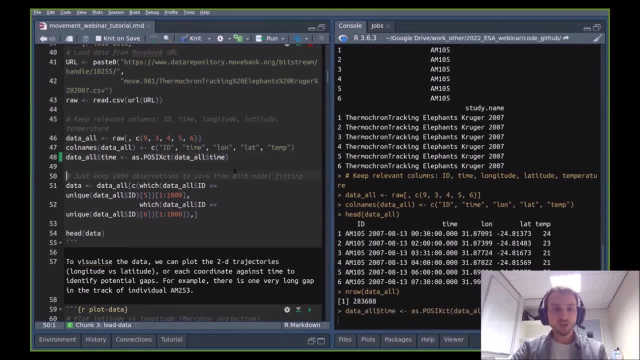 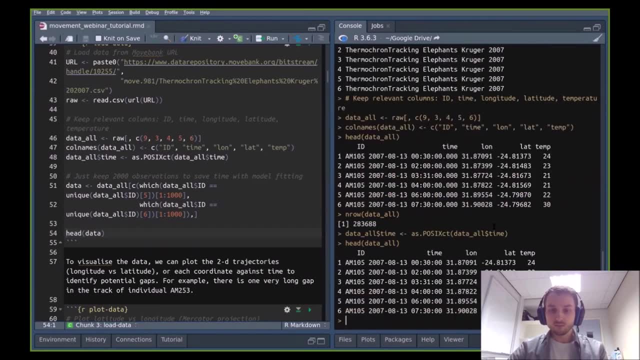 models. so i'm just going to take a subset of the data for illustrative purposes, and so this is what this is doing. so let's see, this is the same thing, but now we just have data from two individuals. oh oops, this is what i wanted to show. 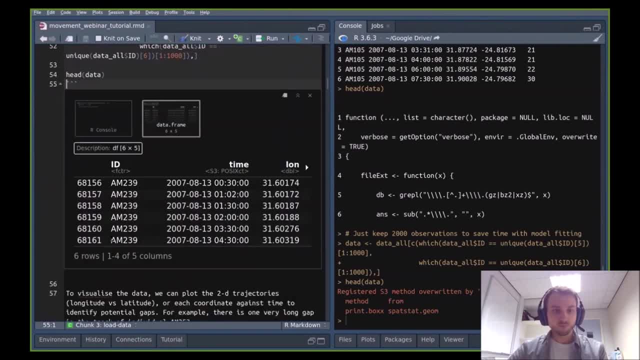 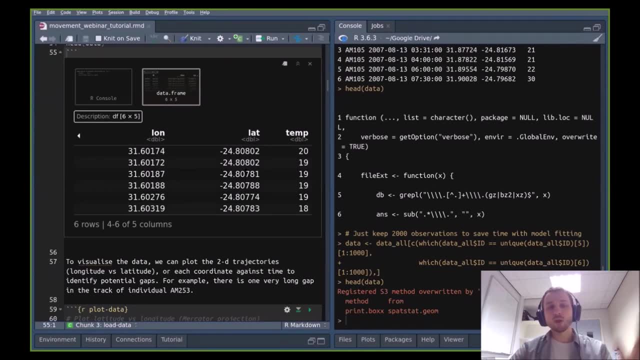 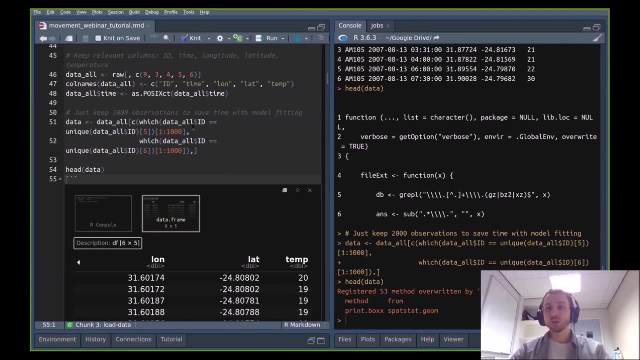 what happened? yeah, here it is. so we have id time, longitude, latitude, temperature for two individuals and we have 1000 observations, uh, of these two individuals. the reason i'm still taking observations from two individuals rather than just taking one track is that i want to illustrate that we can also use these methods on. 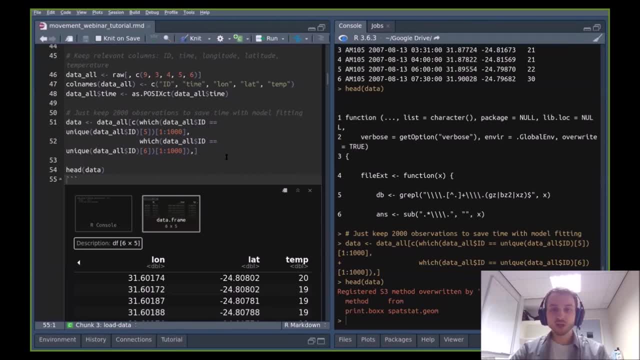 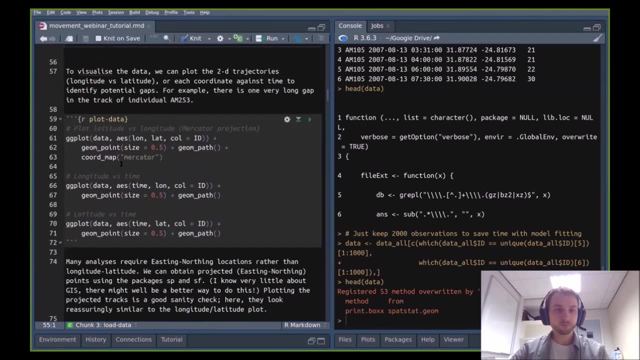 on several, several tracks. okay, there's nothing preventing you from doing that. all you need is a column in your data set that's called id and that identifies, uh, the the tracks. okay, okay, so we can visualize, uh, we can visualize the data. so if we're going to do this, we're going to. 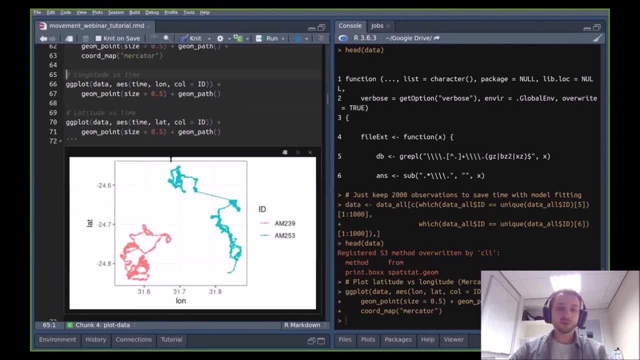 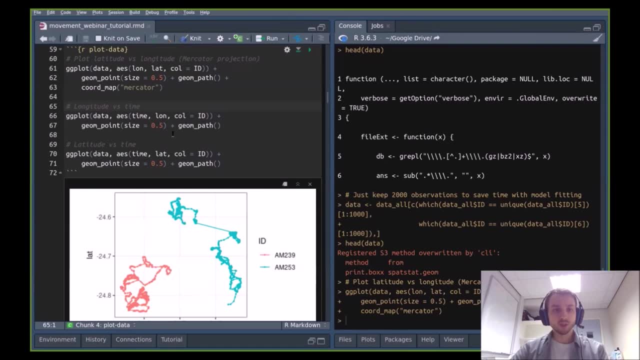 plot longitude against latitude. this is what it looks like. so here it's. the two different tracks are in two different colors. you can see that there's kind of a gap here, and we'll talk about this in a little bit. we can also plot: um, this is just longitude against time, and here you can. 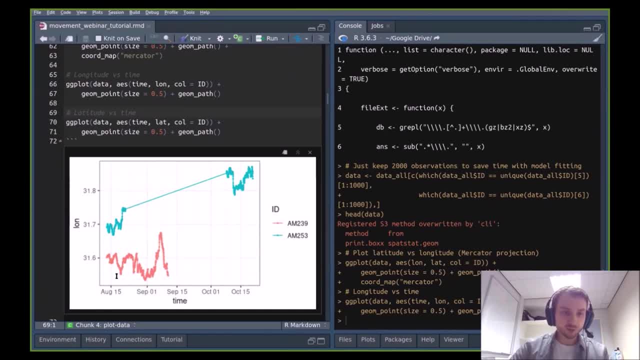 see the gap very clearly. so this, the, the red track here, covers maybe a month or something, and the other track ran, uh, so that i'm guessing that the, the tag, probably ran for a couple of weeks and then stopped working for, or i don't know, it was turned off or whatever for, um, maybe a couple of months, and then right again. 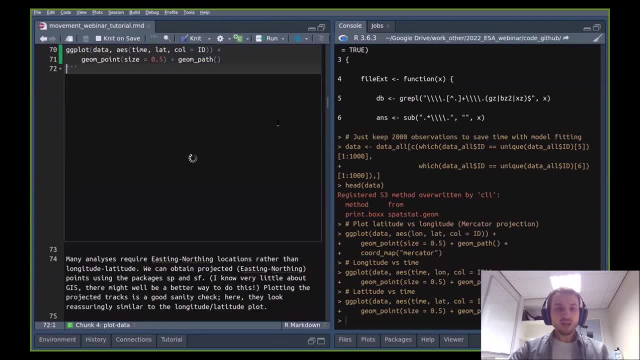 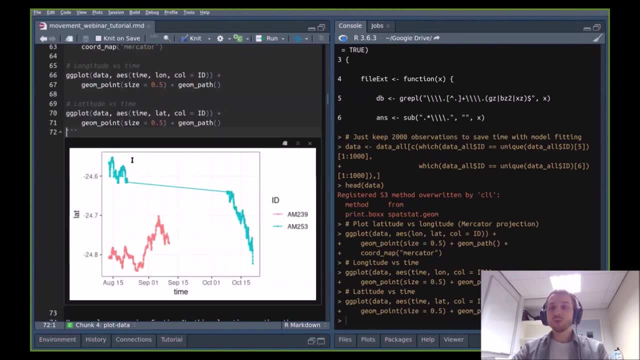 for for a couple of weeks. so there's this big gap and we can also- we can also see um latitude against time and that's what it looks like. okay, so these are gps data. i'm not i'm going to assume no measurement error, so i'm not going to worry about measurement error. what i am going 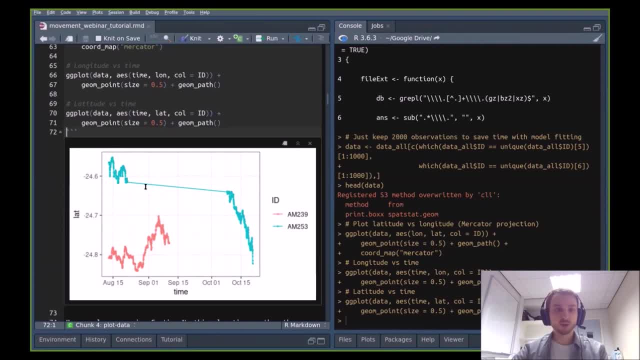 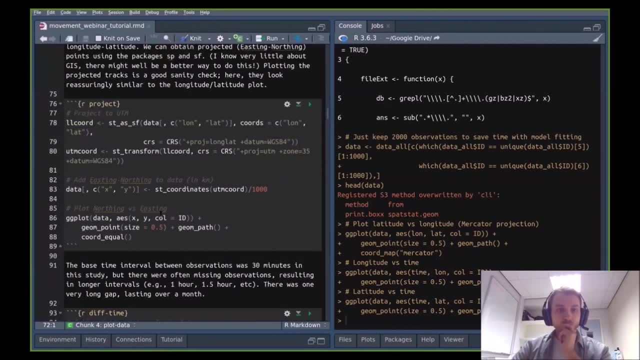 to worry about is these big gaps. at some point we'll have to do something about these, okay. okay, this, um, this chunk of code here, um, i'm using to project the location. so right now i have longitude, latitude locations and in many cases, we're more interested in having easting and northing projected locations. 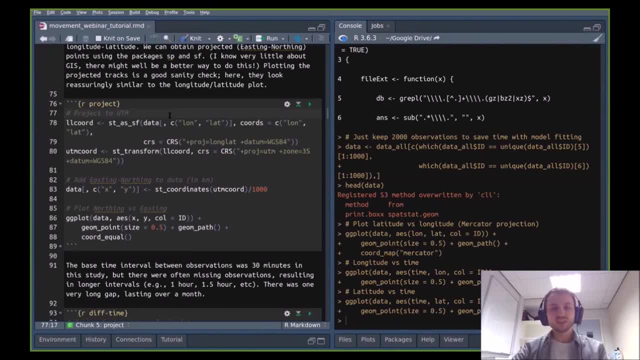 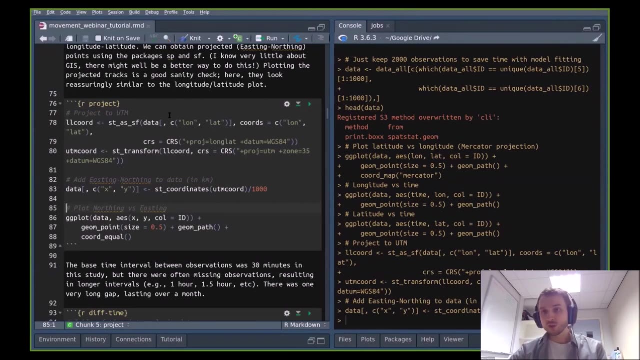 okay, um, and this is because longitude, latitude locations are a little bit strange. they're not, you know, they're. they're both angles, and so they're not very convenient often for for modeling. uh, i don't know very much about gis either, so here this is the code i'm using. i'm not sure that this is the best way to do it, and 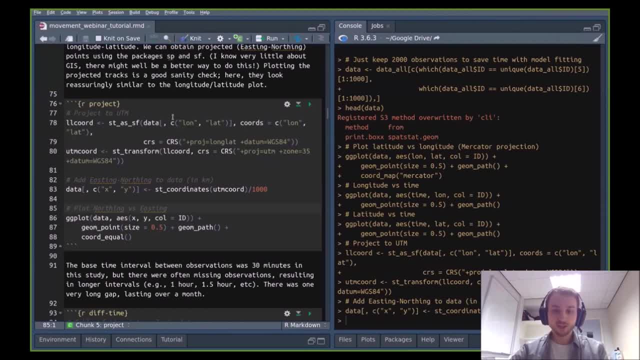 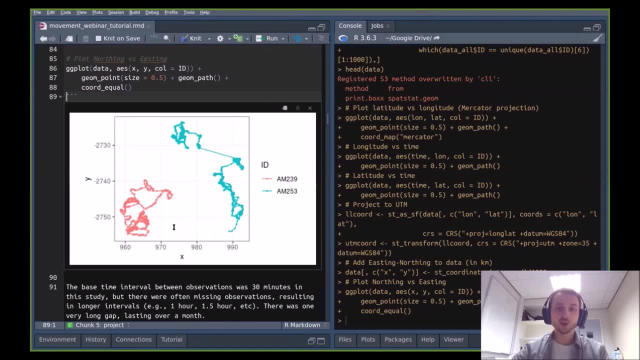 you. you guys might actually find, you know, problems in this code. i hope not, but i think it works. and the reason i think it works is that when i plot the projected locations, which is what i'm showing here, it looks pretty close to the, to the original ones, which is what i would expect here, because 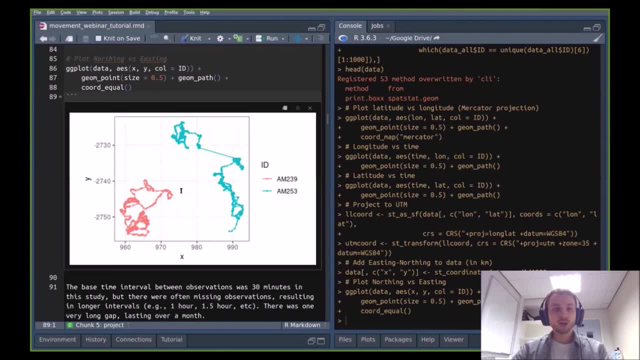 this is a data set from the kruger national national park, i think in south africa, which isn't too far from the equator. if you had data like i was talking about- um, you know, elephant sales or or data in like antarctica or something- when you project your locations, your projected tracks are. 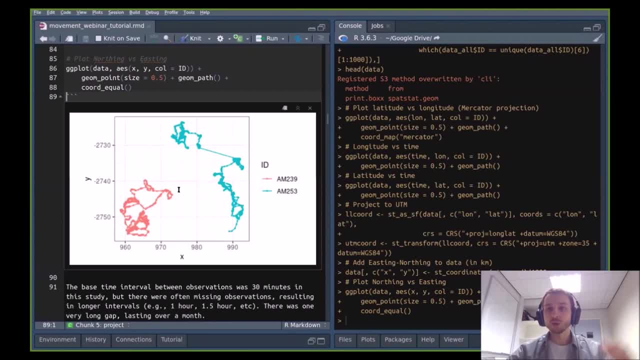 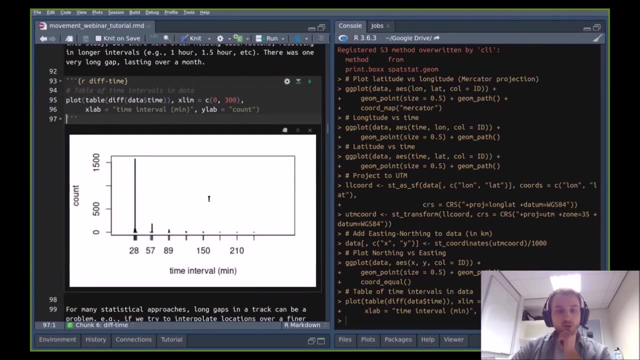 going to look nothing like your longitude latitude tracks, because the further you go, you know, the closer you go to the poles, the more distorted the projection will make them look. but anyway, this is the projected tracks i have. i'm pretty happy with them, okay, so let's talk about the main. 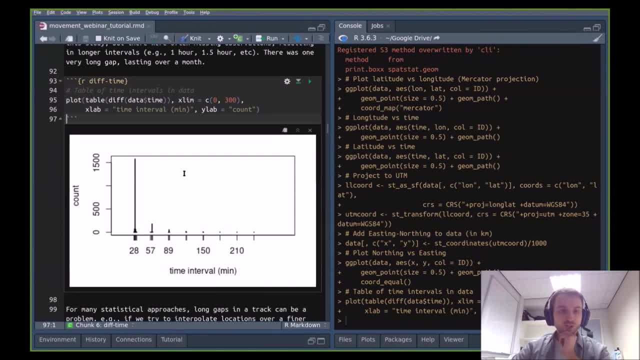 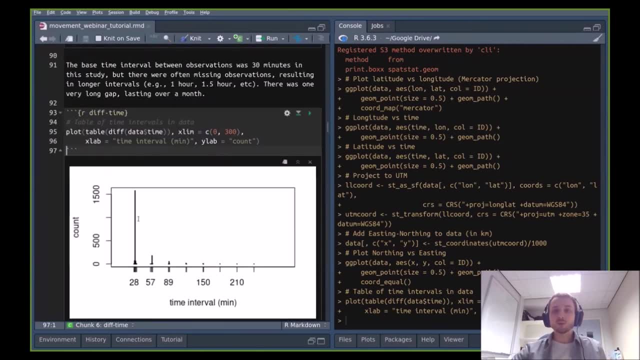 problem we have with this data set before we can apply hidden markov models, which is that we have- and they're not totally irregular- the the base kind of frequency for observations was 30 minutes. one observation every 30 minutes in this, in this data set, but there are quite a few missing, uh. 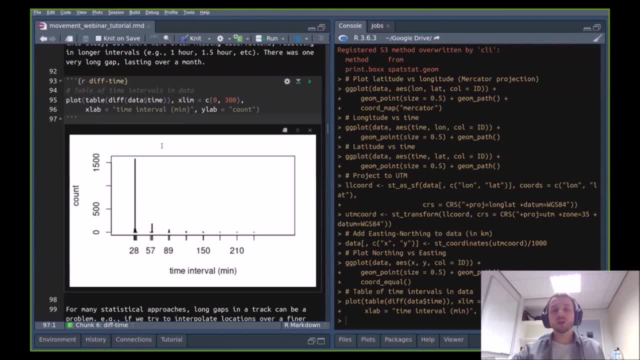 missing uh locations, and each time there's a missing location, instead of having a 30 minute interval, you have a one hour interval, right? if there's two missing locations, you have a one and a half hour interval, etc. and so what i'm showing here is the count for different. 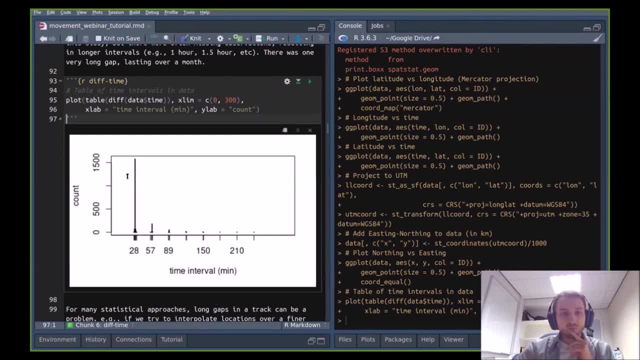 uh, time intervals, and so you can see that most of them are around 30 over here. so that's good, but you have a few around an hour. so these are when there was just one missing location. you have a few around one hour, one hour and a half, etc. and here i'm. 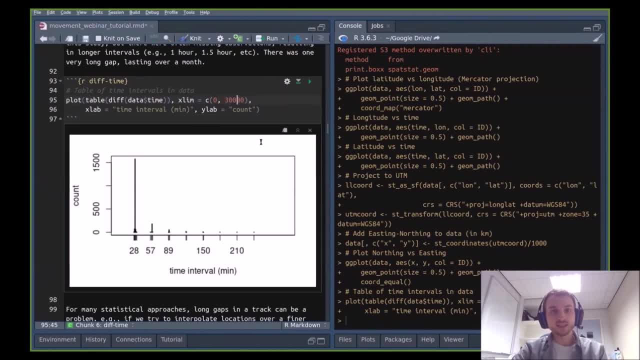 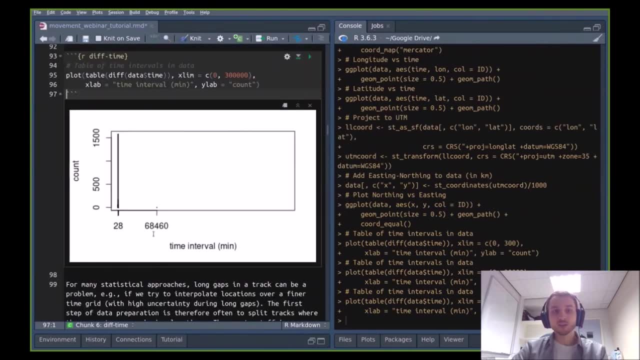 truncating the. i'm truncating the x-axis, but if i don't how, i don't know how big it needs to be. oh yeah, this is. the maximum value is 68 000 minutes. so this is like the very, very long, long gap um that we saw in the um. the second: 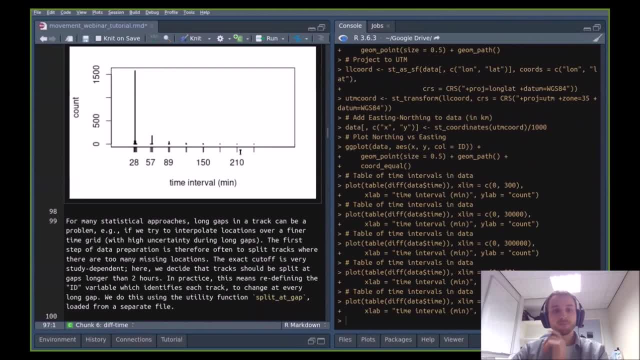 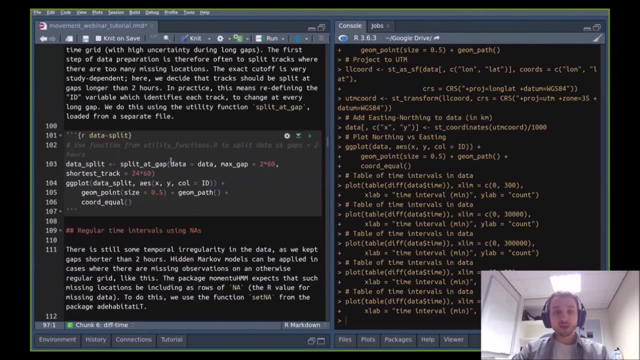 oops, the second elephant's track. okay, so we want to do something about these and, uh, the first stage, i think, uh, that we often want to to apply before doing things like trying to trying to predict locations over the gap or something like like i was talking about with. 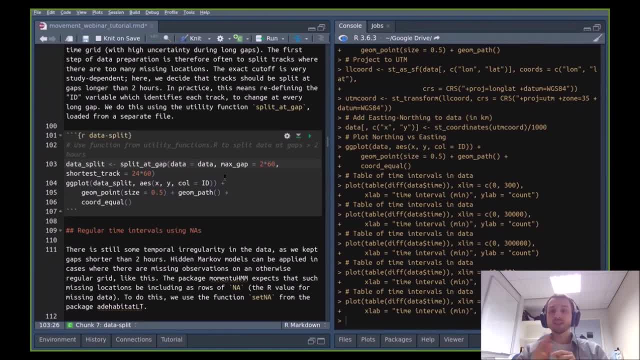 state space models. we might just want to split tracks where there's very long gaps because you don't really want to fill in. you know, if there's a gap of two months, you don't want to months. there's no point in doing that because you're not going to be able to do it with any. 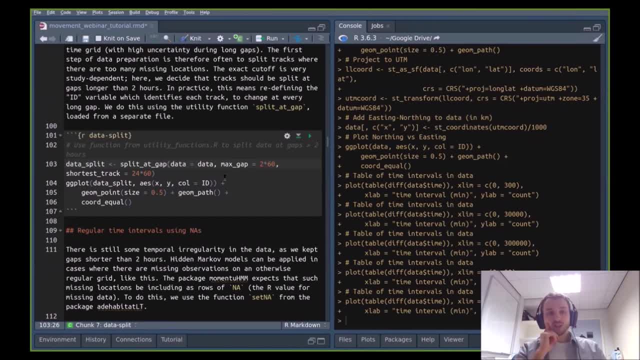 precision. so instead, what we often do first is to split the track, so that then you you say, well, before that two two month gap, it's one track, and after that two month gap, it's another, it's another track. they come from the same animal and you can keep that information if it's useful. but you can. 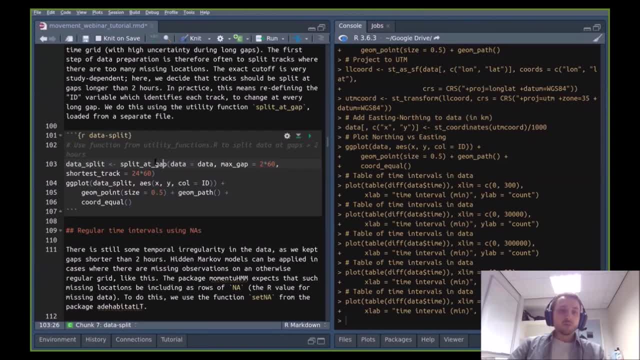 just treat them as two different tracks. okay, and so here i'm using a function that's loaded from from a different data, a different file called utility functions that are that's also on the github, called splitted gap, and it takes the data set and the maximum, the maximum gap as 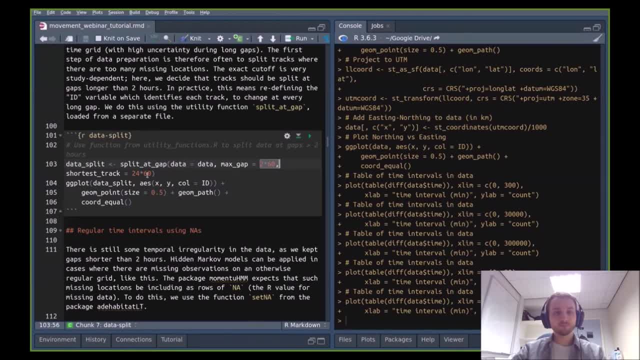 input and the maximum gap is in minutes. so here i'm saying two minutes, and here i'm also saying that if there's, if this gives rise to two tracks that are shorter than 24 hours, you can remove them so that it doesn't like, you know, just like keep a single observation as a track, or something. 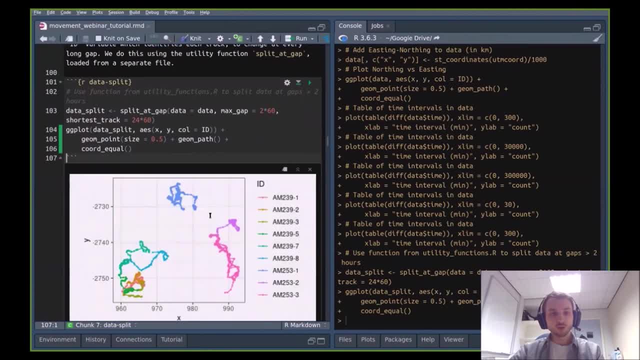 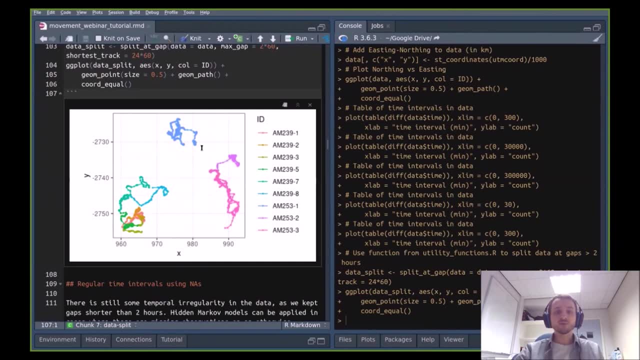 okay, so if i apply this and then, uh, plus the, the split data set, this is what i find. and so here you see what. what it did. it removed the long gaps and instead just defined new tracks, and i'm thinking in this case, it ended up defining nine new tracks by removing gaps, and so we know. 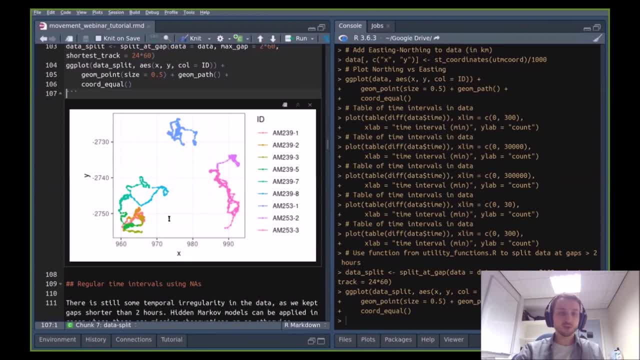 that these three here still come from, you know, the same individual. these, like six or whatever, came from the same individual, but we're just going to treat them as separate tracks, okay. so it just means i replaced the id column by something that identifies the their, their separate tracks, and so now, now we've removed kind of the worst of the long gaps, okay. 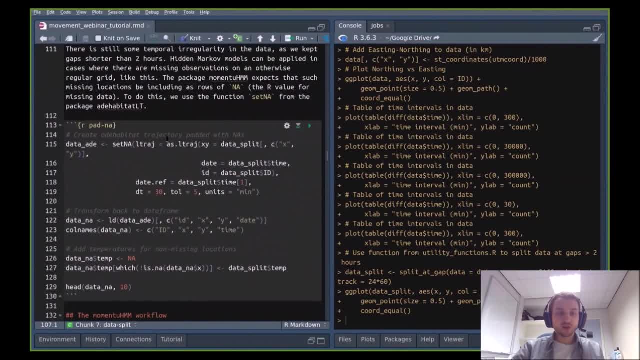 we still have some irregularity because we we still had, um, we had some, you know, gaps that were just like an hour and a half or or an hour or something, and i didn't uh split tracks as the uh, when it was like, when it was this short, i only split. 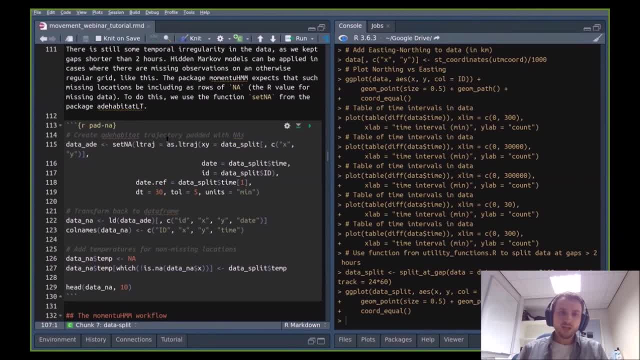 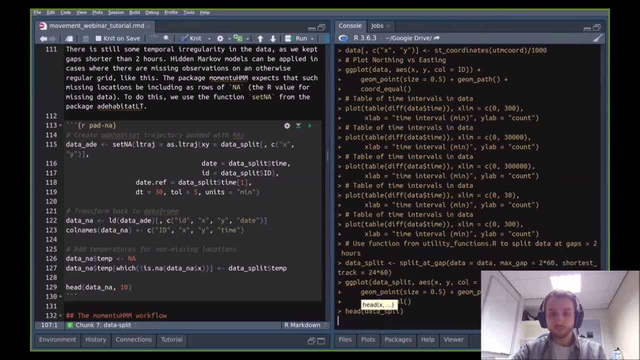 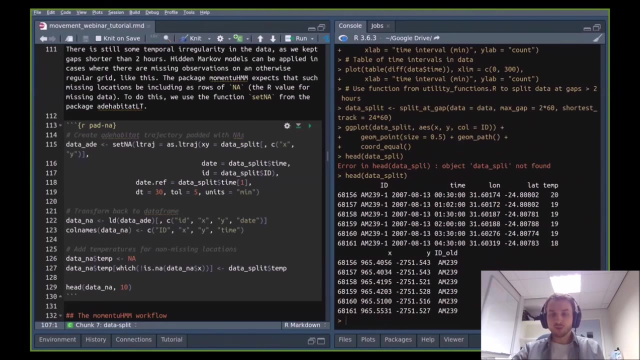 the tracks when it was longer than than two hours, and one thing we can do about this. well, i can, i can show you um oops. so, for example, here, if we look at the data, the first observation was a half past midnight, the second at one o'clock. so half an hour here. half an hour again with uh. here half an hour again. 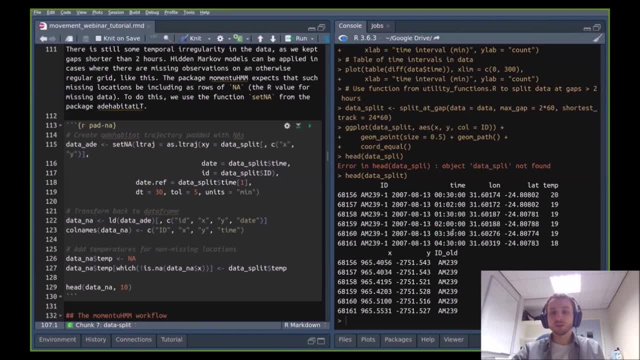 but here there's an hour and 30 minutes of a gap right here, right, and then an hour. so these are still not regular. so this is still going to be a problem to get step lengths and turning angles, uh, for hidden markov model. so one thing that we can do is to include rows of nas. so here, for example, there's two missing. 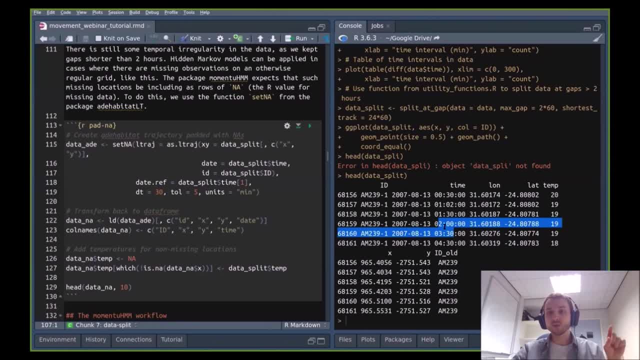 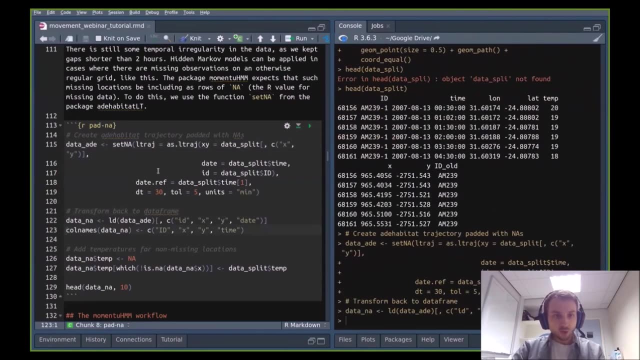 locations between these two. so we can just pad this data set with rows where we put missing values, nas and r for longitude and latitude, and here i'm using a function, set na, from the ad habitat package that does just that. okay, so, so this is. i'm going to show it in the console. 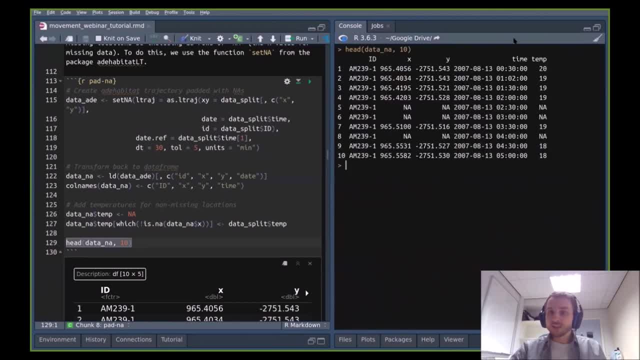 and i'm going to show you how to do it. so this is the data set i have now. i have still id, x, y, time and temperature. it's the same columns, but now i have rows of nas where they were missing- uh, missing locations- and you can see that these correspond to the times where 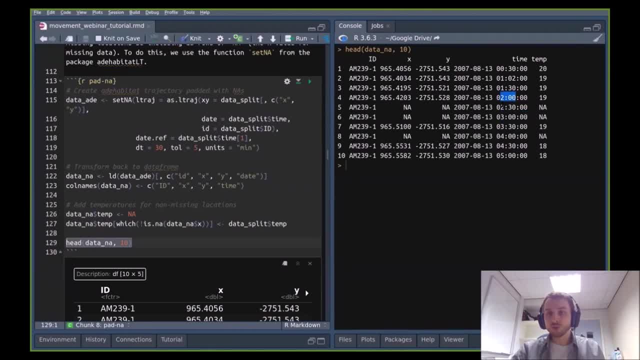 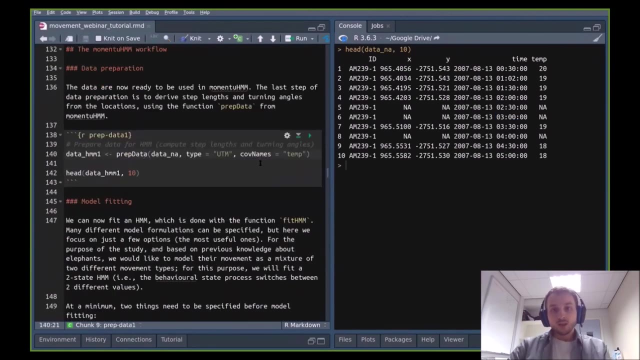 we didn't have a location, okay, so now we have two, two o'clock, two thirty, three, three thirty. these are now at regular half an hour time intervals, okay, and so now we can directly input this into momentum to fit an html, okay. so, uh, first step of the analysis. if you remember the 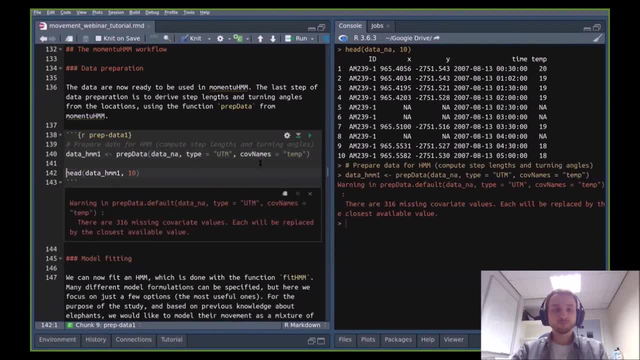 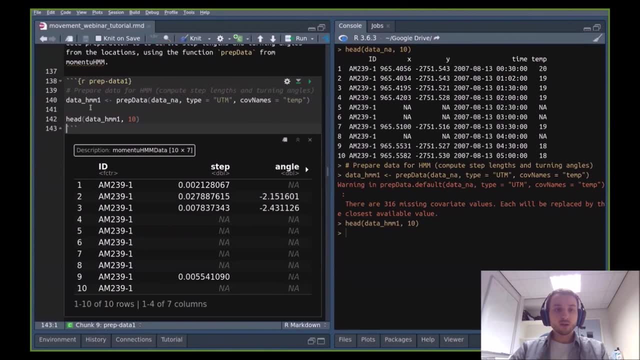 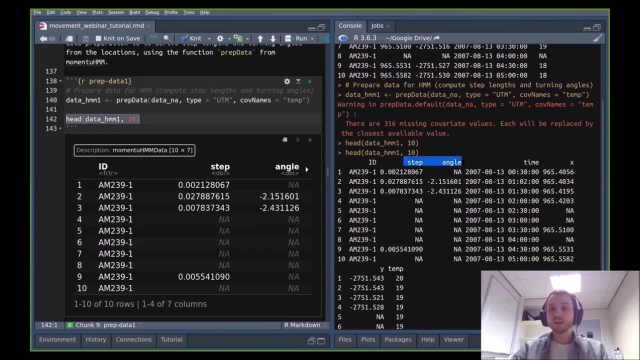 workflow i was presenting is to get step lengths and turning angles. so this is what this function- here- prep data- does, and so here, if i uh print my data set, it's the same variable as before, except it also has a column for step and a column for turning angle. and then these: 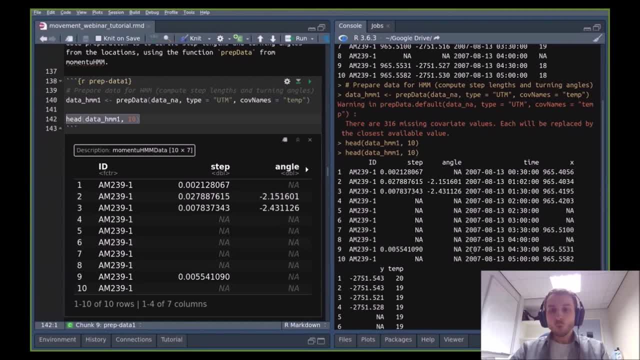 are the variables that we're going to model in the html. one thing i want to point out, in case any of you are confused about it, is that you'll see that there's more missing values in the step lengths and turning angles, columns than there were in the locations, and the reason for 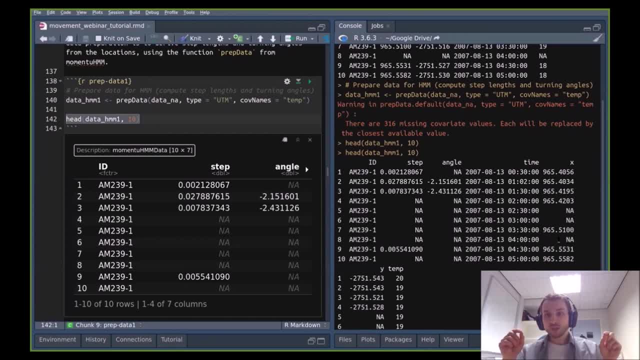 that is, that to get one step length, you need two locations and to get one turning angle, you need three locations. and so when you have one missing location, you get two missing step lengths, you get three missing turning angles. okay, so this is why you can, in principle, you can- include: 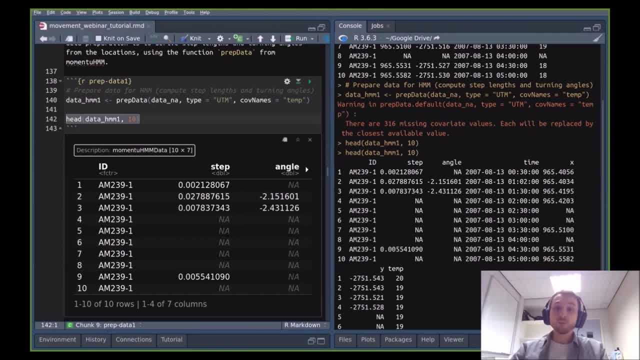 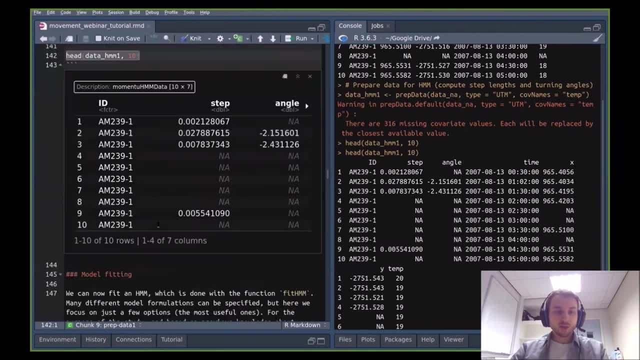 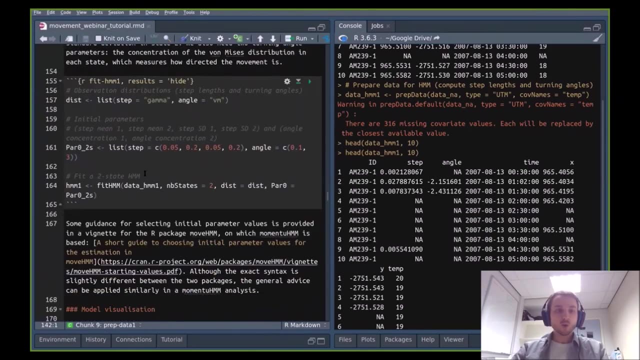 these missing locations and then fit the the html. but it can be a problem: if you have many of them, you might have many missing steps and angles. okay, okay, so this was preparing the data. now we can go on to fit a model. so there's two things we need to specify. uh, we'll be using the function, that's. 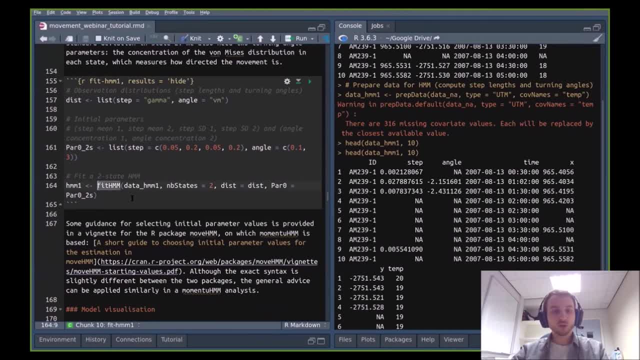 called fit html. fit html is the most kind of central function of momentum. it's the function that fits a model and it takes the data set- this data set that i was showing as input. another input is the number of states. so here i'm just going to fit a two-state model, so i'm 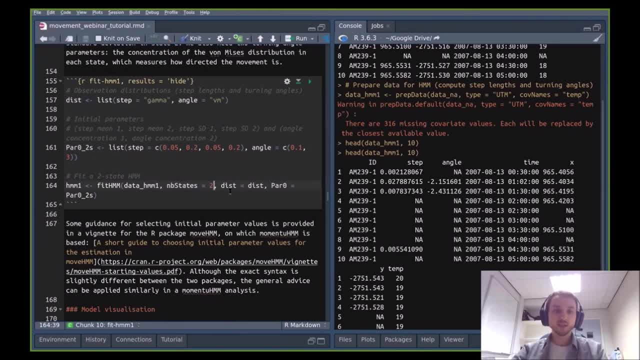 assuming that the movement arises from just two movement states. and then there's two other things we need to specify: this dist argument and this part zero argument. this is, uh, specifies the distributions that we use for the step lengths and turning angles, and here, in this case, so i'm 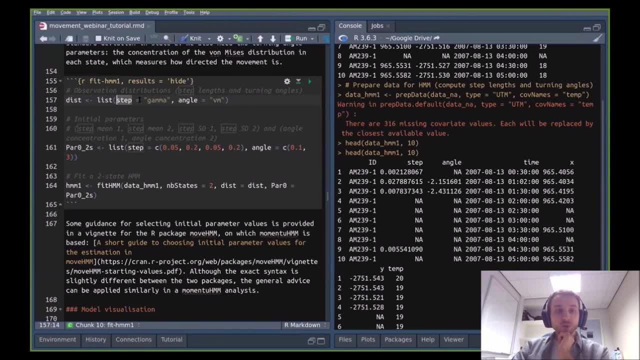 defining as a list, with an element for each variable. and i'm saying: the step lengths are gamma distributed, the turning angles are the step lengths, and the turning angles are the step lengths and the turning angles are von Mises distributed. okay, this is what this means, and then this par: 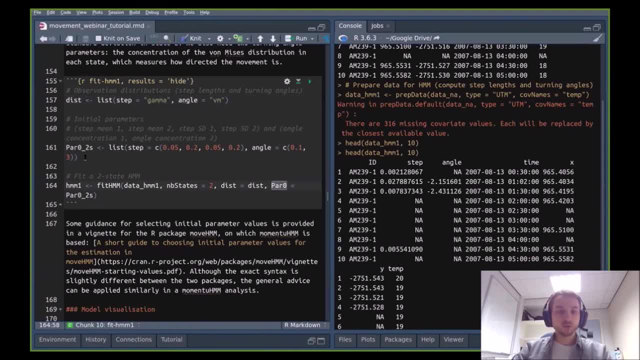 zero argument takes the initial parameter values um that we want to pass to the numerical optimizer for model fitting, and so we need to pass a list of initial parameters that look something like this, and here, in the comment above, i've put the interpretation of these six initial parameters: 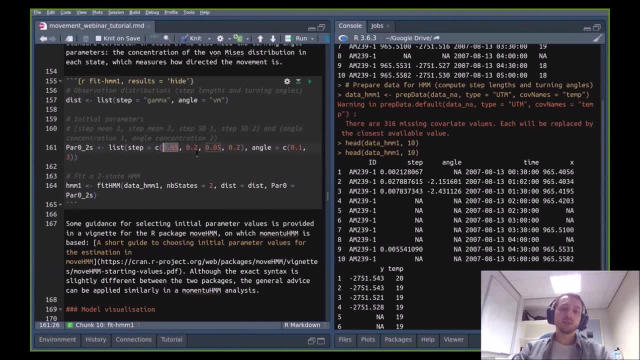 that we provide. this is the mean step length in state one, the mean step length in state two, um. standard deviation of step length in state one, standard deviation of step length in state two. and these are concentration parameters. so measuring how, how peaky the uh, the turning angle distribution. 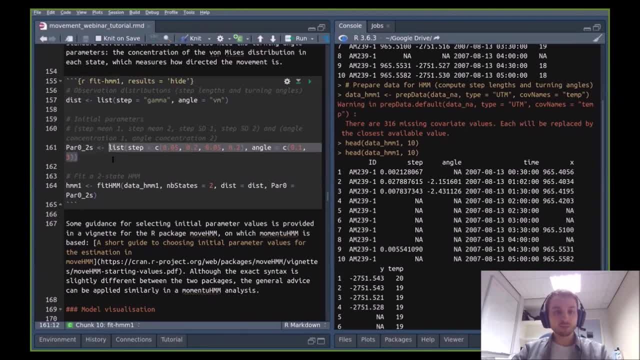 is okay, and i'm not gonna have time to describe how i came up with these values, but i point you to that vignette that i mentioned. i think there's also a link to that vignette right here under the this chunk, if you're curious to know how how i came up with these values. okay, so i'm just going to run. 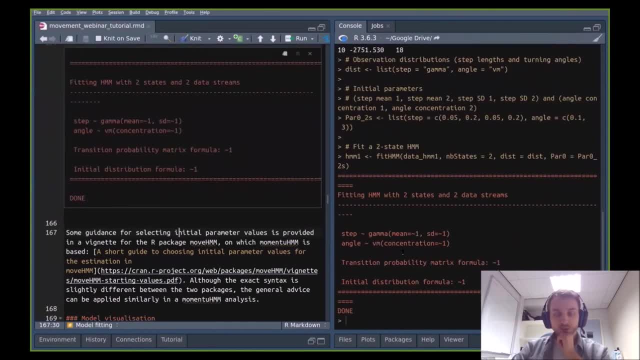 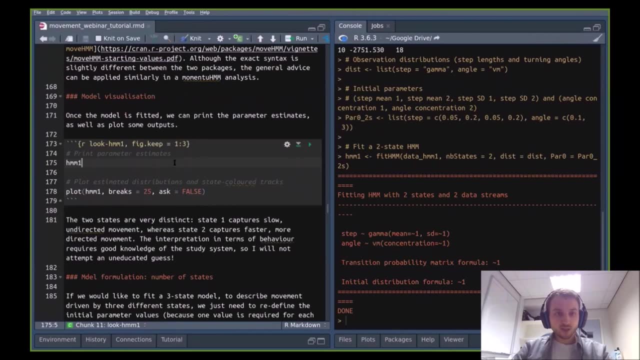 this chunk and it's going to take, you know, a few seconds to fit the model. now it's fitting the hm, it's estimating all those parameters and once we have this fitted, uh, this fitted model, we can, uh, we can print it. so if we print it, it, uh, it gives us the parameter estimates for all those, all those. 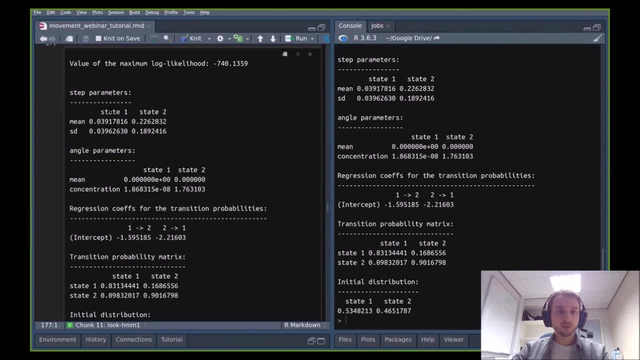 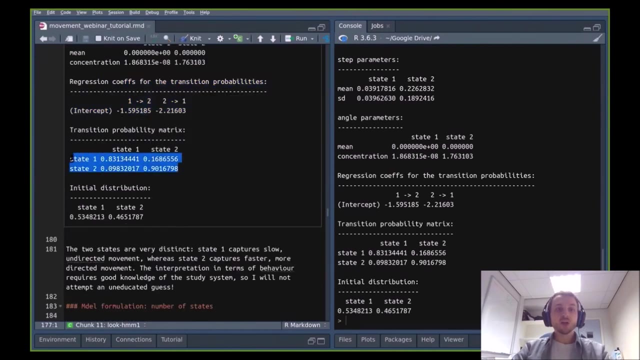 parameters. so these are parameters of the step length, uh variable. so this is. in state one, we have a mean and a standard deviation. in state two, we have a mean and standard deviation as well. these are parameters of the turning angle distributions. you don't need to worry about these right now. and these are. this is a transition. 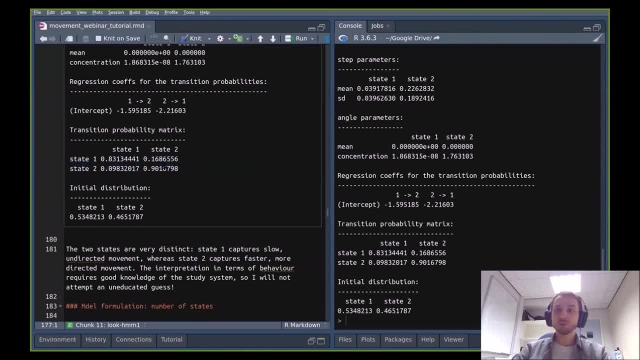 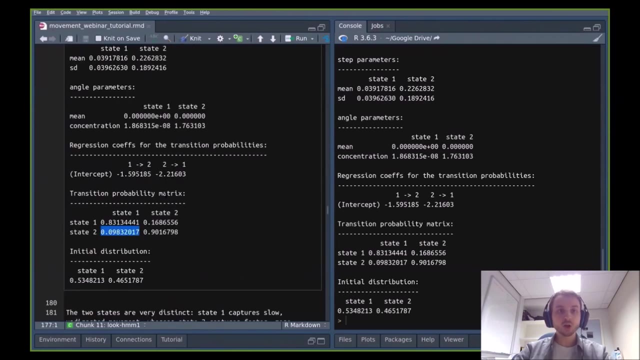 probability matrix, so showing us the probability of transitions between our two states. so this is the transition probability from state one to state two: about 17 in this case. and this is the probability of transition from state two to state one: it's about 10 in this case. okay, so these are. 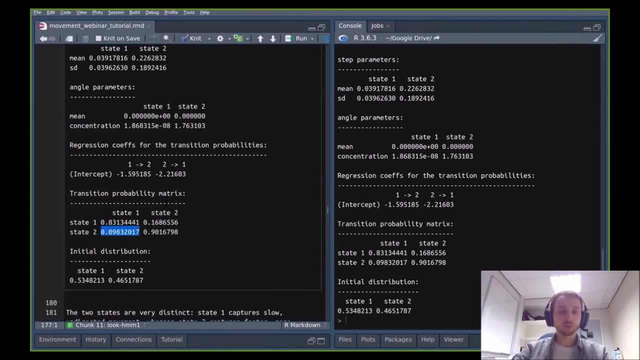 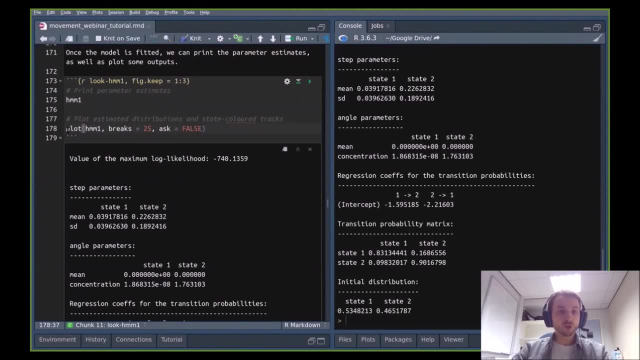 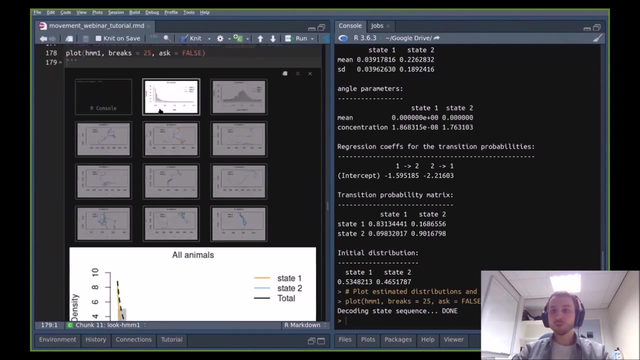 all the parameters that i mentioned in my slides, all the parameters that we want to estimate okay. so it's a little bit difficult to interpret these in and of themselves. one thing you can do is to use just the plot function on the hm object, and if you do that it's going to return a bunch of different plots that help you interpret. 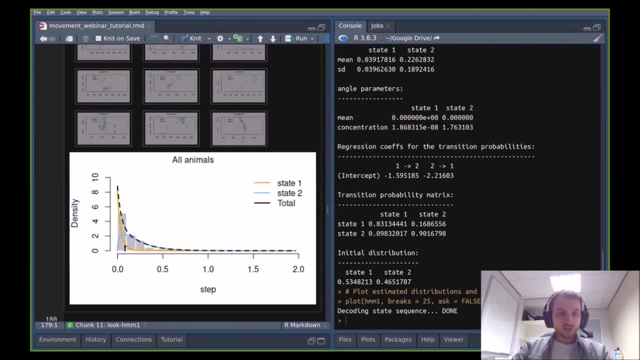 the model. so the first one: this shows a histogram of the step, the observed step length, and then the two colored lines are the densities of step length as the estimated distribution of step length in the two states. so we see in state one it's a distribution that's going to capture mostly kind of 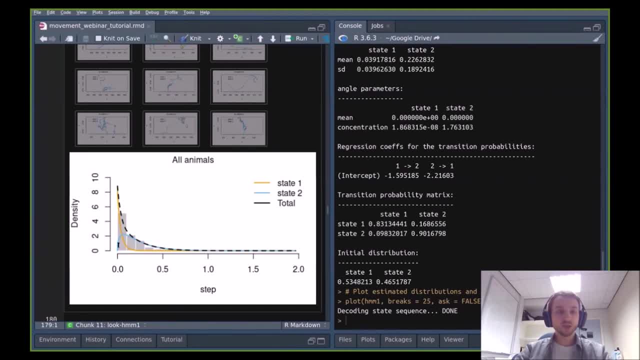 short steps because most of the probability is kind of close to zero and state two is going to capture more kind of the longer steps because it it ranges from zero to i don't know one kilometer or something. it's going to kind of capture those longer steps. so state two is going to be faster. 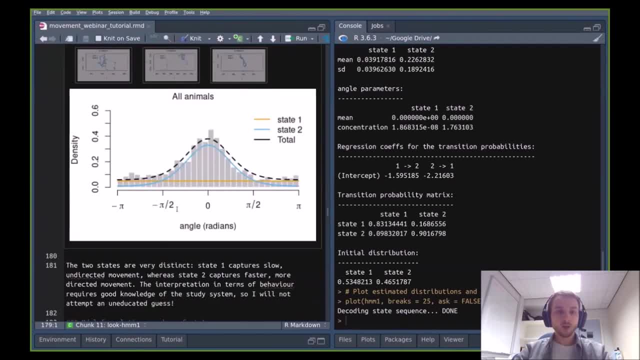 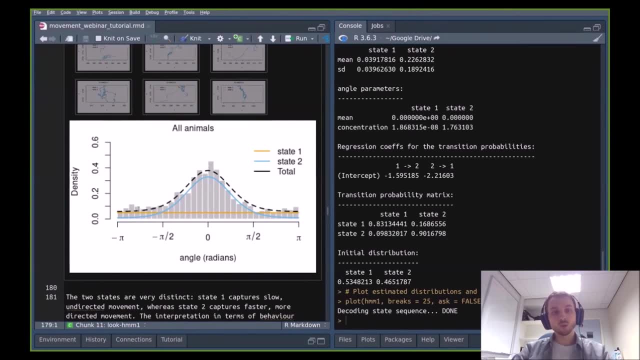 movement. state one is going to be slower movement. same with turning angles. in gray is the histogram of turning angles in the data and then blue it's the well. orange is the probability distribution of turning angles that's estimated for state one. so in this case it's very flat, so very undirected. 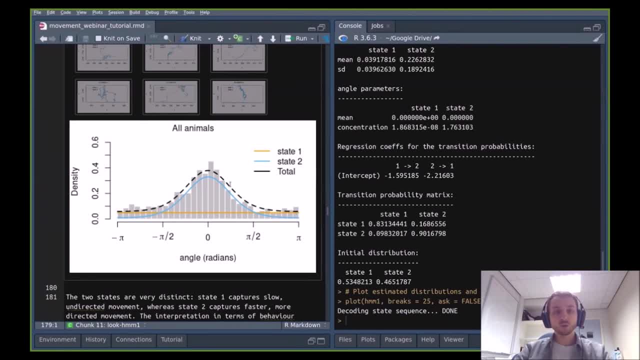 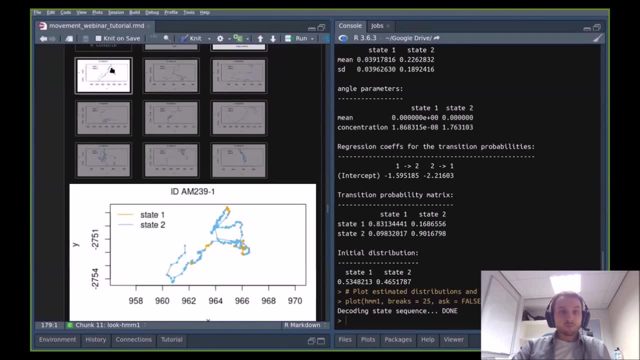 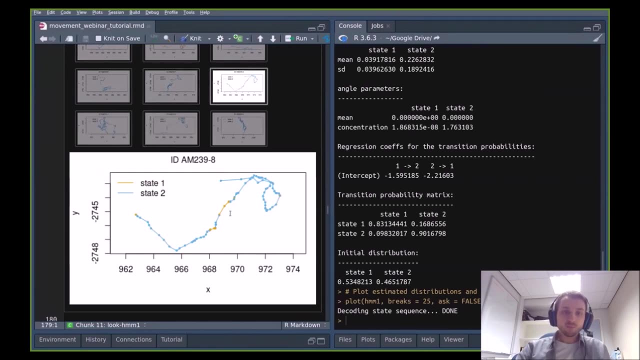 movement and in blue it's um, it's a little bit more peaky, so a bit more, a little bit more directed, and you can also get um. you can also get tracks. so these are just the nine tracks that i had in my data set, colored by the, the estimated, the most likely state sequence. okay, so here, for example, i: 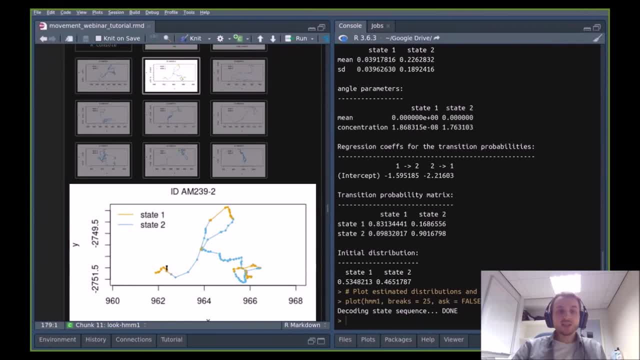 don't know if i can find an interesting one. i mean any of them really. you see that, as i was saying when i was going over the distributions, slower movement is captured by the orange state, the first state, and faster movement is captured by the blue state. okay, so with these you can already tell quite a bit, and 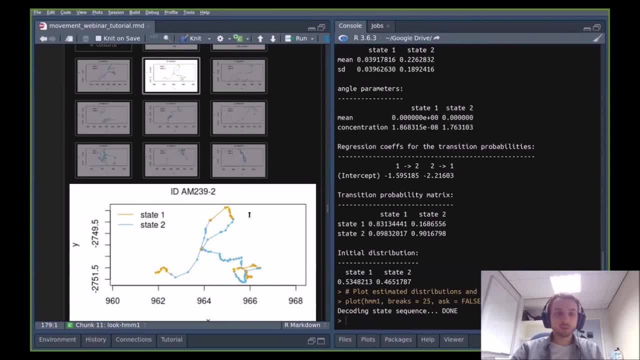 and probably you know, if i knew something about elephants, i could probably already say something about you know, the blue state is maybe transit between areas of interest and the orange state is a mixture of, like i don't know, resting and foraging or something. okay, okay, um. 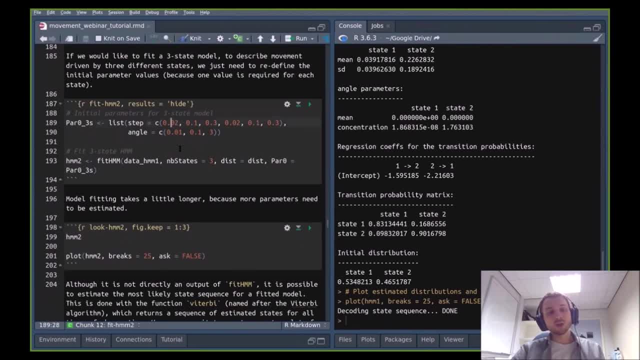 so one thing we can try to play around with is the number of states. so let's say we want three states. actually, we think that elephants follow three different stereotypical behavioral states and we want to try to capture these in our model. so the only thing we need to redefine is, uh, the 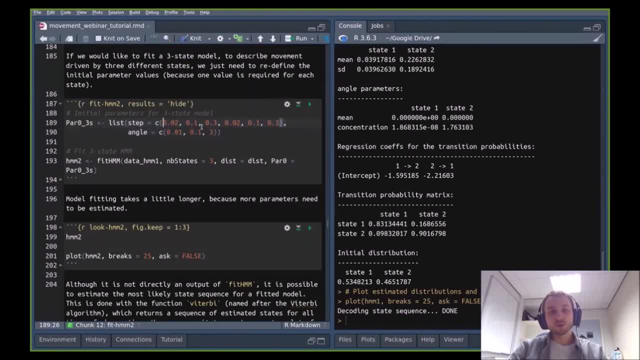 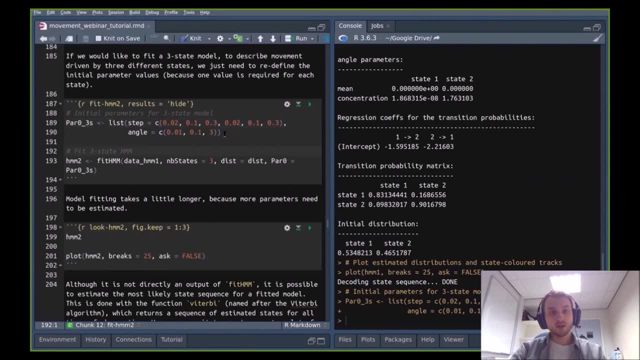 initial parameters, because now we need three parameters of each, because there's three different states and one parameter for each state. so again, i don't really have time to explain how i found these, but I'm redefining these and now I'm fitting the three-state model. 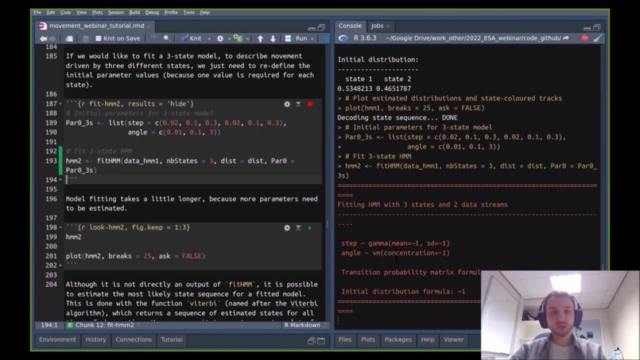 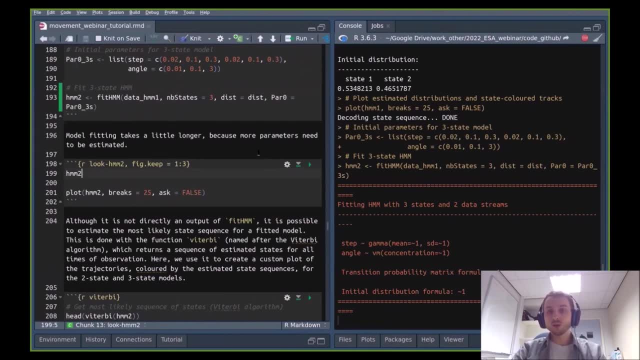 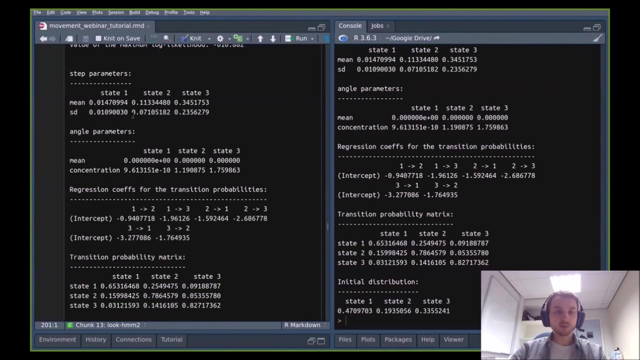 It takes a little bit longer because there's more parameters to estimate And once we have estimated it, we can do the same thing as before: We can print it to get the parameter estimates and we can plot it to get all those plots. So if we print it, these are estimates of our parameters of step lengths and turning angles and transition probabilities. 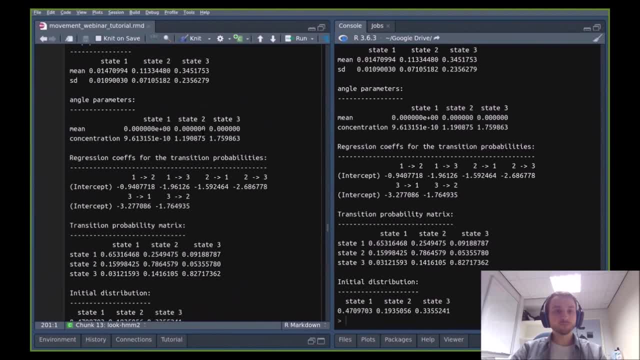 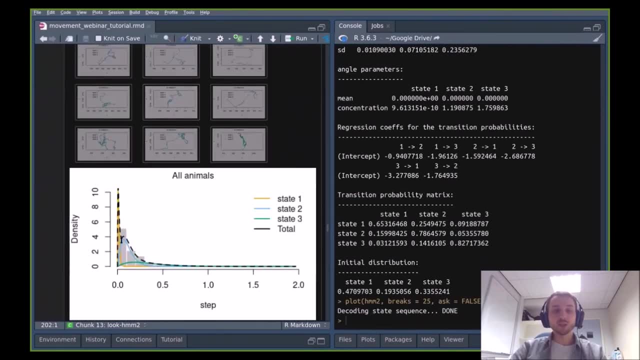 But this time there's three columns, because one for each state And we can also make the plots, And so this time there's three curves. And so here you can see that the first state captures still very short steps. The blue state captures maybe intermediate steps. 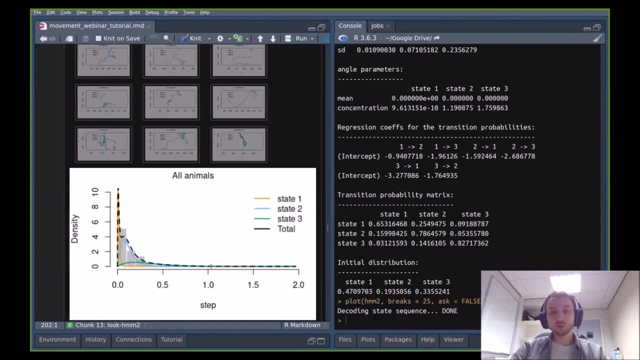 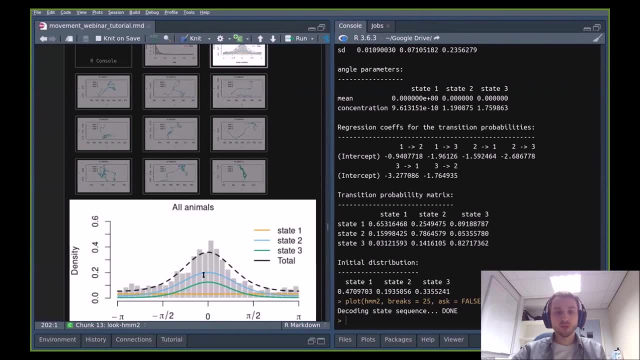 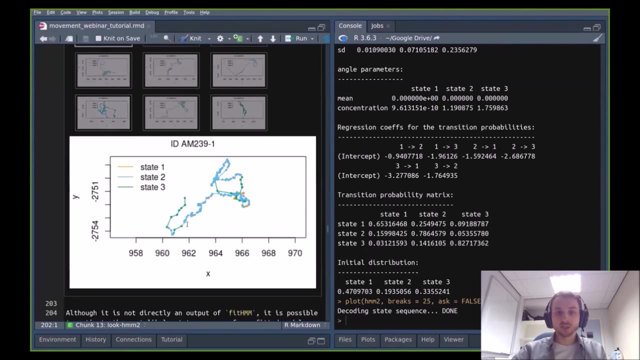 And the green state captures the longest steps. So you have kind of these three pretty distinct states that capture different types of movement, And here this tells you something about how directed the movement is in each state. Okay, You can also plot them Here. you see that this is kind of what you would expect. 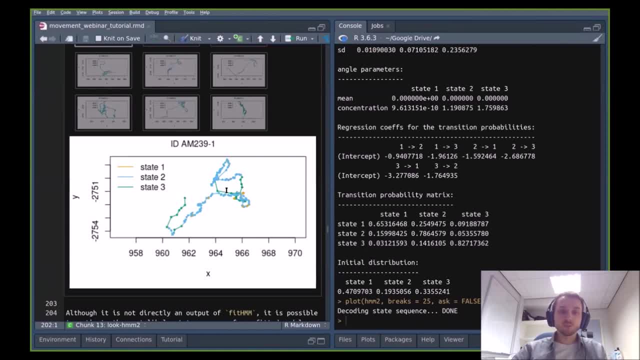 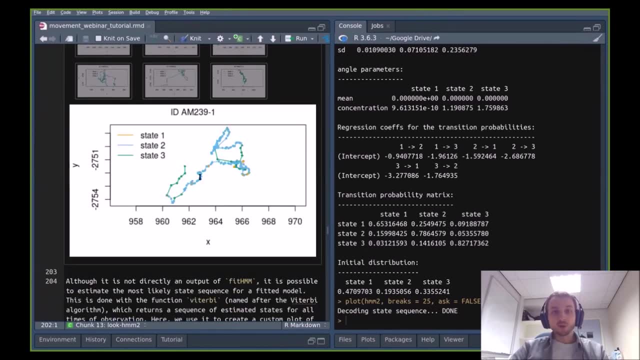 Very slow movement is in orange, Intermediate movement is in blue And very fast movement is in green. Okay, Okay, So a three-state model. And again, how do I choose whether to use a two-state model or a three-state model? 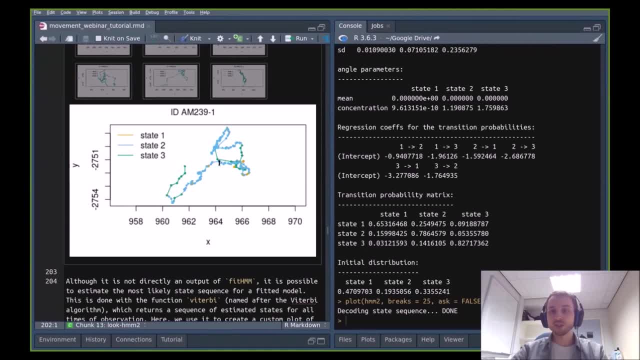 There's no super clear guideline, It's just mostly about biological expertise. And again, I direct you to that JABES paper, the Pollitt-Alt paper 2017.. And I'll also use this to see a discussion of this. 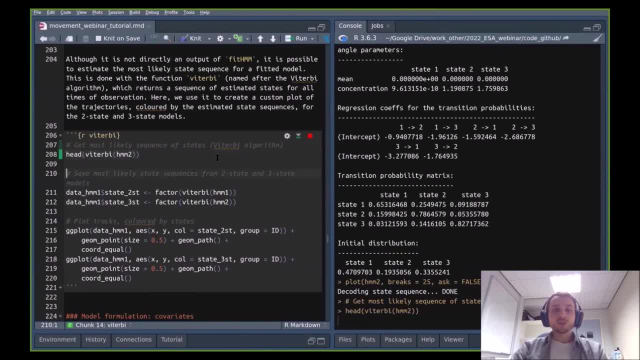 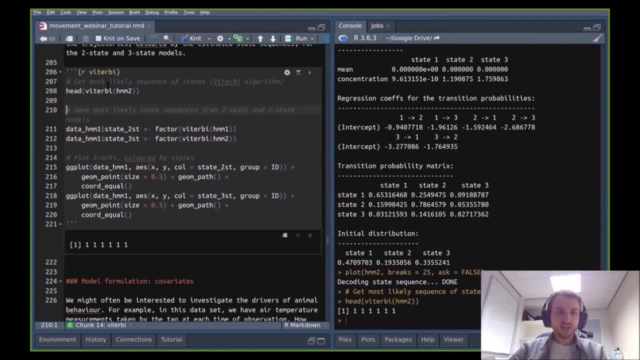 Okay, Okay. One thing we're actually interested in doing with these models is to get an estimate of what the animal was doing at each time step through our data set, And there's a function in R and Momentum that's called Viterbi to do this. 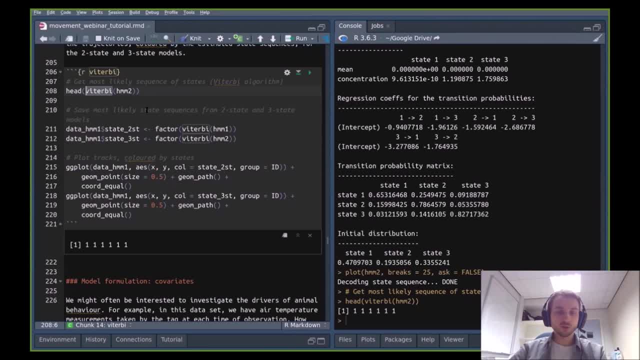 And Viterbi uses the Viterbi algorithm- That's what the algorithm is called- to get a sequence of numbers, And there's as many numbers as there are time steps in the data And for each time step it tells us here, it tells us that it was in state 1, 1, 1, 1, 1, 1 for the six first time steps. 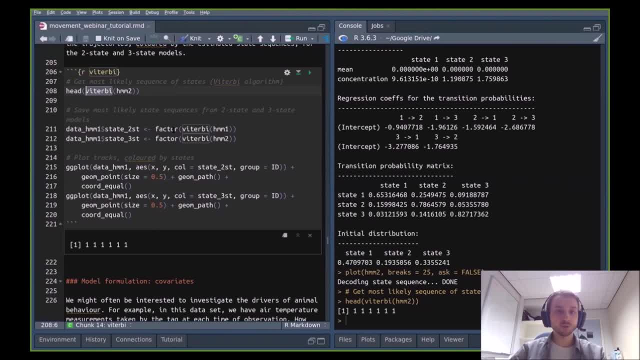 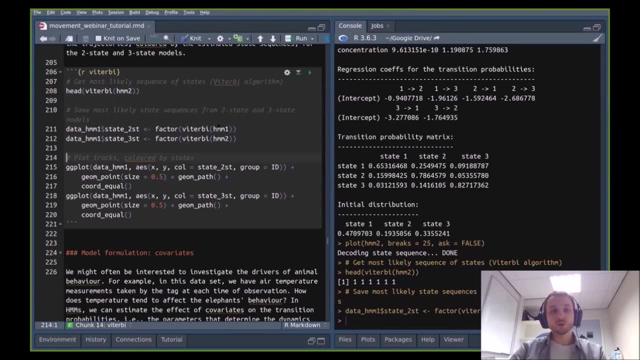 And then it would switch to state 2 or 3 or something at some point. So here, what I'm doing is I'm adding a column to the data set with the estimated states for the two-state model and the estimated states for the three-state model. 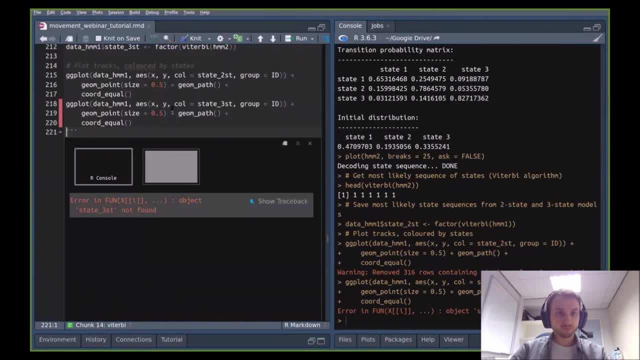 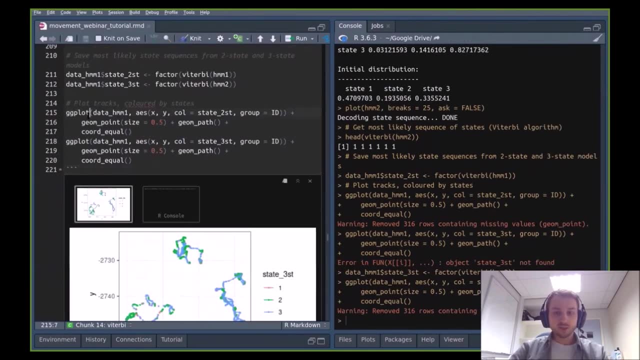 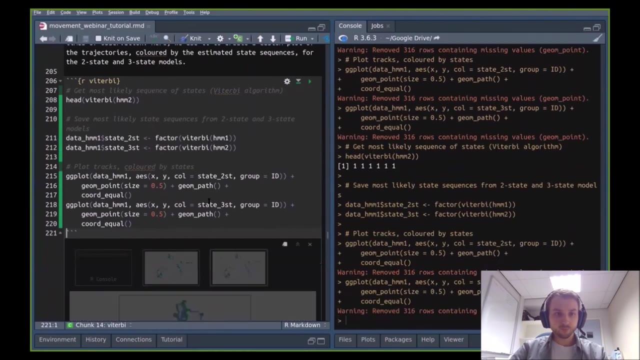 And then we can plot these. Do I not run this? Yeah, We can run this. Okay, So we can run this, And I guess I can get both of these. Here we go, And here this is the estimated states for the two-state model. 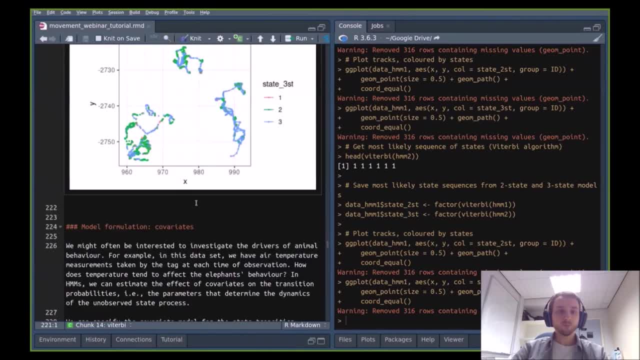 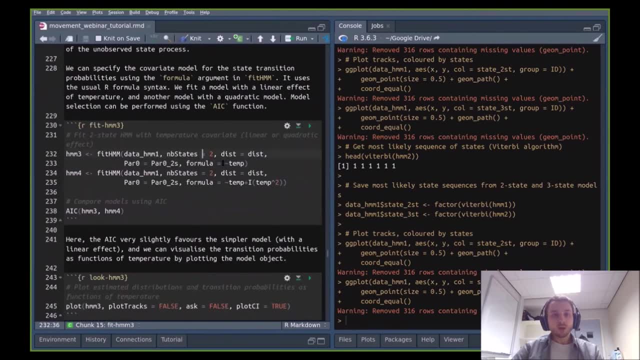 This is the estimated states for the three-state model. Okay, So all of this takes just one line of code with this Viterbi function. Okay, An extension- maybe the most useful extension in these models, because normally we want the number of periods on the transition probabilities. 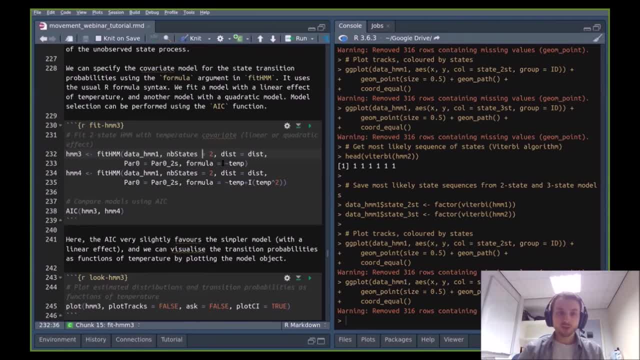 So we want the probability of the animal being in the foraging state, say, to depend on temperature or something, And we can do that using the formula argument in fit HMM in that function that I've used, I've been using to fit models. 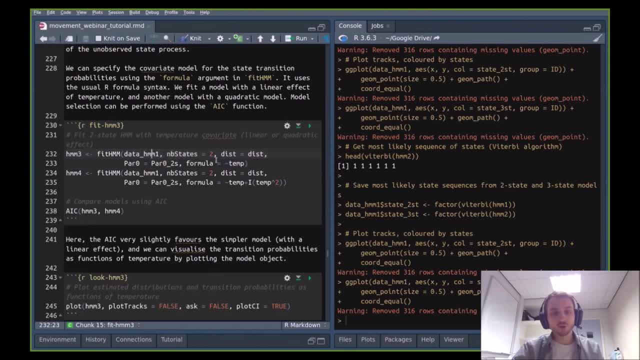 So here I'm using the same function call as before, except I've used this, this formula, and this indicates a linear effect of temperature. I could also fit a model with a formula like this, which indicates a linear Natural Z-interference indicates a linear and a quadratic effect of temperature. 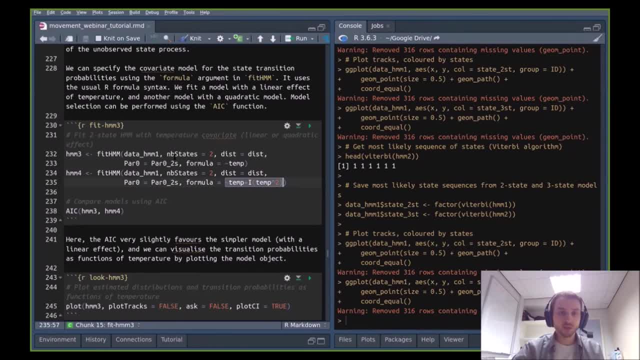 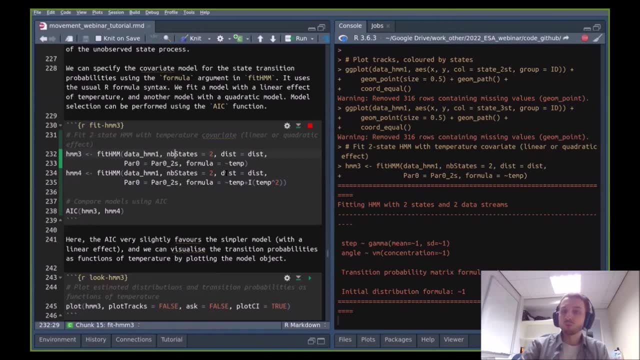 This just takes the standard R-formula syntax. okay, So let's run both of these Again. it's gonna take a little bit of time because now there's more parameters to estimate. We need to estimate the effect of the covariates. 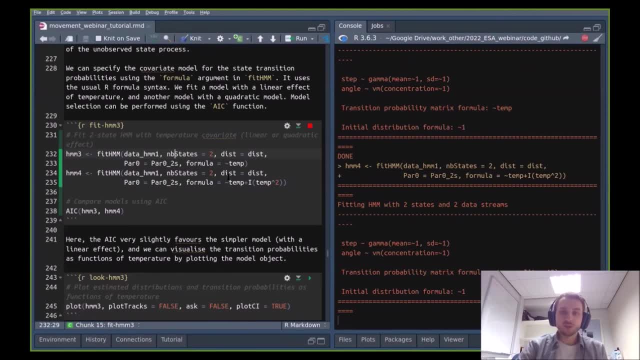 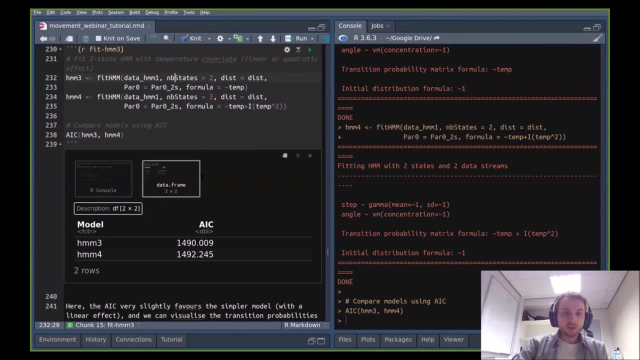 and the transition probabilities, And then I'll show you what kind of interpretation we can have from this. Okay, so first thing I wanted to say is that you can use AIC to compare these models, So when you have different covariates formulations. 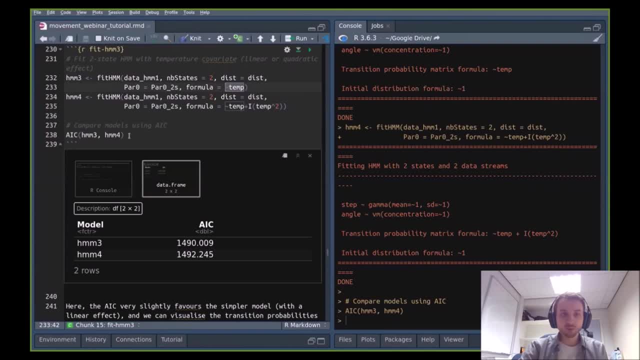 you can compare those with AIC. In this case, for example, I just used the AIC function on those two models And it tells me that the HMM3, which was the model with a linear effect, is very slightly favored by AIC. okay, 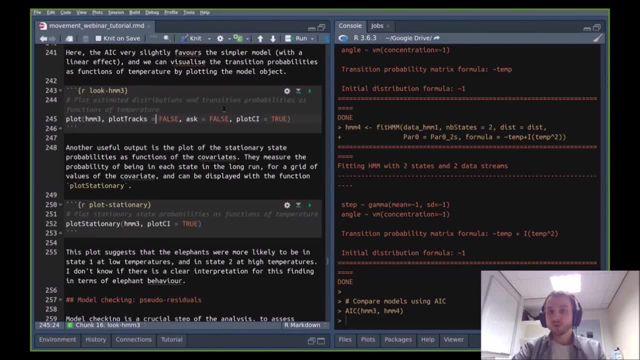 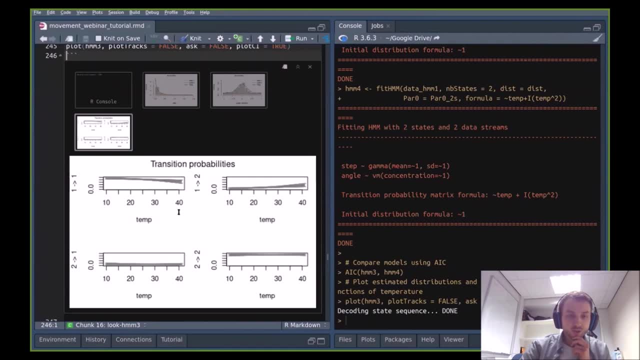 So then, if we want to try to interpret the effect of temperature on the transition probabilities, we can try to plot the model, And when we plot the model, a plot like this is gonna show up, And maybe can I try to do it here. 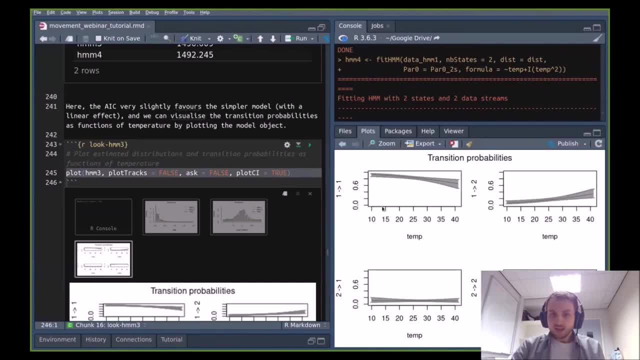 because it's a little bit squished, Yep, And what this is showing is: so this is the probability of transition from state one to state two, So from slow to fast, and this is the transition probability from fast to slow, And it's showing it as a function of temperature. 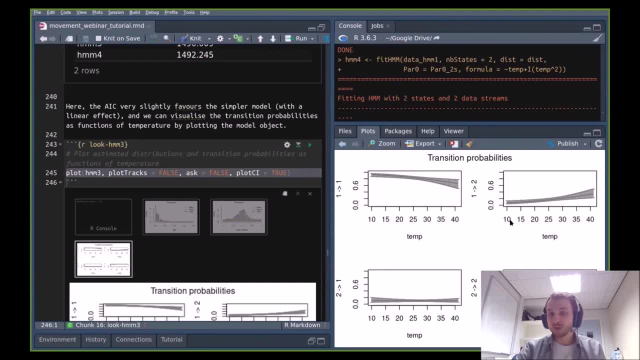 with some confidence band, And so the main pattern that emerges from these plots- and I'll show another plot a little bit later that might be a little bit clearer- is that this transition probability increases with temperature, So it's more likely to transition from slow to fast. 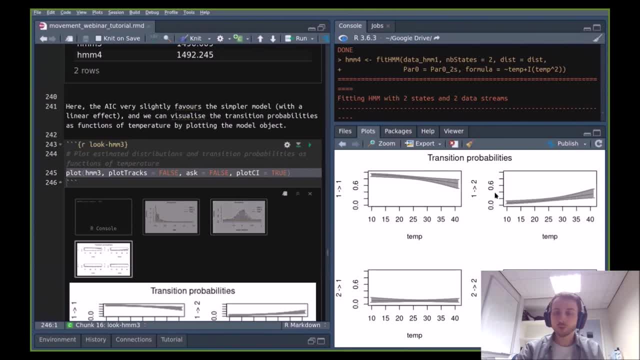 when it's warm than when it's cold. okay, And so with this, as you can imagine, you can infer, you can make a lot of ecological inferences about the effects of environmental covariates on animal behavior. I think these can be a little bit tricky to interpret. 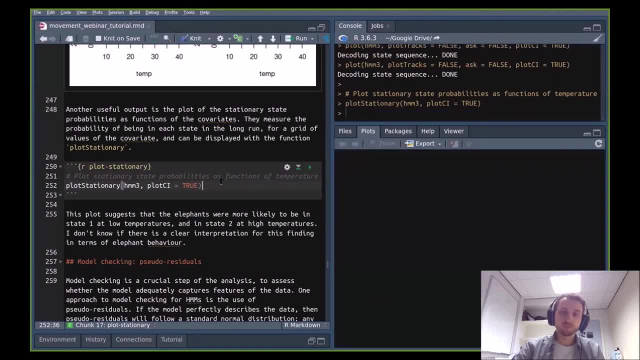 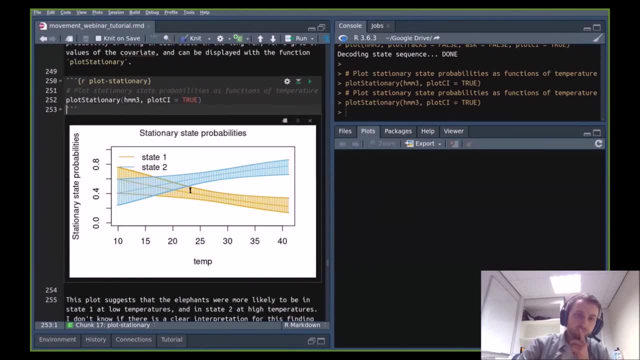 And so another type of plot that I find a little bit more, a little bit easier to interpret is a plot of stationary state probabilities. So what this is showing? again, it has the temperature on the X-axis, but this time it's showing us: 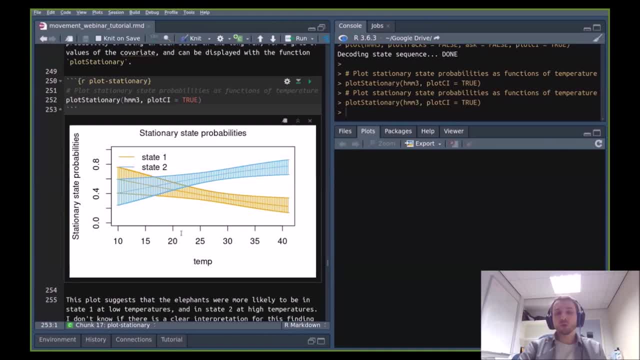 the probability of being in a state if the covariate was fixed to that value for a long time, And so, for example, if it was 40 degrees, you would have, you know, almost 80% probability of being in state. two: 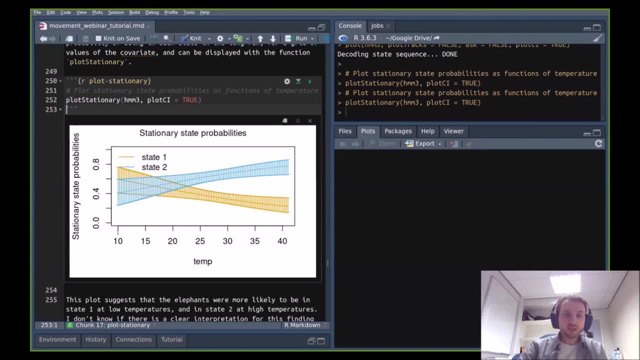 about 20% chance of being in state one, Whereas if it's 10 degrees, there's a 40% chance of being in state two and 60% chance of being in state one. okay, And so you can make inferences about you know. 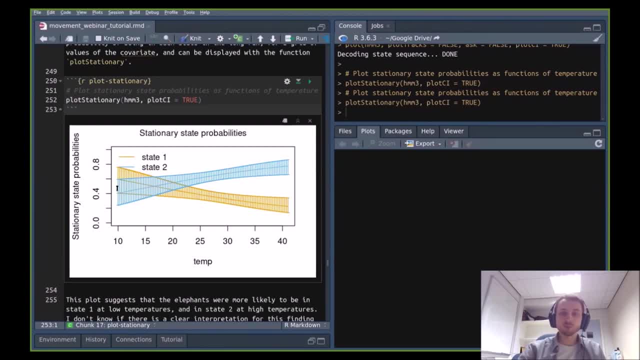 at what temperatures is it more likely for elephants to be foraging? At what temperatures is it more likely for them to be transiting, et cetera. And I should say that this interpretation here, or this, what I'm finding here, is that 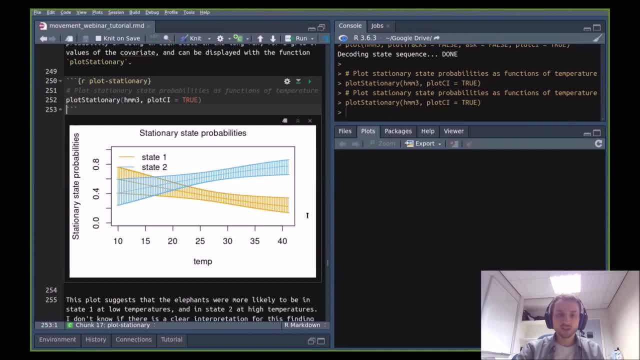 elephants are more likely to be in their kind of active movement states when it's warm, And I think that goes kind of against what I've heard from people who actually know about elephants, which is that they kind of they don't like heat very much. 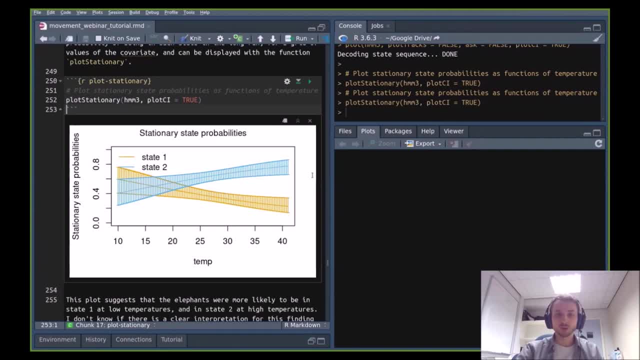 and they tend to rest in the shade when it's hot. So I don't have a very good biological explanation for why this pattern shows up. Maybe it's just you know. maybe it's just that the 2000 observations I subsampled from the data have this weird pattern. 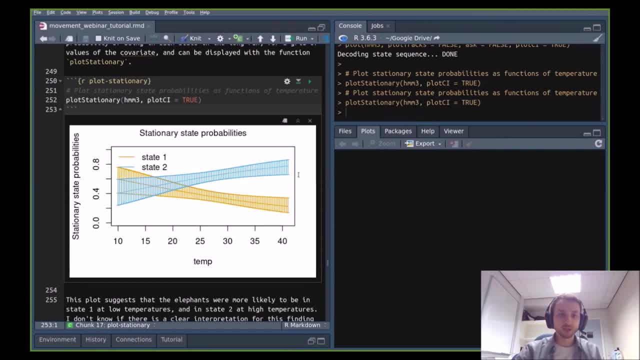 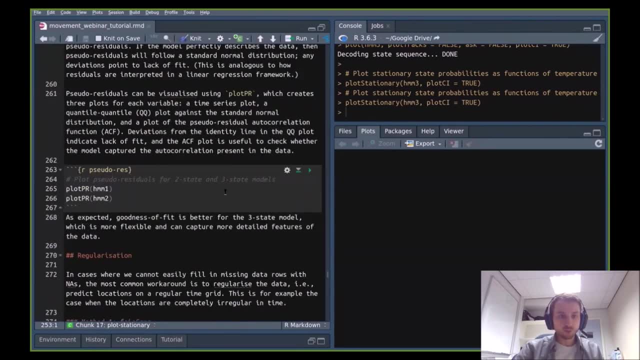 that the rest of the data wouldn't, or something. Anyway, I'm not making any biological claims again. Okay, I'm conscious of time, I should probably hurry up a little bit. There's a method called pseudo residuals, to check goodness of fit in these models. 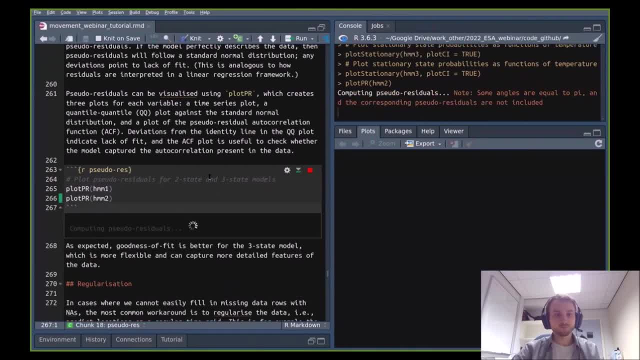 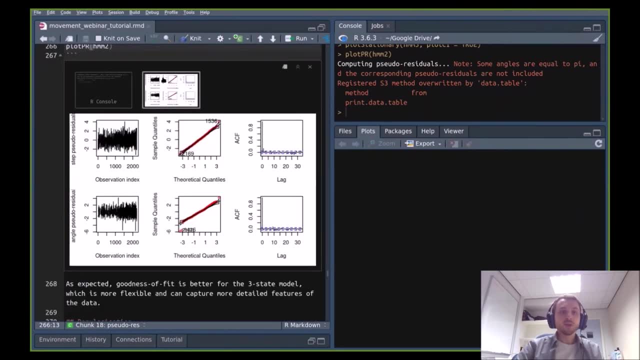 And maybe I'll just show for one model. Let's say this one: There's a function called plot PR that plots pseudo residuals for a model in momentum. And those pseudo residuals, they're a little bit analogous to residuals in linear regression or something. 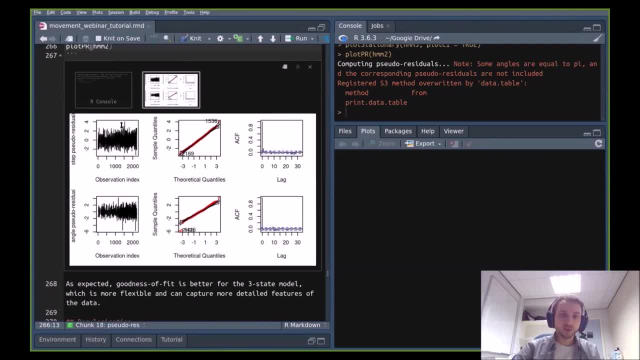 They're supposed to be independent and normally distributed And these plots show you some kind of diagnostics that show you whether or not they are. And so these, in particular these are quantile-quantile plots of the pseudo residuals against the standard normal distribution. 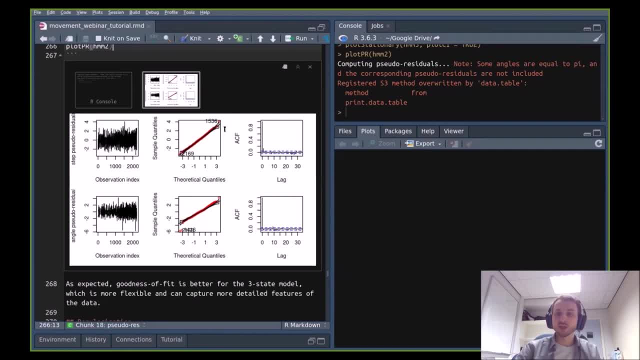 And so deviations from this kind of diagonal line suggest lack of fit right, A little bit like you would do in linear regression. So here this is the three-state model. Actually it seems to fit pretty well, And you get pseudo residuals for the step lengths. 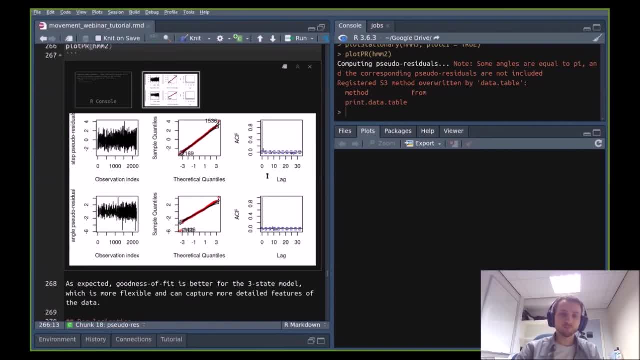 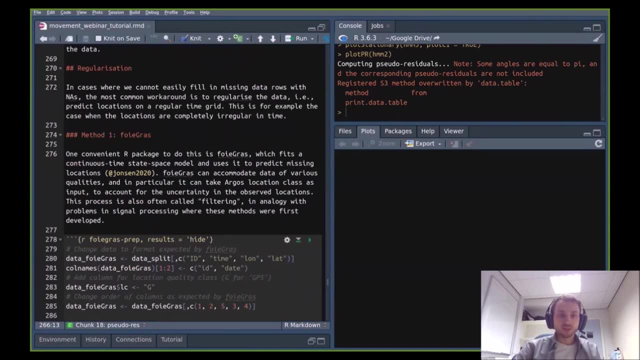 That's what's written at the top, and for the turning angles, which is what's shown at the bottom. Okay, so I went a little bit fast on this because I wanted to have a little bit of time to talk about regularization. So what I did throughout this analysis. 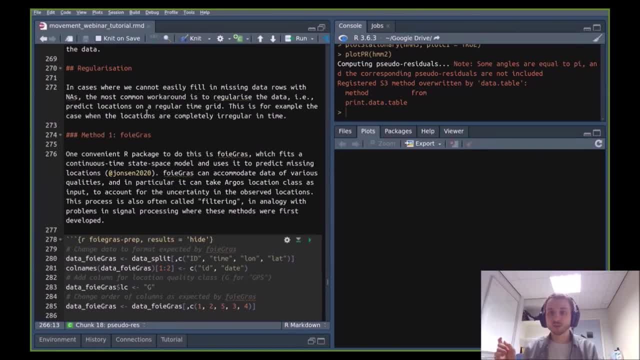 is that I put missing values in rows of data that were missing when there were gaps in the data sets. I just put missing values, But in some cases you might not have that option, for example, if your data are completely irregular. right, 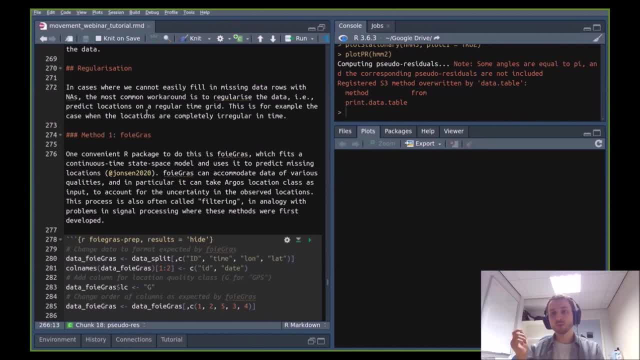 If it's not even missing values on a regular grid, if it's just like- sometimes it's 37 minutes, sometimes it's 23 minutes, sometimes it's seven minutes, just depending on when the animal comes to the surface or something. 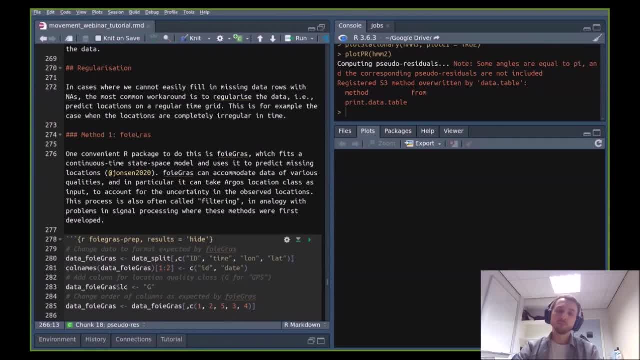 And so in this case you're gonna need another piece of software- usually something kind of implementing some sort of state space model- to somehow predict the location of the animal on a regular time grid before you can apply a head Markov models, And here I'm gonna show a first example. 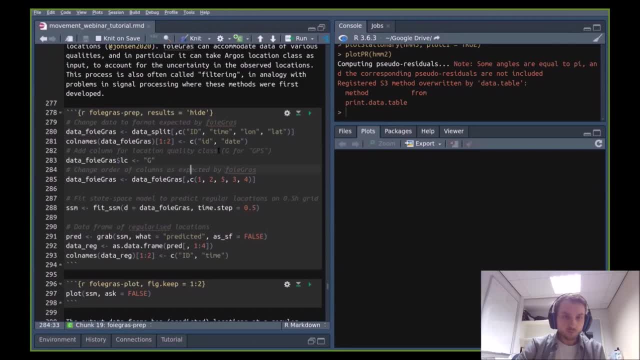 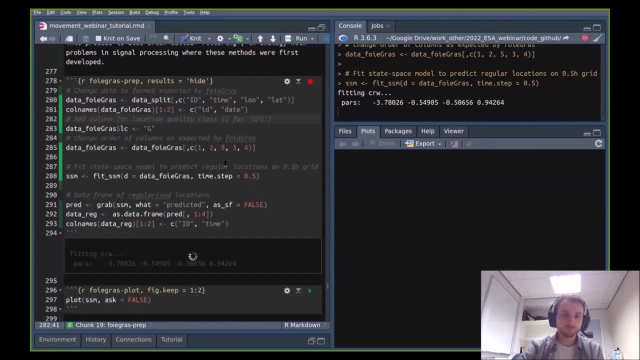 using foie gras. Okay, so I'm not going to go into the details of what this code does. It just fits a foie gras model to the data and then predicts on a half an hour time grid. There's a little bit of code. 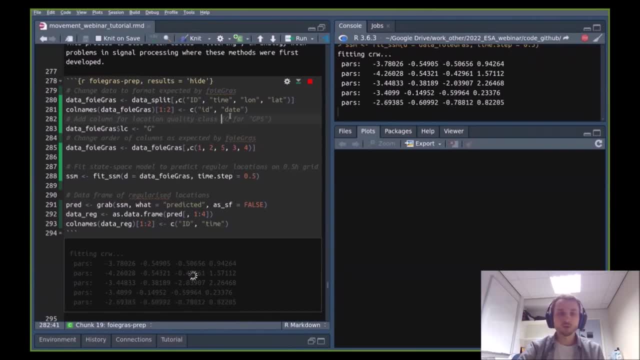 that's really just to change the names of the data columns and stuff, because different packages have different expectations, but this looks, I think, more complicated than it really is. But the main thing is this: this fits the state space model in foie gras. 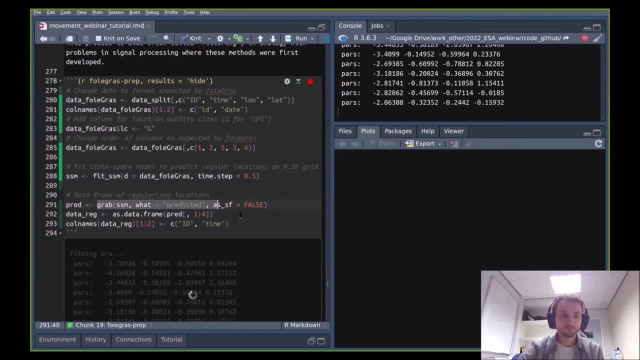 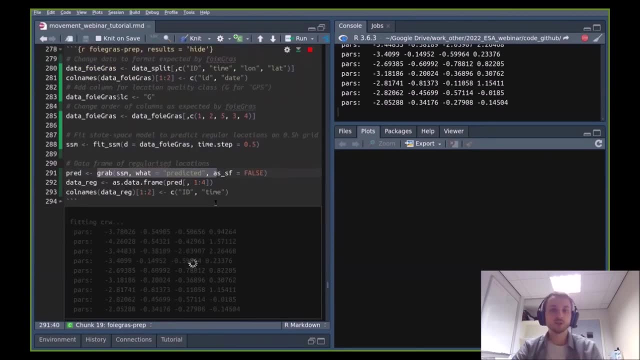 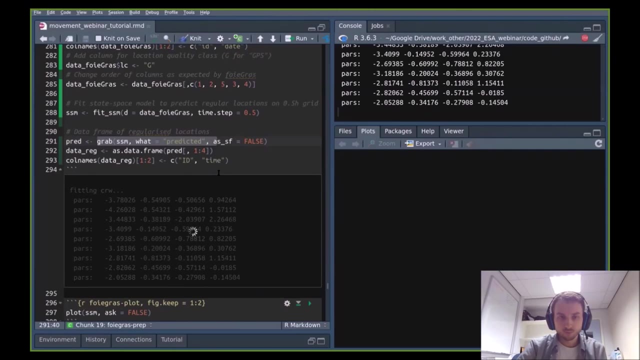 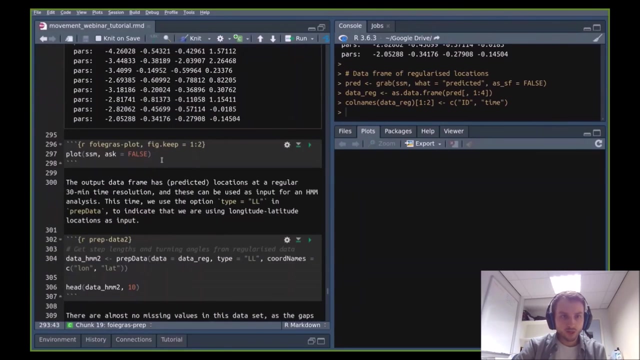 and this gets the predicted values. Okay. so right now I'm waiting for this to finish and I'll just show you what the regularized tracks look like. Okay, I think it's done now, So you can plot in foie gras. 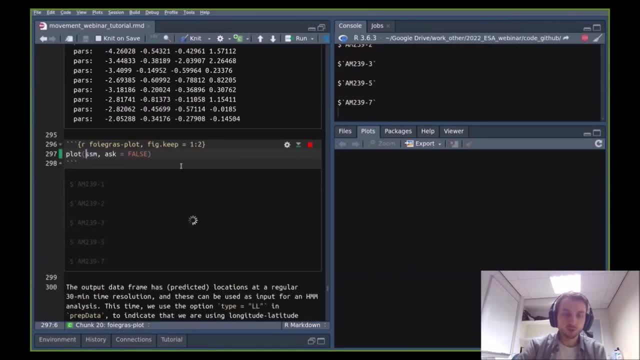 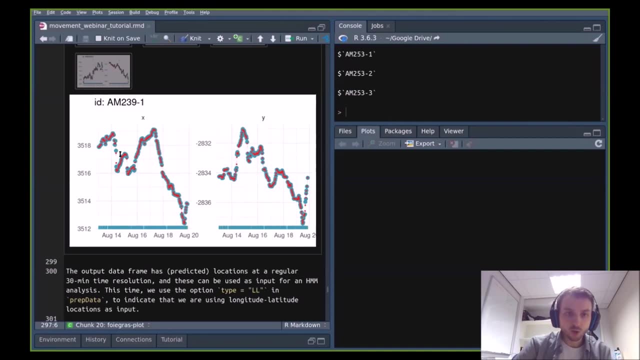 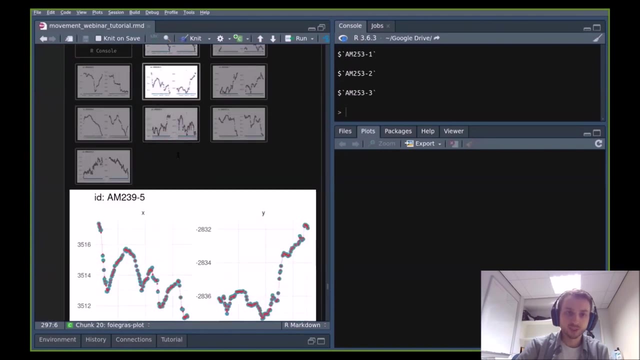 you can plot the fitted model, and it gives you a plot for each track of the regularized locations, And so it looks something like this, where so, I think, the blue dots are observations and the red dots are predicted locations, And so you can see that you're predicting. 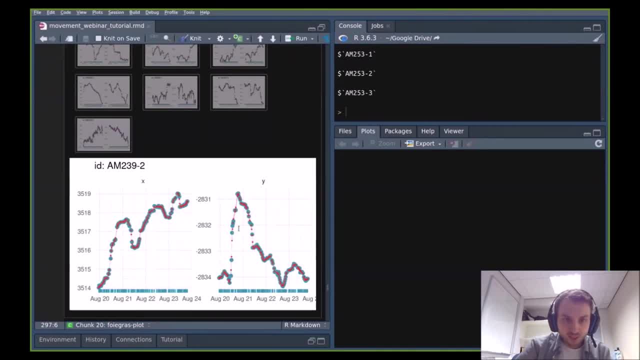 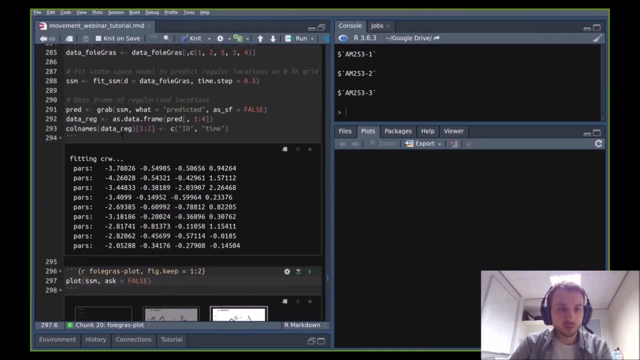 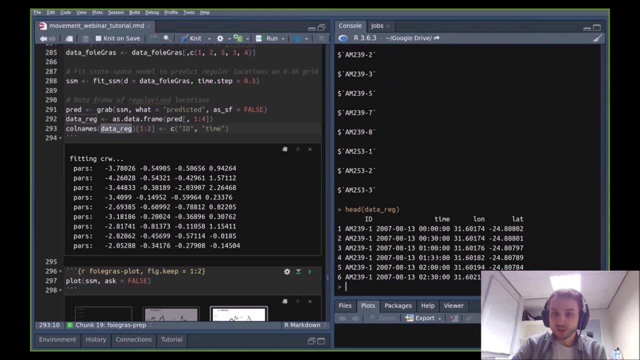 let me try to find an example with some nice gaps, Like here, for example, you're predicting some locations over the gaps to fill them right, And so if we, where is it? If we look at this, this is the regularized track. 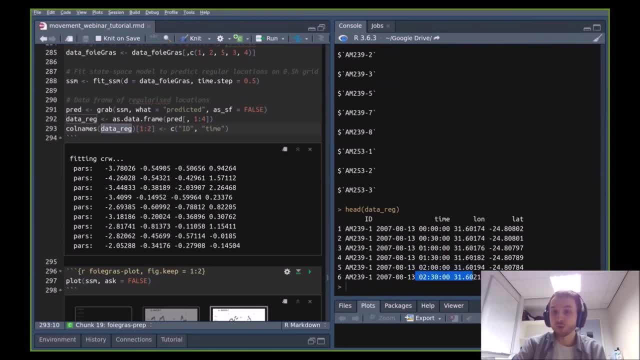 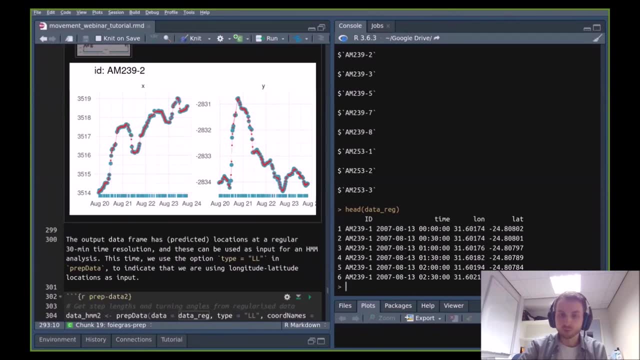 Here you see that now there's locations every half an hour with predicted longitude and latitude values, and these were obtained from that state space model. okay, So because here we have regular rows, we can directly use that in MoveHMM in Momentum. sorry, 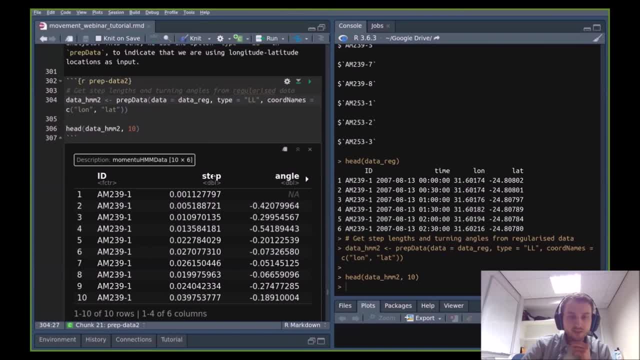 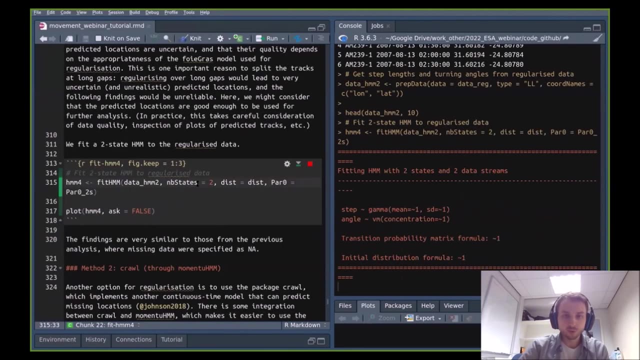 Okay, So I'm going to take this regularized data set and estimate step lengths and turning angles. This time there's no missing values in the step lengths and turning angles, because we filled in all those gaps with predicted locations right, And we can fit a model just like we did before. 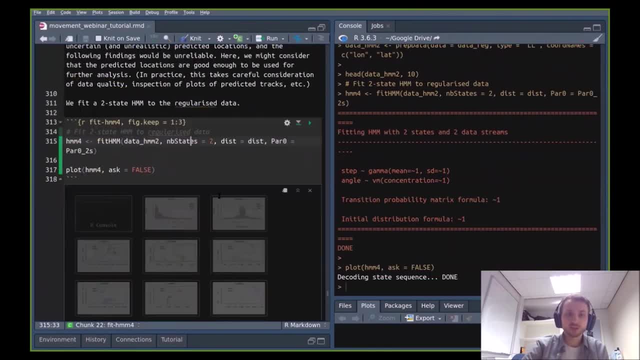 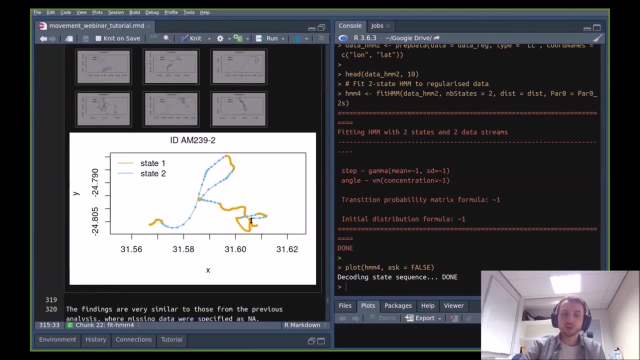 to the predicted, to those like regularized tracks, And we get something like this where now we don't have any gaps anymore, It's all regular, regular, regular locations. So we can see that this is a very good example of how we can capture the same data. 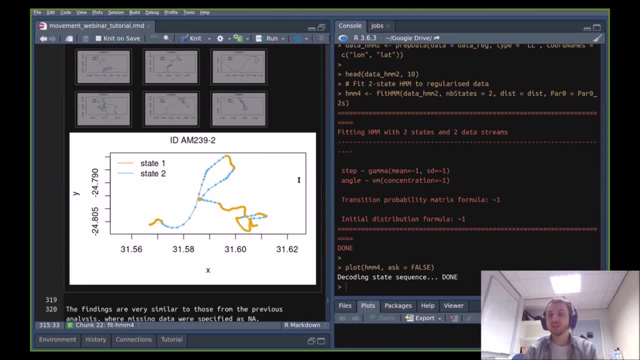 and the same locations obtained from that state space model. And, as I mentioned before, this is a little bit risky because here we assume we take as data something that was obtained as the output of the previous model, the state space model, And so this ignores some of the uncertainty in the data. 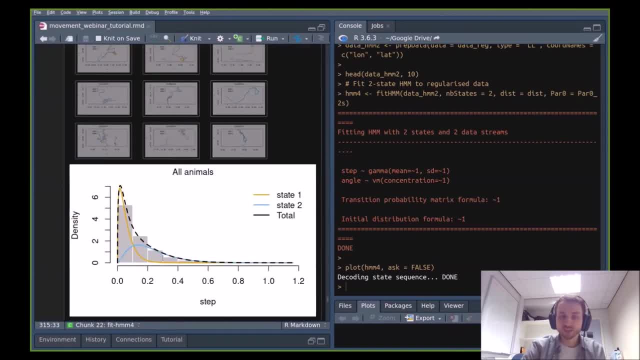 which comes from the uncertainty over those gaps of missing locations, right. But in practice in this case we get two pretty distinct states as well, just like before, that roughly capture the data, right? So we can see that we have the same two behaviors. 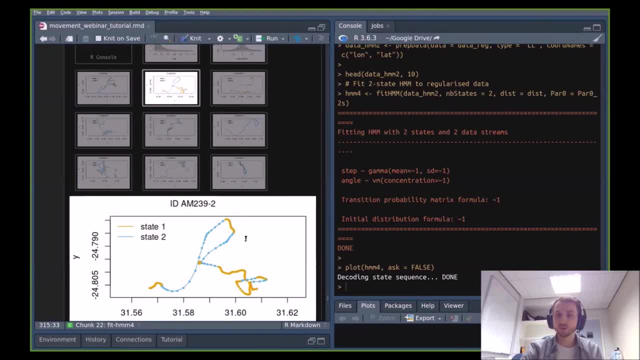 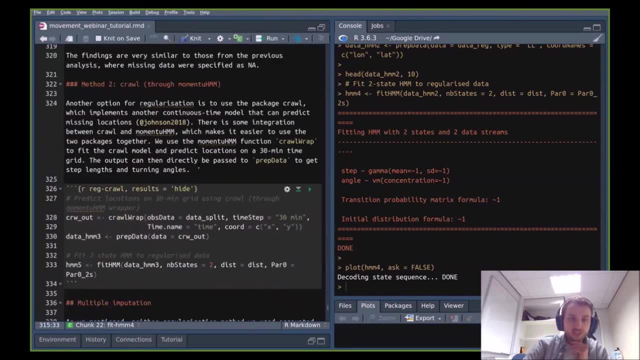 One is kind of fast and directed and the other one is slow and directed movement. okay, So this is one possible way to do it using foie gras. Another piece of software that has been used for this is called crawl, and you might have heard about it. 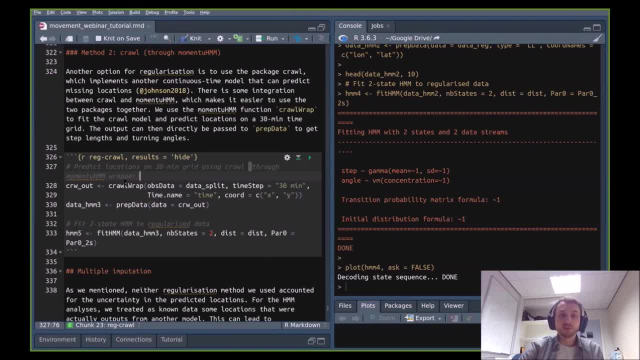 It's very popular And crawl has a nice interface with momentum, which makes this a little bit easier to integrate into your momentum workflow. There's a function called crawl wrap. That's a momentum function That does the regularization for you prior to the HMM analysis. 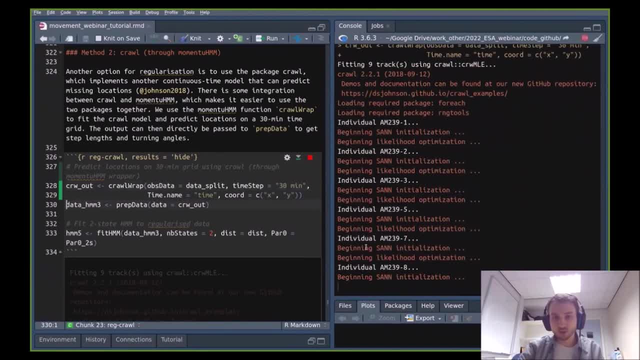 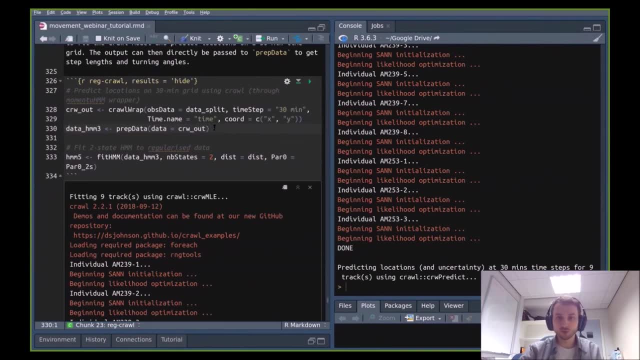 So if I call crawl wrap, it's gonna fit. So here this is a little bit similar to what was happening with foie gras. Right now, crawl is fitting some models to the tracks and then predicting locations on a regular time grid. 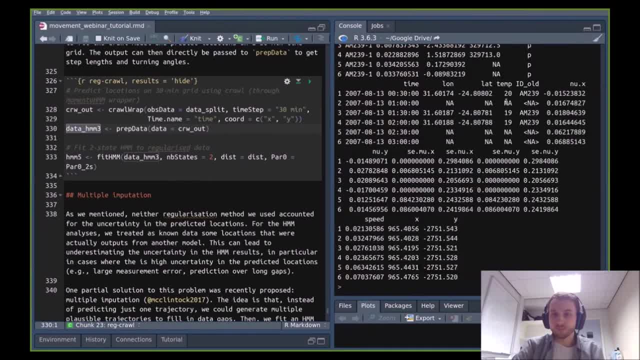 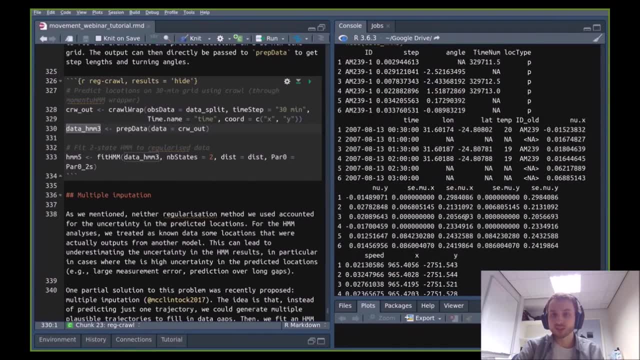 And these are the regularized tracks. The crawl ends up adding a whole bunch of data. It's adding a whole bunch of columns, but the point is that now we have regular time intervals- again half an hour every time- And so we can directly apply the HMM methodology. 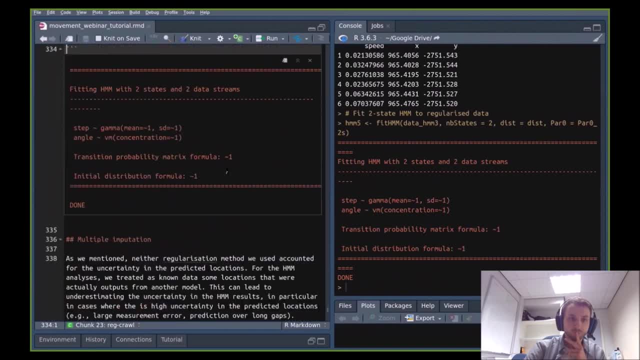 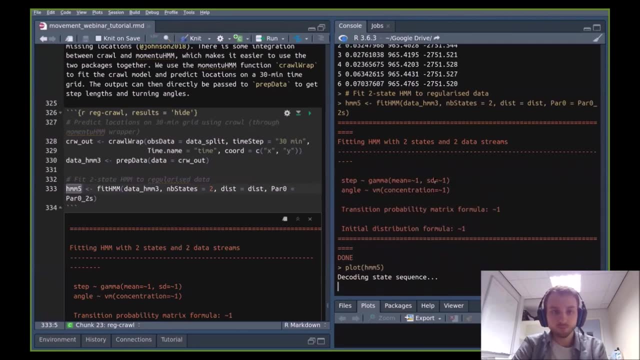 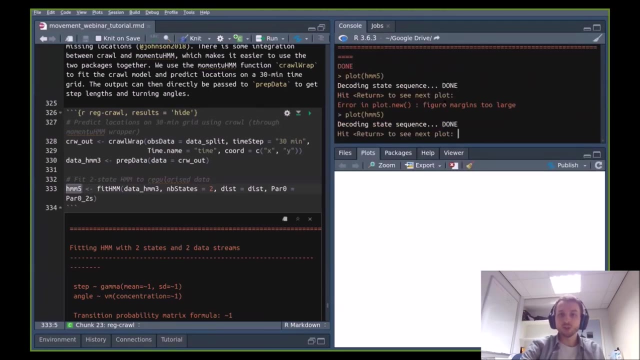 We can directly apply fit HMM to this regularized data set as well. Okay, And if I plot this, Oops. So now I'm plotting the results of the HMM fitted to the crawl data. Again, we get something pretty similar, where we get one state that captures fast directed movement. 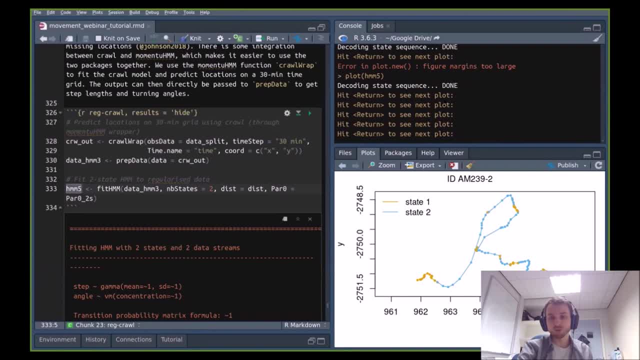 in blue and one state that captures slow, undirected movement in orange. Okay, So this is another option. So whether you do it with crawl or foie gras, there's always this problem that here we're not accounting for the uncertainty on the regularized locations. 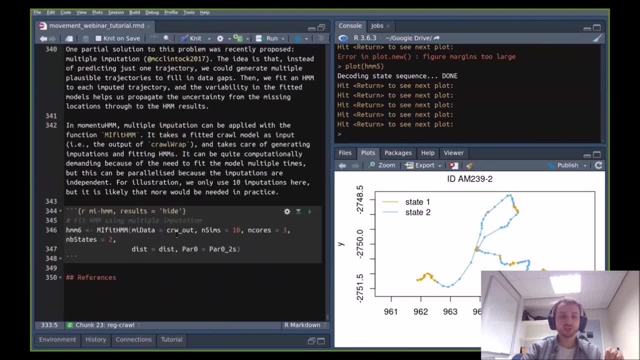 And so here I have a kind of a very brief mention of multiple imputation, And in Momentum there's a function for multiple imputation called mi-fit-HMM- multiple imputation-fit-HMM- that takes as input the output of a crawl model. 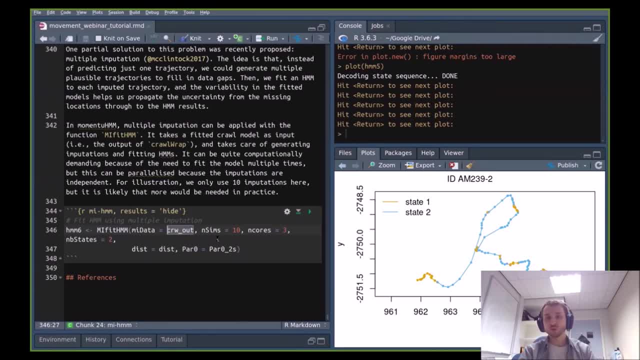 And then what it does is that it generates those plausible trajectories that I talked about from the crawl model and it fits an HMM to each one of them, And then maybe I should start running this, cause it's gonna take a little bit of time. 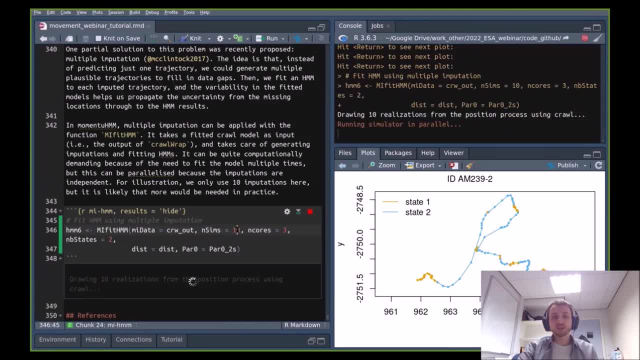 So here I passed this argument here, which means I want 10 fitted models. So I want the function to generate 10 plausible trajectories and to each one of them fit an HMM, And then the function automatically merges all the models and gives you the kind of the summary. 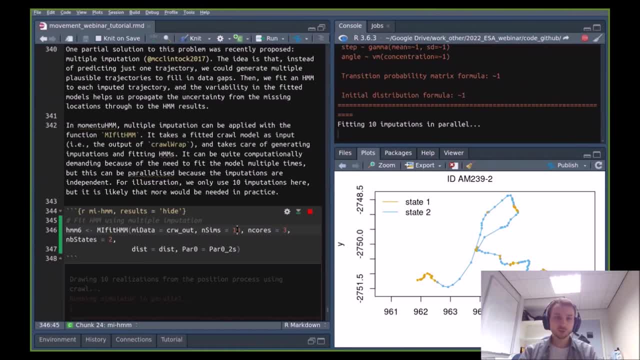 That includes the uncertainty that you had on the original data. So obviously this is computational, because you need to fit now, instead of one model, I need to fit 10 models and actually in practice I mean you should use more than 10 in practice. 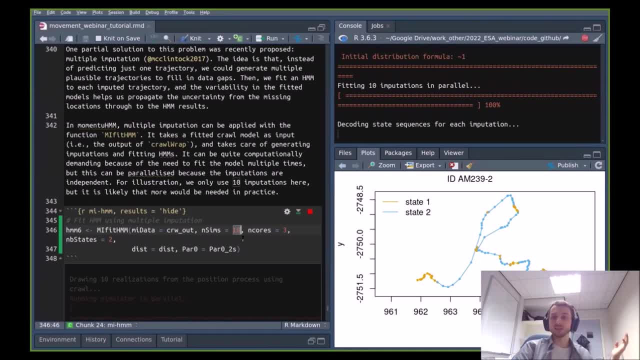 you could use 25 or 50 or something, And then the more you increase this, the better you capture the uncertainty in the data, but the more computational it is. The good news is that all those models can be fitted separately and in parallel if you want. 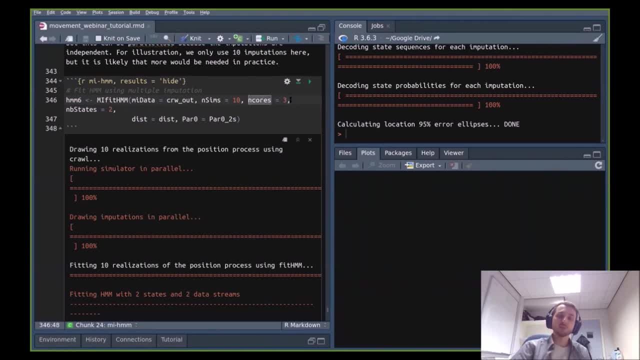 And there's this argument and cores. that lets you specify how many cores you want it to be fitted on. And so if you have a supercomputer with like 64 cores or something you can fit 64 models, It's gonna take just as much time. 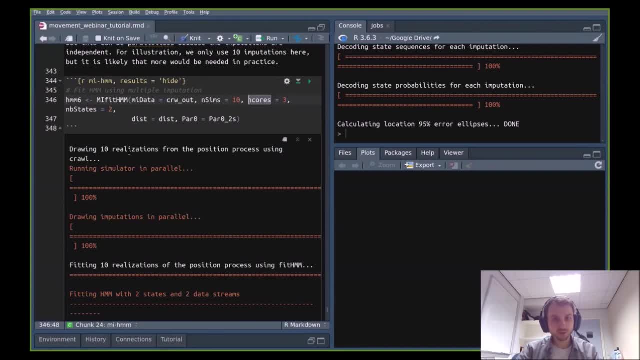 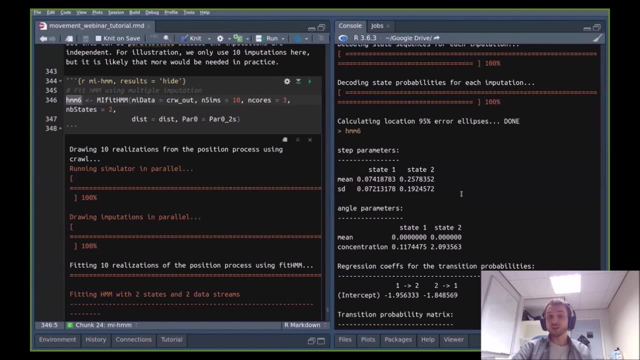 as it would have to fit one model. Okay, so now it's finished, And so we can look at the model. It ends up being just like a single model, just as if it was fitted like a single model, But the difference now is that 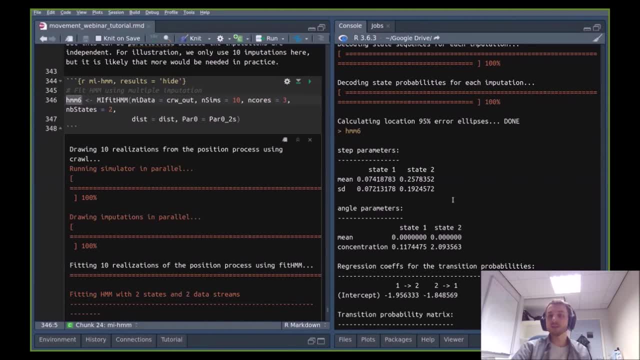 confidence that these estimates, and if I was to look at things like confidence intervals, those would include the uncertainty, not just the uncertainty on kind of one predicted track, but the uncertainty that comes from all those generating all those plausible trajectories. okay, 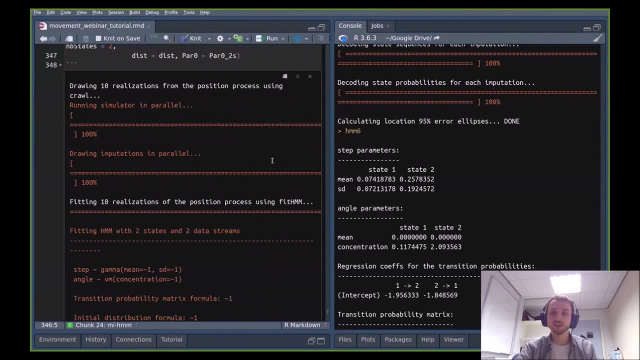 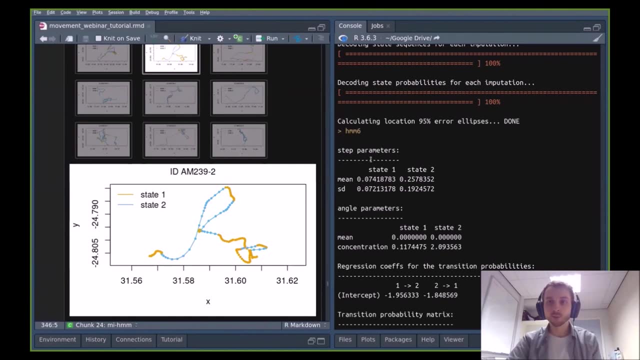 Okay, great. This takes me to the end of this document. I realize I had to go quite fast at times. I hope that you know if you go over this again and at your own pace, it will all make sense and it will kind of help you get started. 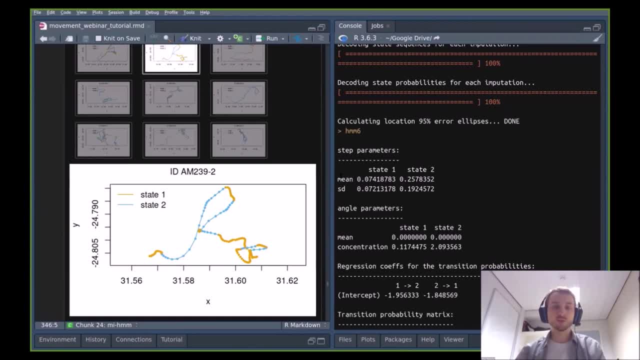 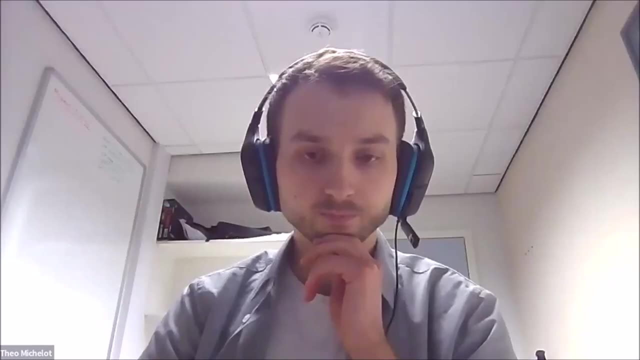 with these analyses and that you can use this code. You can use this kind of vignette to analyze your own data if you have some. okay, So thanks, I think I'll hand over to Dennis and we can take questions. Fantastic, Thank you, Theo. 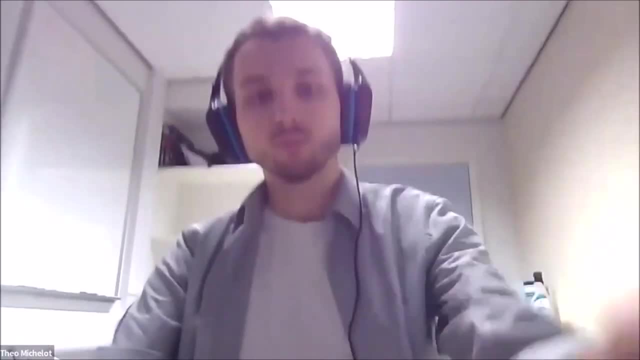 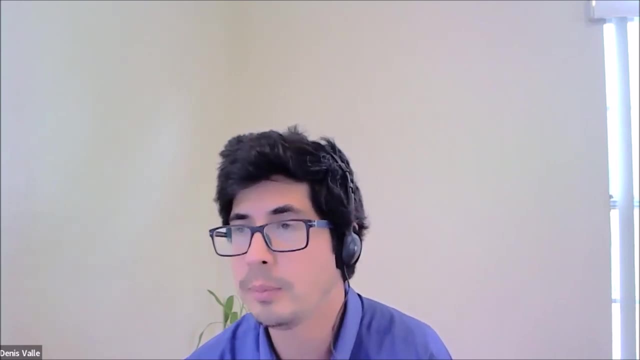 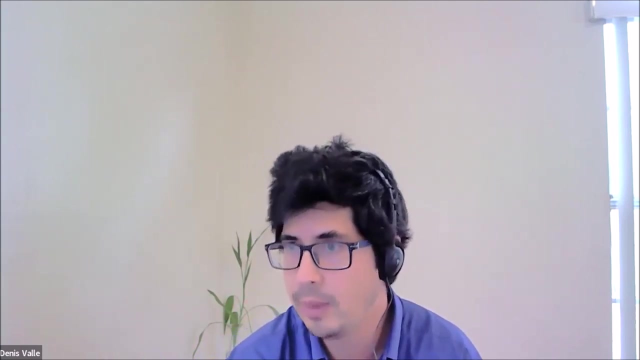 That was really very comprehensive. So what I'm gonna do is I'm gonna. I went to the paulaevcom EFI 2022 website And so if you have questions that you haven't made yet, please post it there If there are questions that are already there. 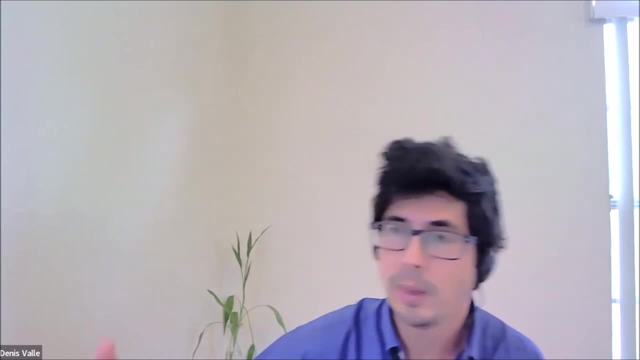 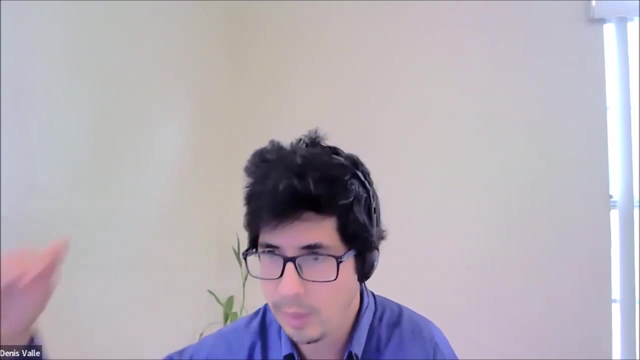 that you'd like to see answered. please upvote them. So I'm gonna start the questions by going over the ones that have been most upvoted and then I'll just move down the list. So the first question, Theo, is: you know, is you know? 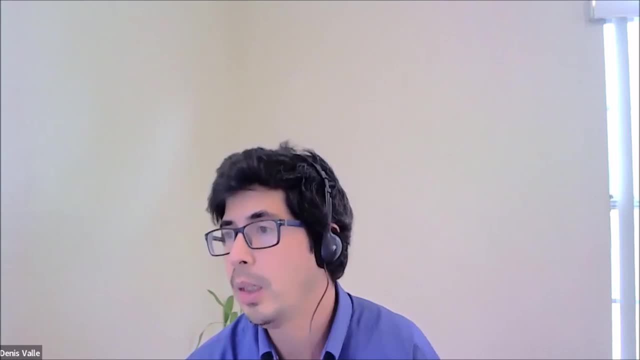 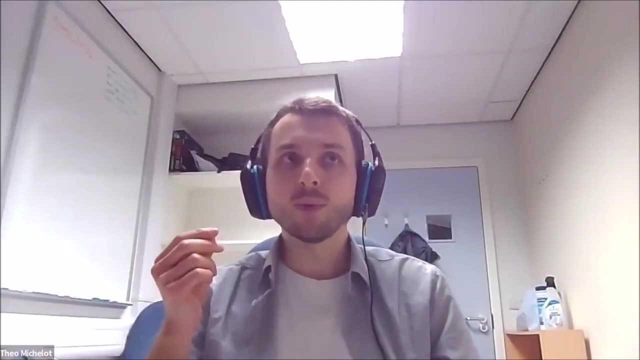 if you have preferred literature, books with a general overview of movement ecology. do you have any recommendation of a book that could help in terms of movement ecology? Okay, So I might not go as broad as movement ecology as a whole. There's a book. do I have it here? 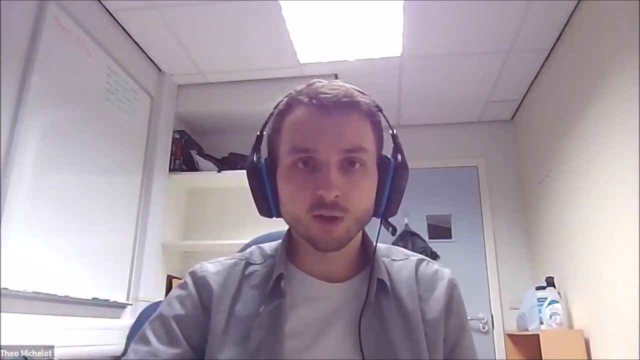 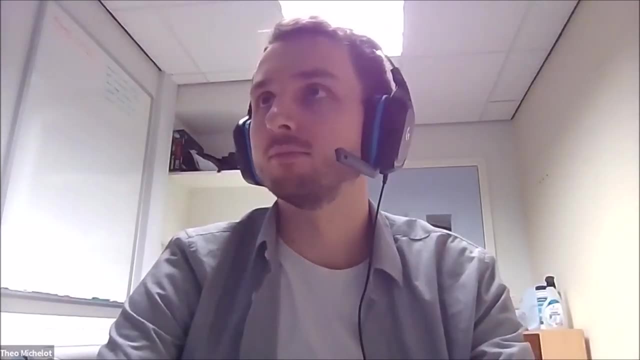 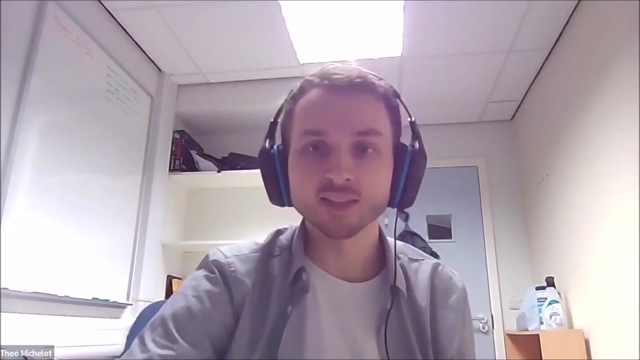 There's a. it's a book by Mevin Hutton and coauthors that came out in 2017.. I should know the title. I think it's just animal. is it animal movement? statistical models for telemetry data. So that's kind of a. it's a pretty good review book. 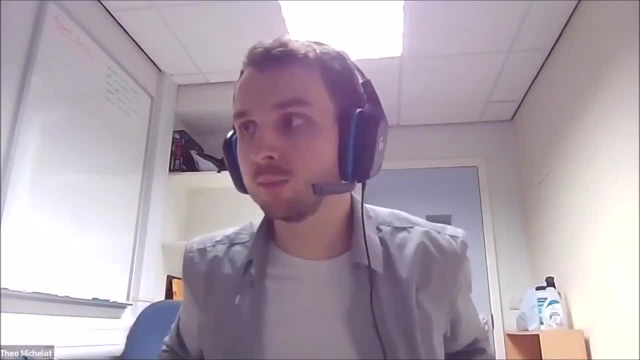 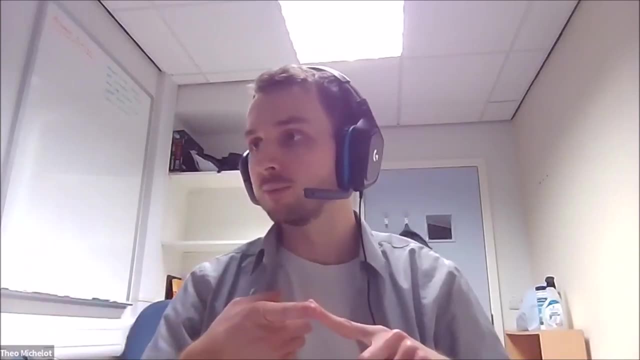 that came out a few years ago by. you know a few people who work, amongst other things, on hidden Markov models and who also work. I mean, the coauthors include the author of momentum and the author of crawl, and so a lot of people who know a lot. 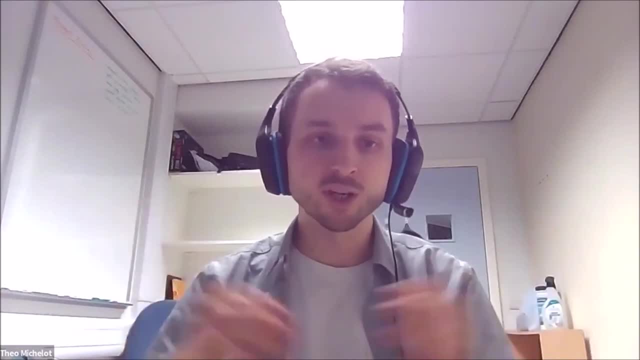 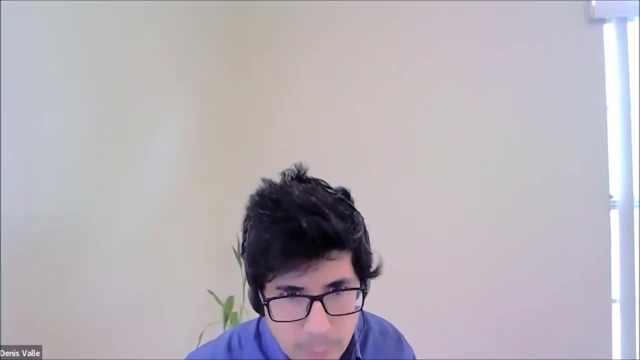 about this, So I think it's a really good starting place. I mean more than a starting place, it's a really good reference. Great, Yeah, I think somebody even posted the link here, so thank you, Emma, for that. And so the other question is: 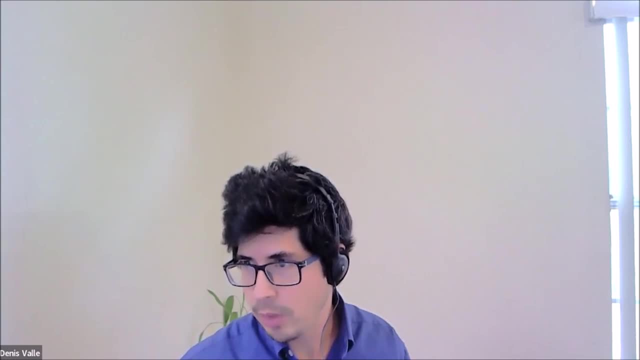 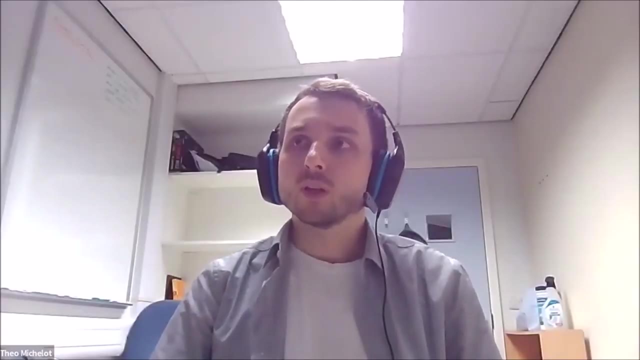 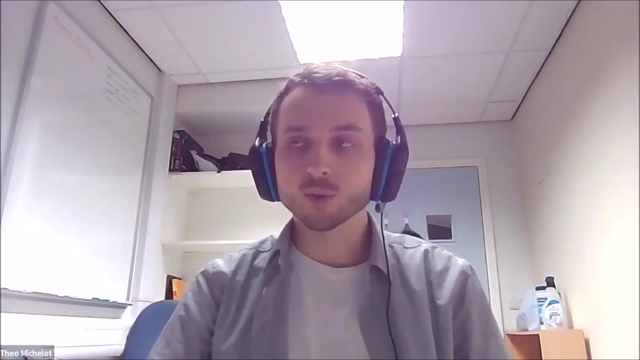 can the HMM models you implement, you know, be processed across different cores in parallel? Yeah, so to some extent. so, to the extent that I described at the end. So when you're applying multiple imputation, so then yeah, you can do that. 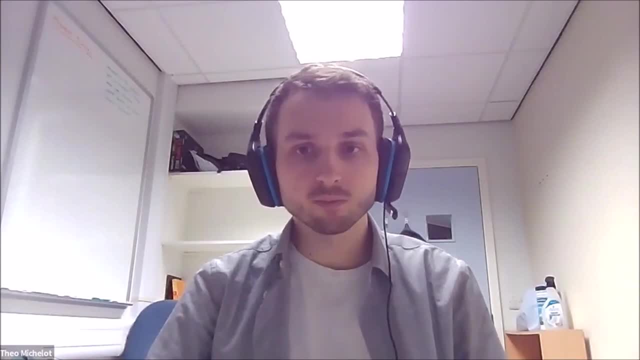 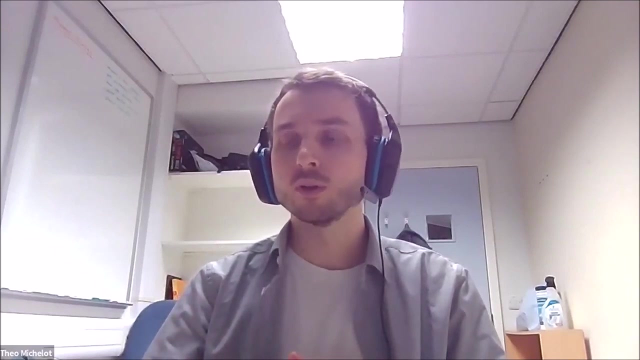 because you're fitting 25 separate models and it doesn't matter which one you fit first. So there are computational challenges to actually implementing the fitting of one model in parallel, because those models are fitted in a way or the likelihood for those models is computed in a way. that's kind of sequential. 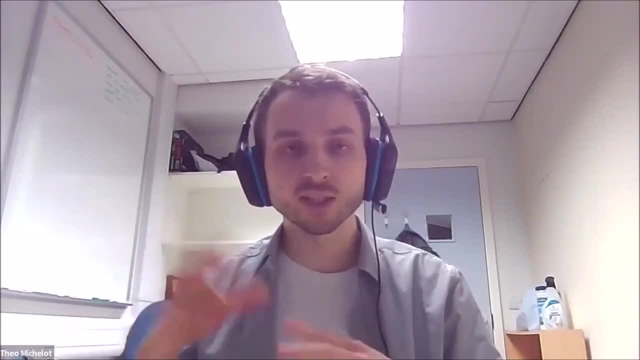 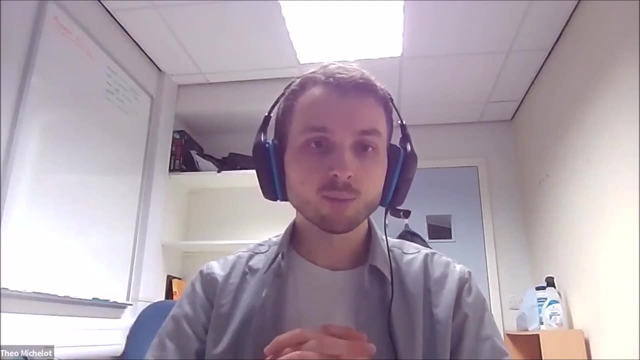 So it's a little bit tricky. You can't really just like split the data in a clever way or something to get the likelihood calculated in parallel. So it's not in parallel in general. but when you have to fit many different models, like in multiple imputation, then you can. 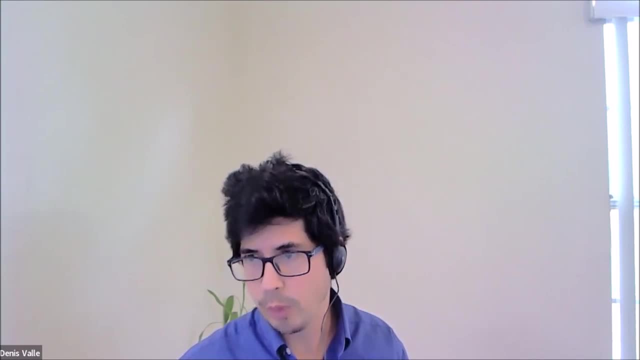 And there's one question here: When you have an estimated state for each point in the trajectory, is there some way to estimate the confidence that the state is correct? And I think part of this has to do with the Viterbi algorithm, right? 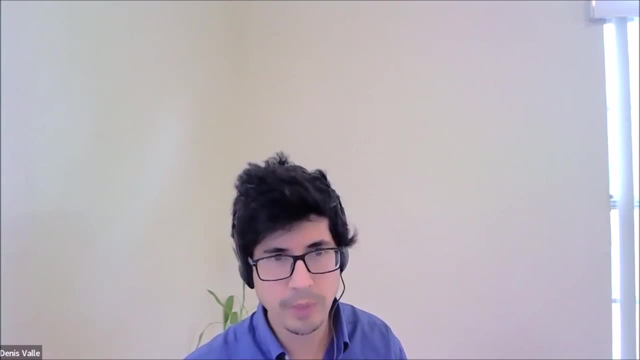 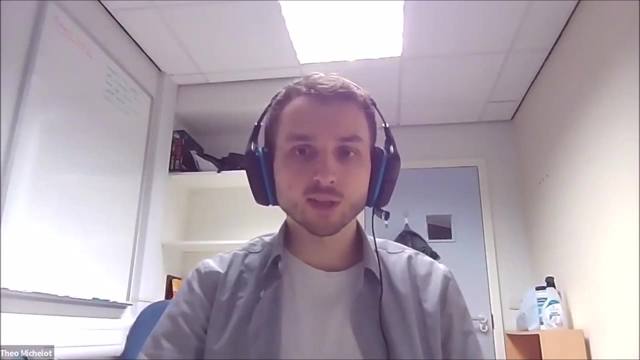 It's the most likely, but is there any uncertainty associated with that? Yeah, yeah. So I mean definitely, And that's a really good question, And it's almost kind of an active area of research. I think it's kind of tricky. 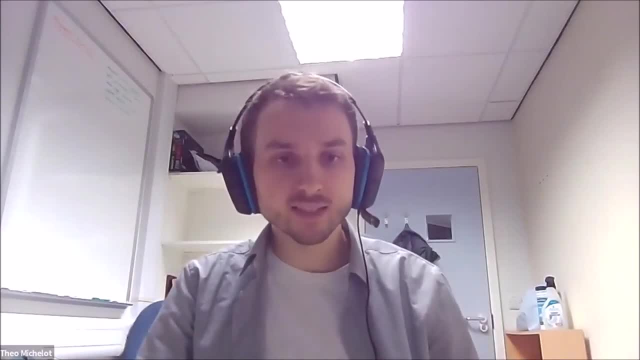 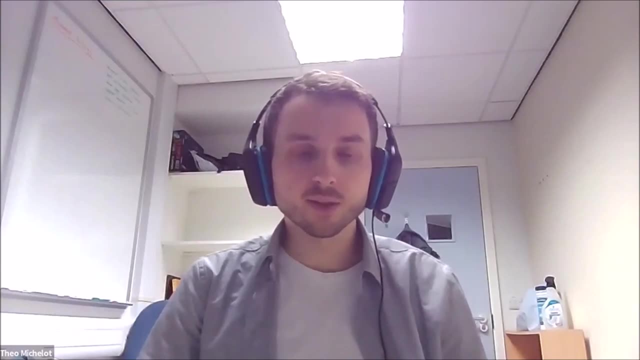 Often what people do is that they take these as granted and like the, or as data. I guess there's this estimated behavior or this estimated states, and they're not obviously the output of a statistical model And one way and the kind of the simplest way that you can. 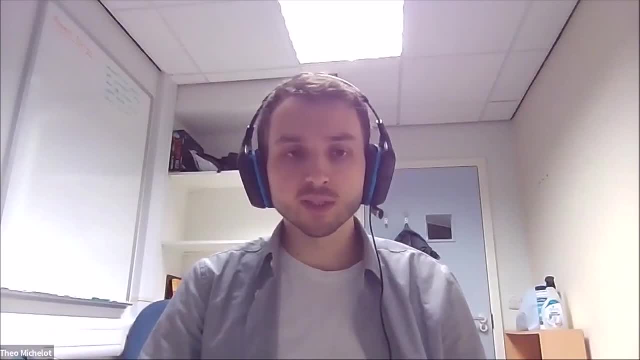 to have a better idea of the uncertainty- and that's implemented in Momentum- is to have a look at what we call state probabilities. So there's another function that I didn't show here in Momentum. that's called state probes, And what it gives you is that for each time step. 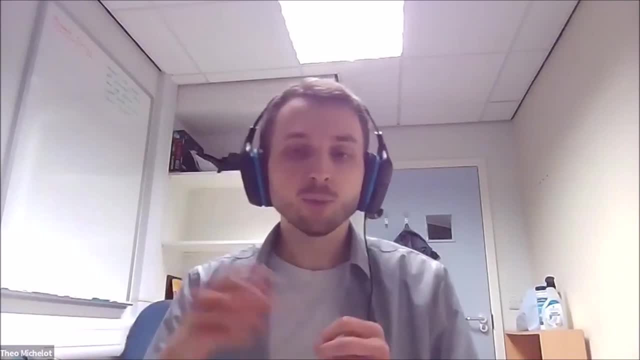 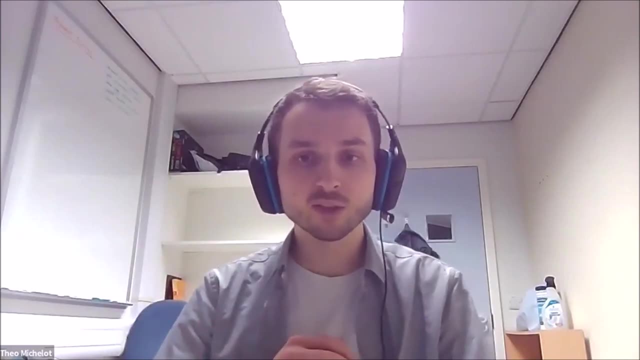 it gives you the probability of being in each state. So, for example, maybe it's gonna tell you that you know you have a 52% chance of being in state one and a 48% chance of being in state two, And so you're like, oh, okay. 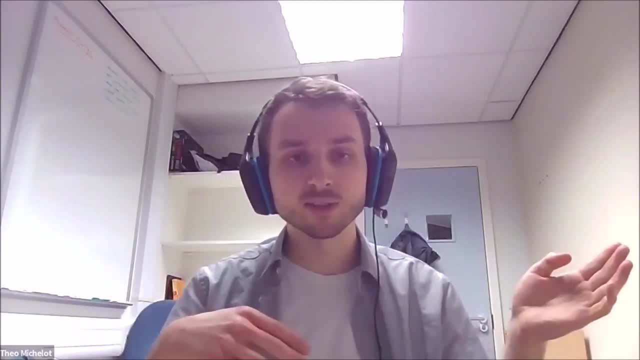 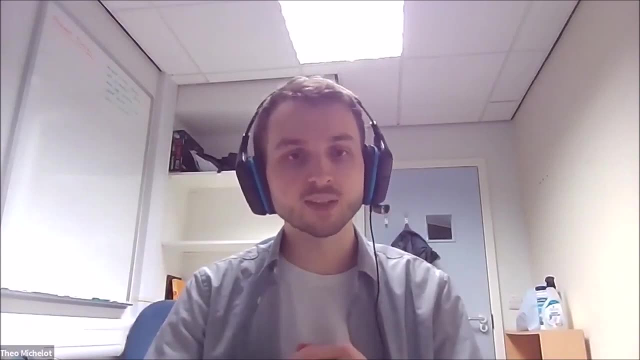 So it's classified it as being in state one, but really it's really really close right, Whereas in other cases it might be a 99% chance of being in state one and 1% chance of being in state two. 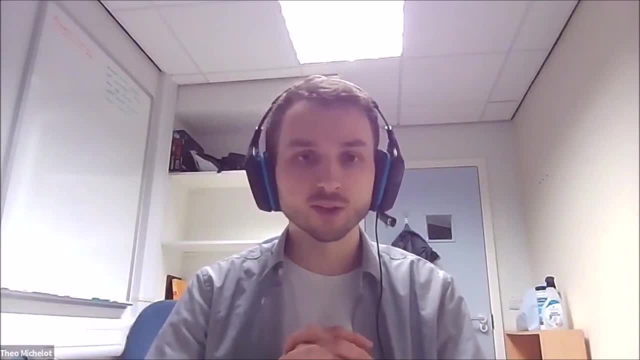 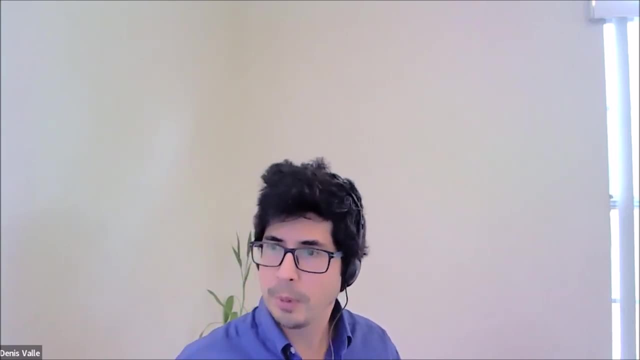 And so it gives you a better measure of that uncertainty. Okay, So somebody is asking here: can you review your typical model evaluation steps, So, in addition to checking pseudo residuals? so how do you typically, how do you typically evaluate the performance that fit of the hidden Markov models that you run? 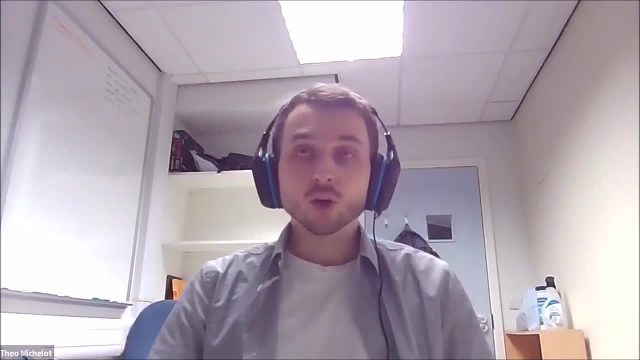 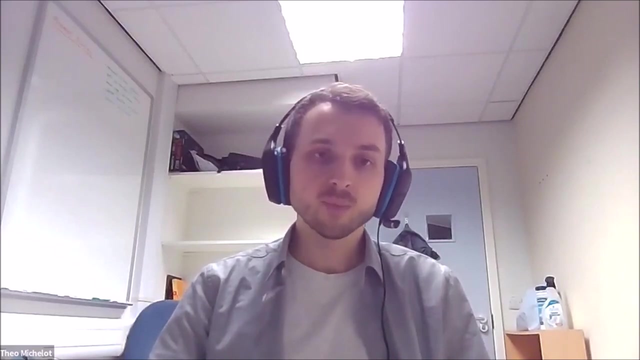 Okay, That's a really good question, A really a complicated, a difficult question, I think. So I think pseudo residuals are often the first place. Pseudo residuals can tell you things about whether you've missed something in the distribution of step lengths. 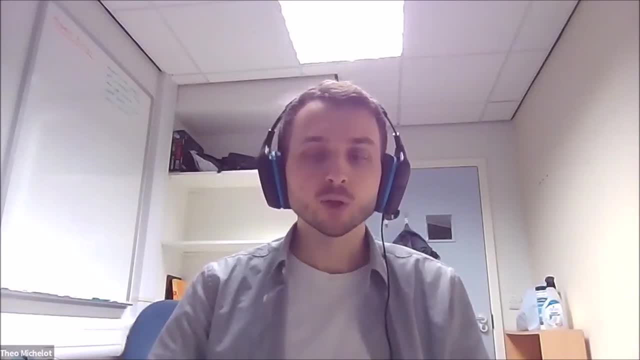 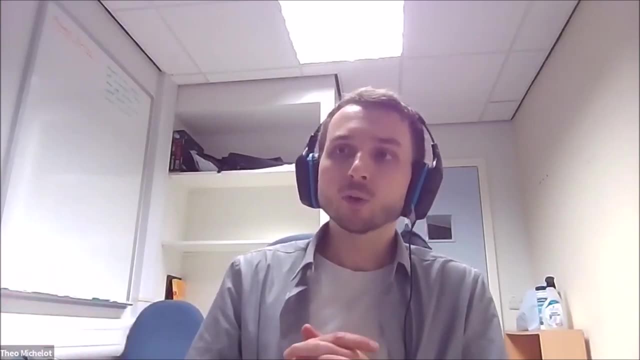 or distribution of turning angles. So, for example, if you don't, you know your distribution of step lengths is very heavy tail, then you haven't captured that. It's going to tell you that, or something like this. It can also tell you about residual autocorrelation. 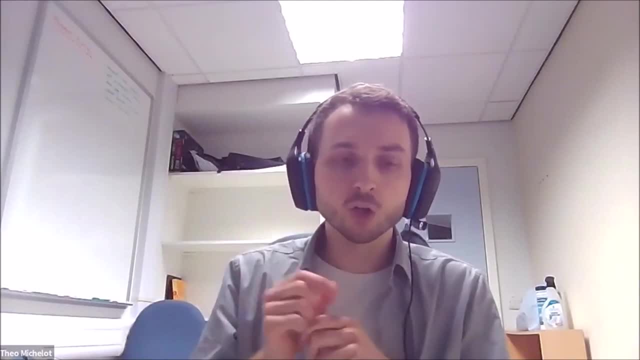 And because I had to go quite fast, I didn't mention that. but it gives you a little autocorrelation function plot for the pseudo residuals that you could use in a similar way to what you would do in linear regression or something where what you want 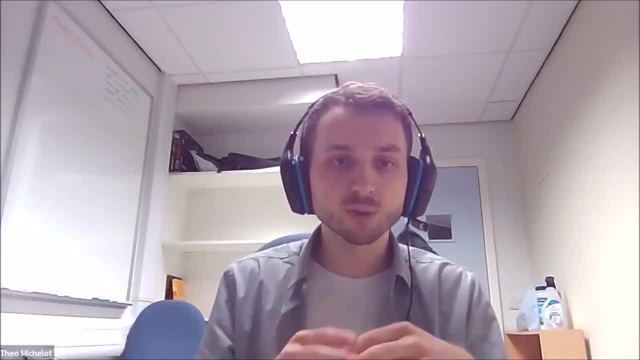 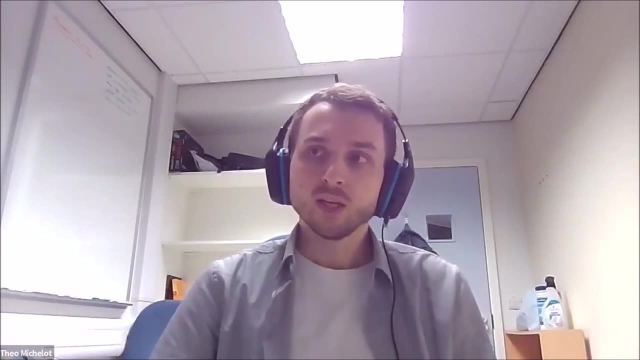 basically is that you don't want residual autocorrelation. If there is residual autocorrelation, it means that there is some kind of autocorrelation in your data That isn't captured by the model, And that's going to happen fairly often. 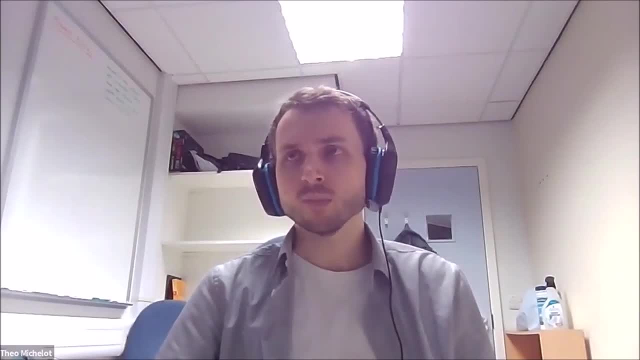 Often it's not really a problem, but it's good to be aware of So pseudo residuals. I think it's a good thing to just visualize, the model, visualize. That's why I spent quite a bit of time showing all those plots. 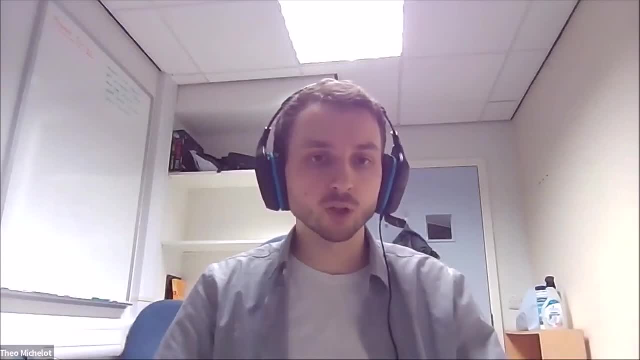 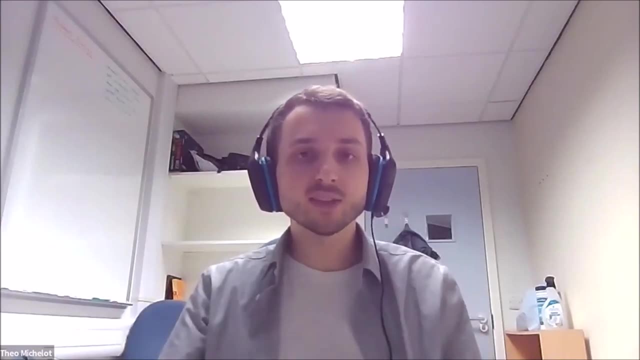 I think you know, looking at your decoded- like color coded- tracks, looking at your distributions, I think this helps really give you an idea of whether the states that you've identified with this model Are well-defined, whether they overlap or not. 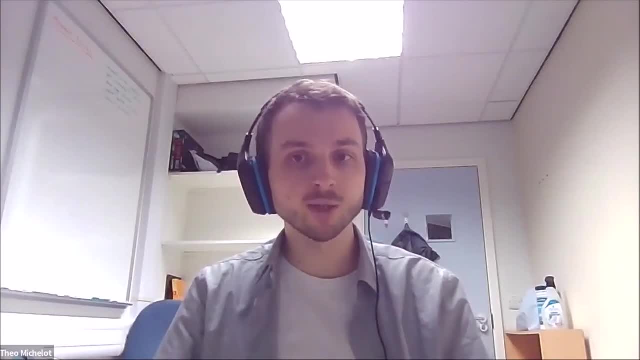 Hopefully they don't overlap too much, Otherwise the interpretation can be a little bit tricky, And then it helps you with the ecological interpretation as well. Helps you say: well, I think for this species, slow movement, it's got to be resting. 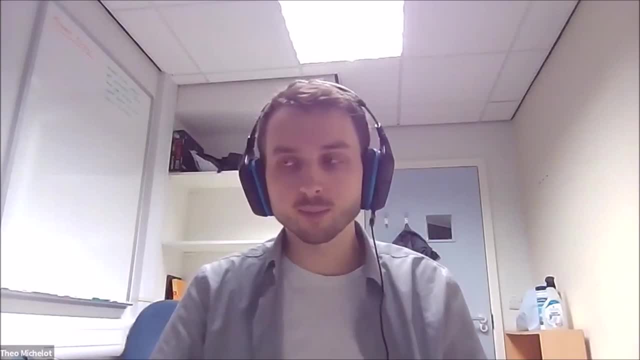 And fast and very direct movement. it's got to be transit or something. So I think quite a bit of kind of almost exploratory analysis with the output of these models. One very last thing that I wanted to mention, and this is not used a whole lot in practice: 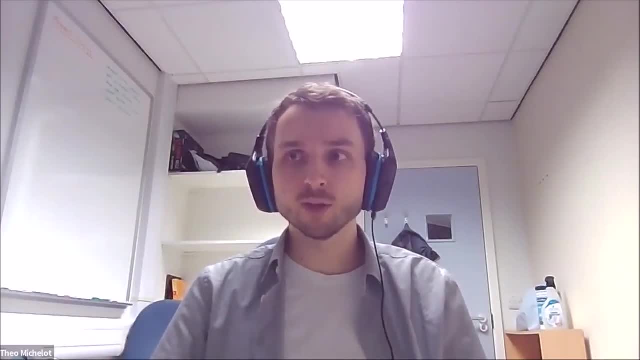 but has been recommended in theory is to use something called posterior predictive checks on using these models, And the idea there is that you would simulate trajectories from your fitted model, And you can do that. There's a function called simdata in Momentum where you can put as input just your fitted model. 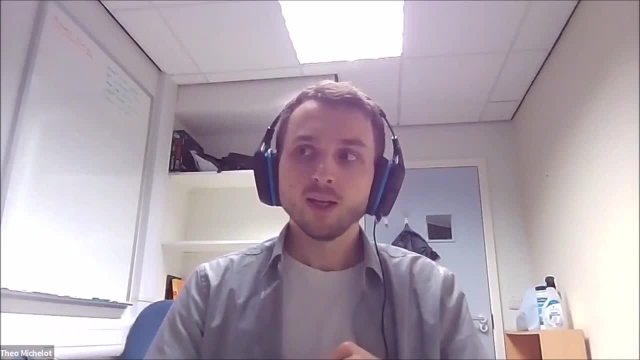 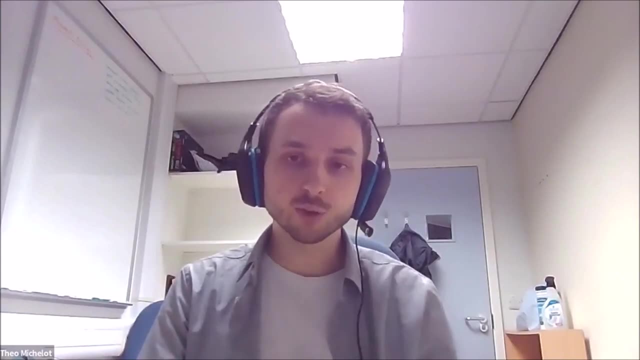 And it will generate trajectories from that model. And the reason that this can be useful for model checking is that you can look at features in the simulated tracks and compare them to features in the original data And they can give you an idea of what's been captured. 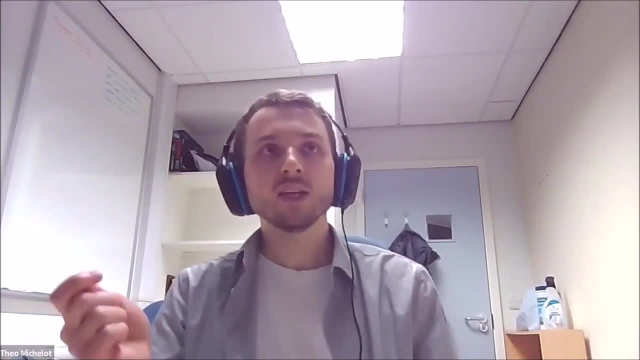 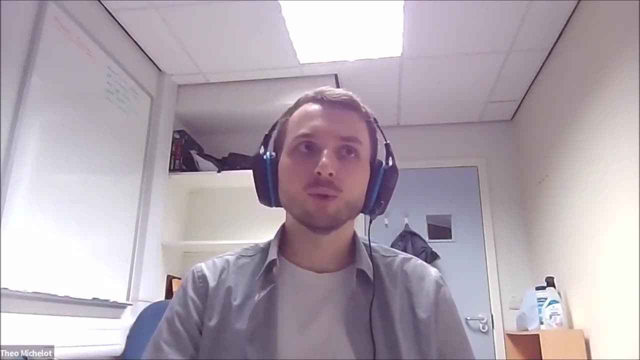 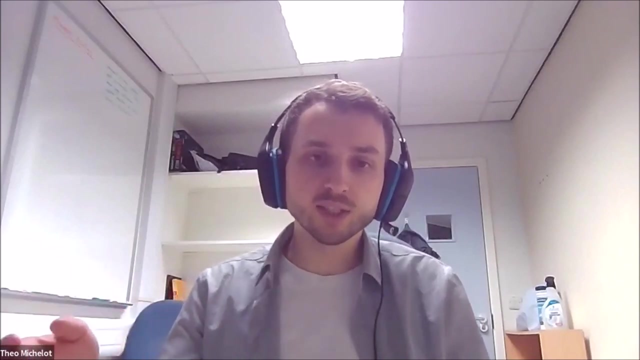 and what hasn't. So if you simulate data tracks and you realize that the animal just goes way too fast compared to the real animal, or you realize that the animal I don't know, I mean things like that. Yeah, like, if you identify features in the simulated data. 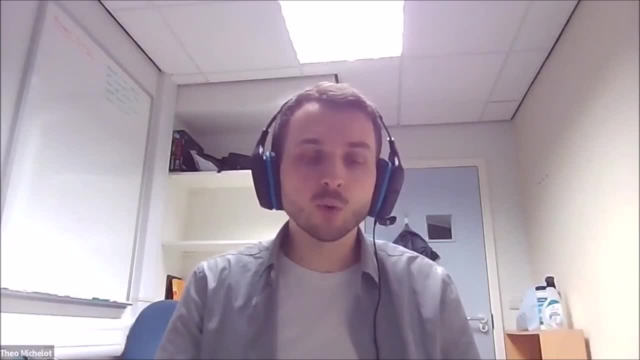 that doesn't mean that you can just go and do it. Yeah, So don't look like features of the real data. Those always point to things that you've missed in your data. OK, So yeah, these are the main directions I would explore. 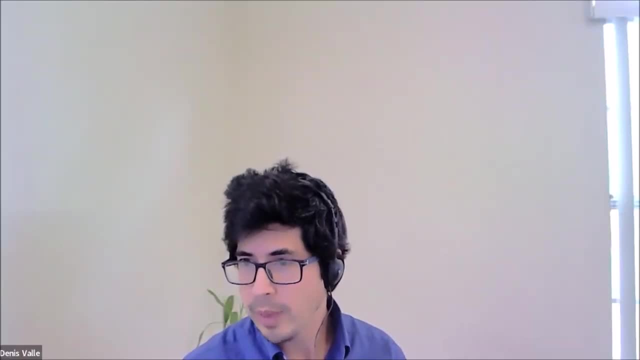 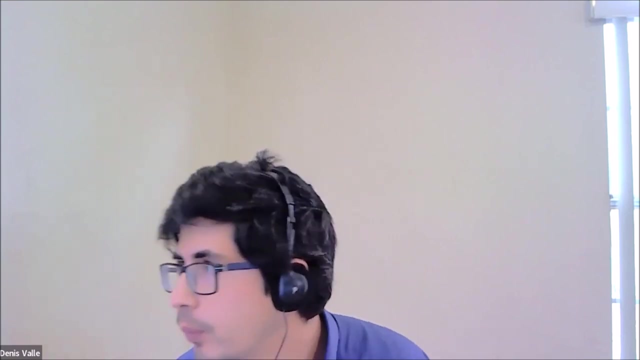 Great, Awesome. So there's a question here As an alternative to path filtering. so if you have incomplete but very accurate GPS trajectory data, what are your thoughts on data imputation and how do you do that? Where did that go? 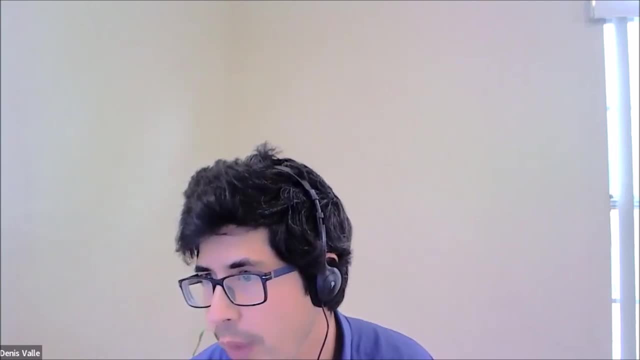 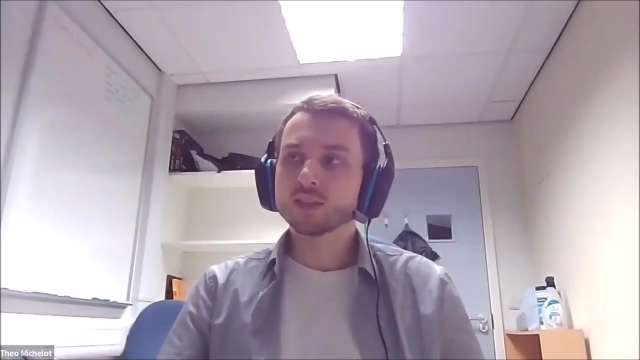 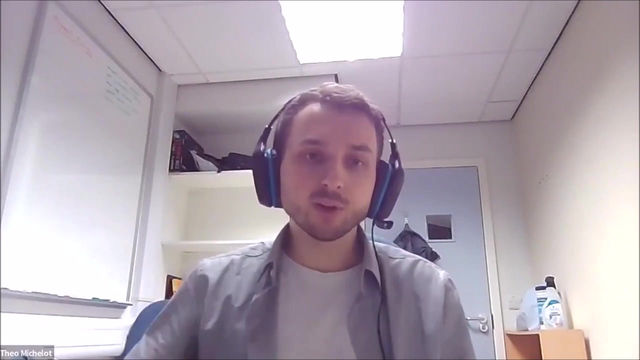 To reconstruct paths. are there tools to do that currently available? Any recommendations when multiple movement phases- searching, resting- exist? OK, I think there are several parts to this question, So I was using the term filtering a little bit, maybe a little bit liberally. 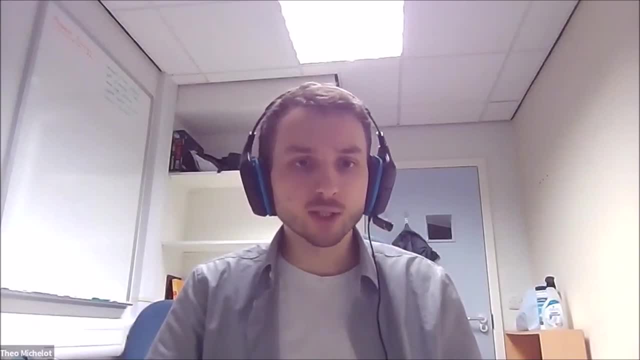 I was also referring to more generally regularizing a data set. So, for example, that's what I used with the elephant data set. There was no measurement error, or I assumed no measurement error, But I could still use packages like foie gras and crawl. 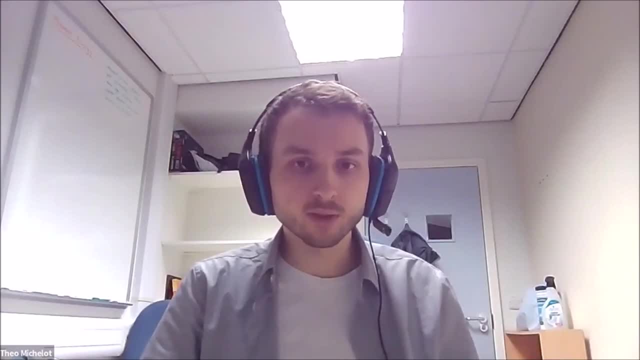 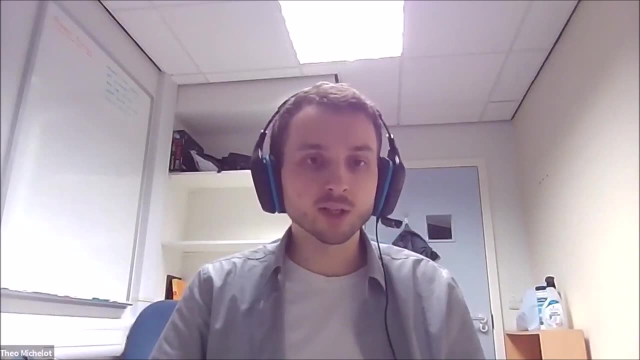 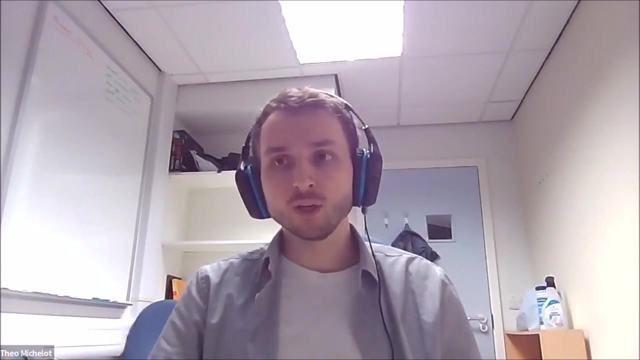 to regularize the data set. So I think that's probably similar to what you were referring to for these imputation methods. So that's where I would direct you: foie gras and crawl and similar methods. The second part of the question about particular tools. 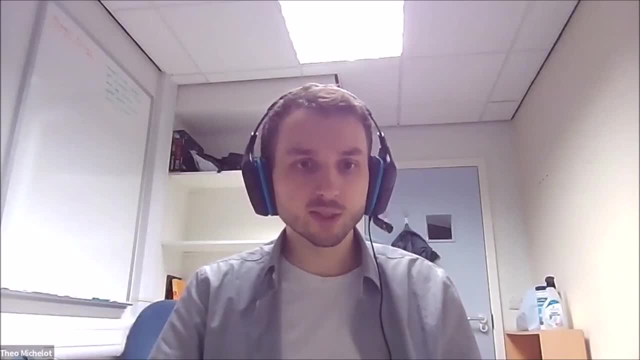 in the case where we know that there are different movement phases. I think that's a very difficult question. I don't actually know that there are good tools to do that, And I can say maybe one more word about this, which is that 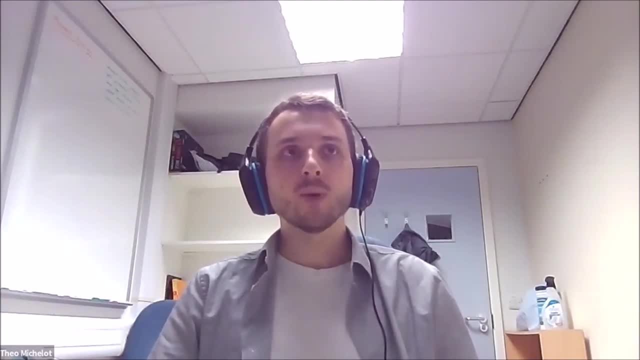 and I think that's what this question is hinting at. those predicted paths or even, in the case of multiple imputation, all those plausible paths that we're generating, are generated from a state-based model that doesn't have built-in behavioral states. 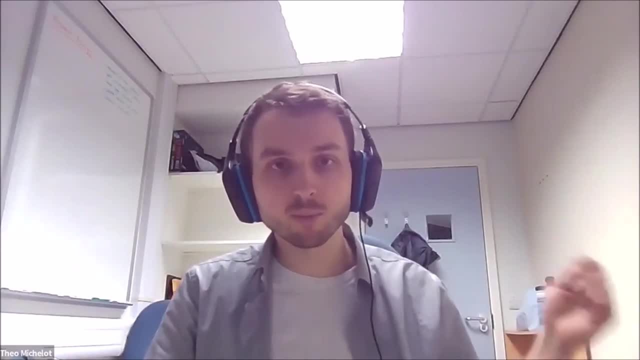 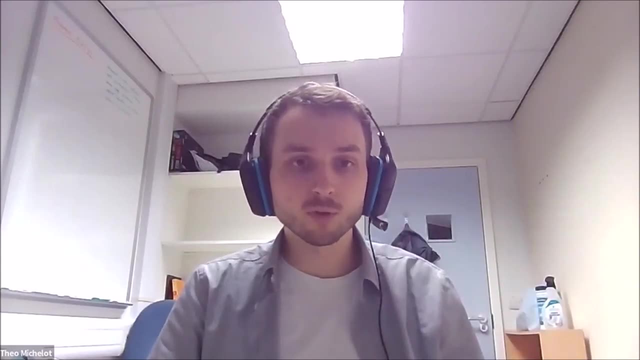 That state-based model just assumes that there's one type of movement, And so it's going to predict those imputations using just that one type of movement, Whereas what we would want, because we know that there are several types of movement. that's why we're fitting an HMN. 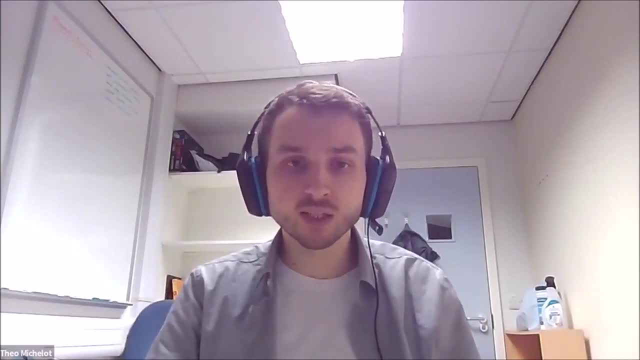 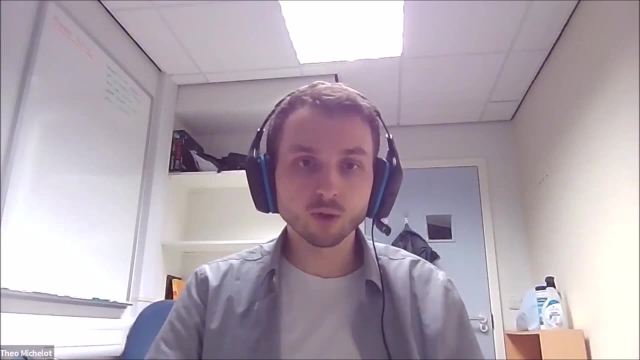 We would want a state-based model that can capture that heterogeneity in the movement that comes from different behavioral states, so that we can predict the trajectories or we can generate those plausible trajectories over those long gaps in a way that accurately or realistically represents what the animal could have done in that gap. 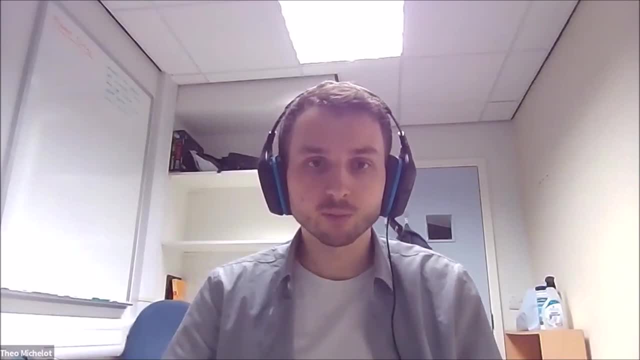 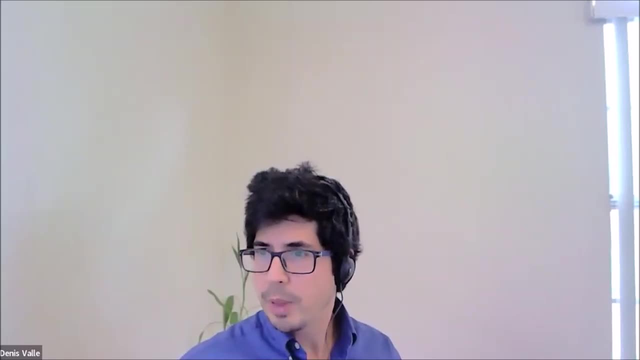 And I think that's again an active area of research. There's no current kind of easy tool for that Perfect. How does the Markov model perform at differentiating behavioral states for data that are collected at different time intervals, say a couple of minutes interval? 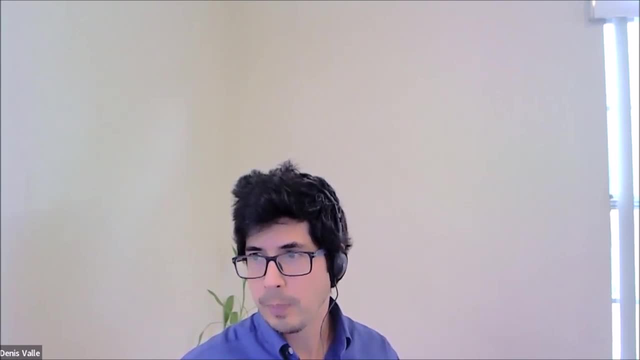 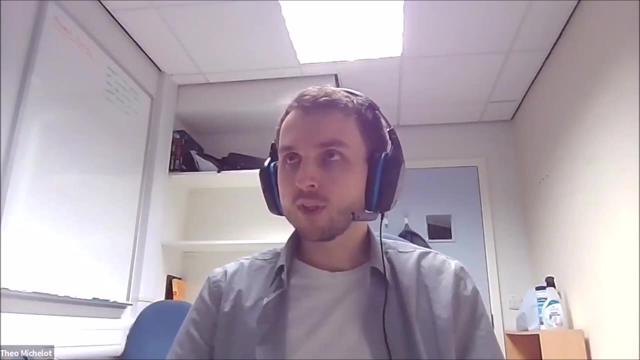 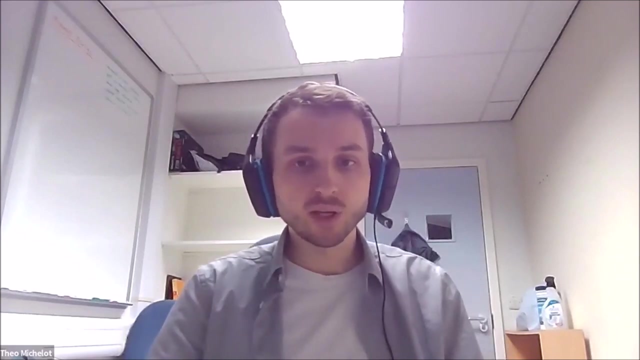 versus hourly interval. OK, So I'm not exactly sure what the question is asking. If you're asking basically, does it work better at differentiating between behaviors that define time resolution or course time resolution? I think it depends a lot on your data set. 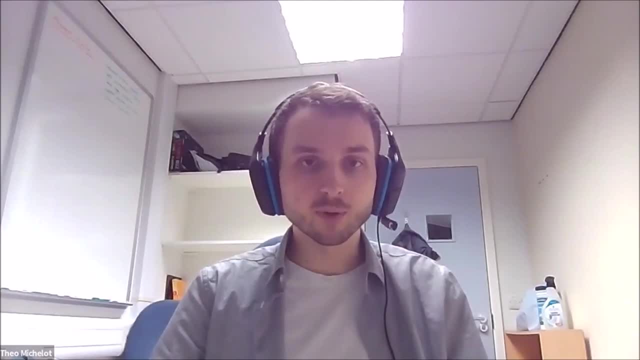 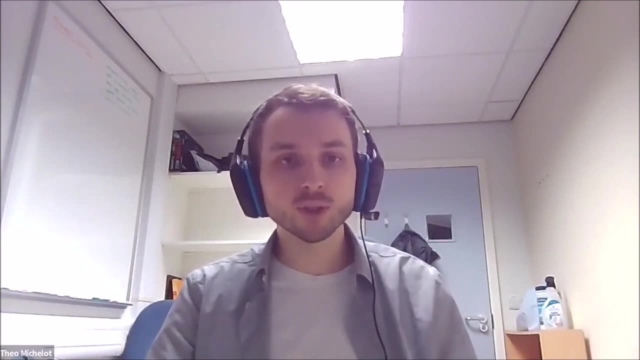 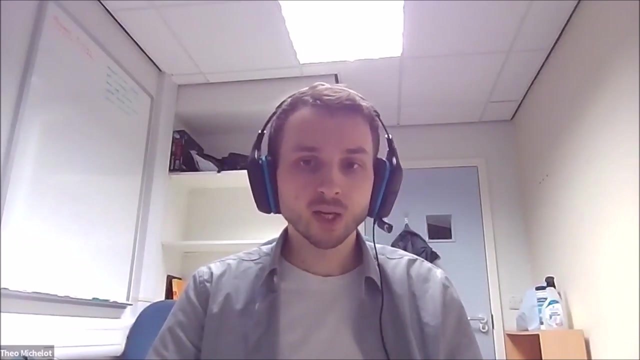 One thing that's really important with these models is that the interpretation of everything depends on the time interval of your data. So if you have observations, it's not uncommon for some systems to have only maybe one observation every day or something, And maybe from that you can still. 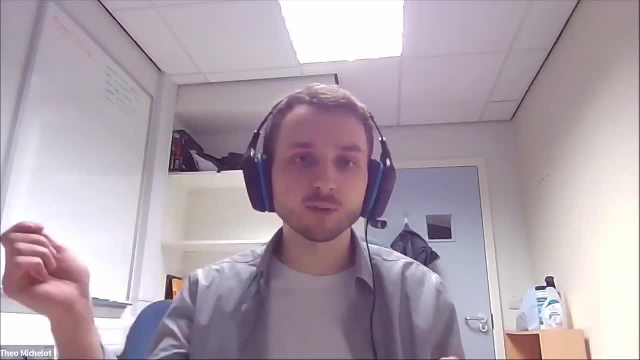 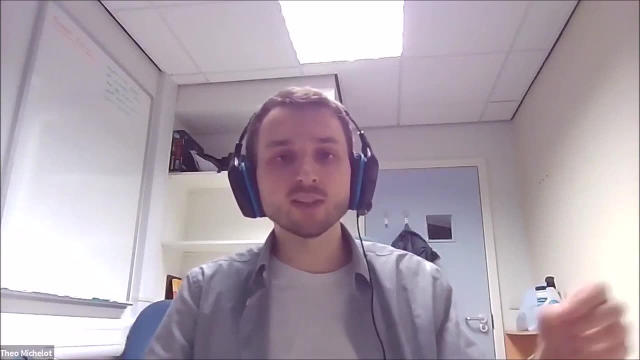 pick up some behavioral differences. You can pick up maybe migrating versus not migrating or something. But obviously at that time resolution you wouldn't be able to differentiate between I don't know- fine scale foraging and searching for food and all those kind of finer scale. 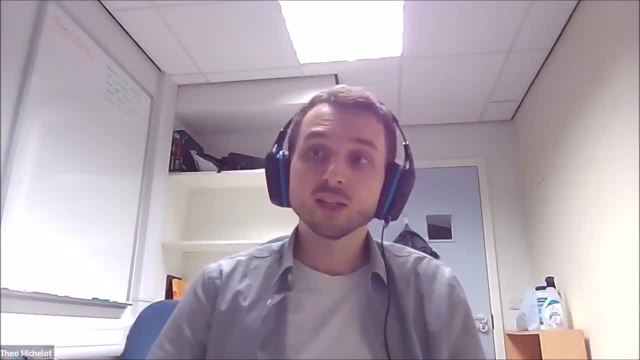 OK, So that's one of the things that's really important to consider when you're looking at scale behaviors. On the other hand, from your two-minute data, you're probably not going to be able to differentiate between migrating and non-migrating. 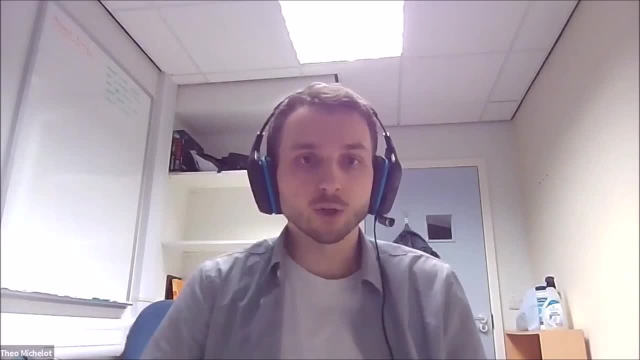 because that's just too coarse of a scale. But you'll be very good at differentiating between, I don't know, very slow movement, very fast movement, the kind of everything in between, depending on what your animal is doing. So I think the question of whether those models are better 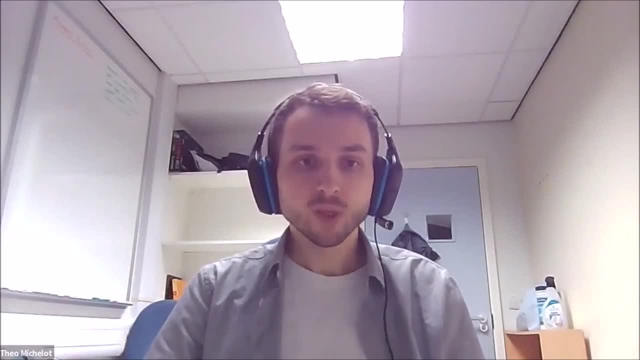 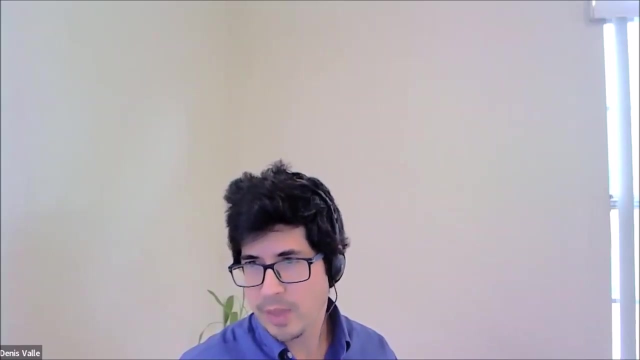 or what time resolution those models are better at doesn't really have an answer, But you need to remember all the time that the interpretation depends on the time resolution. If I could just add, it seems like part of the challenge would also be thinking about the amount of noise in the data. So if you have very short time intervals, you might have a lot more noise than signal, But then if it's a very long time interval, then you have some noise. So, assuming a straight path, I guess it depends how exactly you're modeling this. 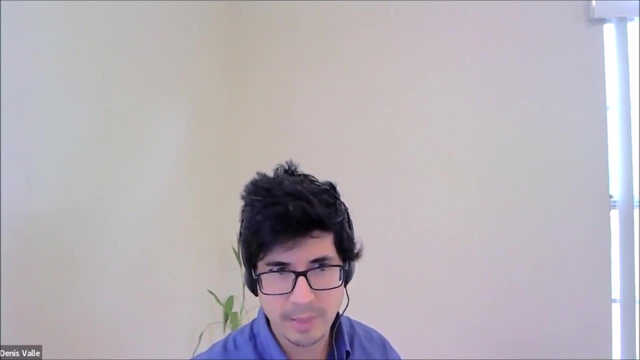 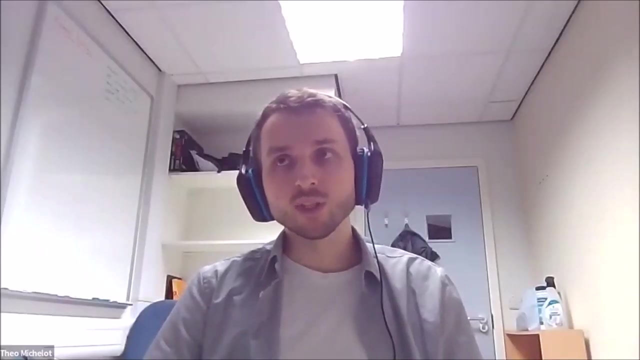 but which may or may not be accurate. So that's another sort of trade-off. Yeah, that's a good point, Thanks, Yeah, Is there an advantage to using fordRAW over crawl for data regularization? No, The reason I showed both is that I don't know. 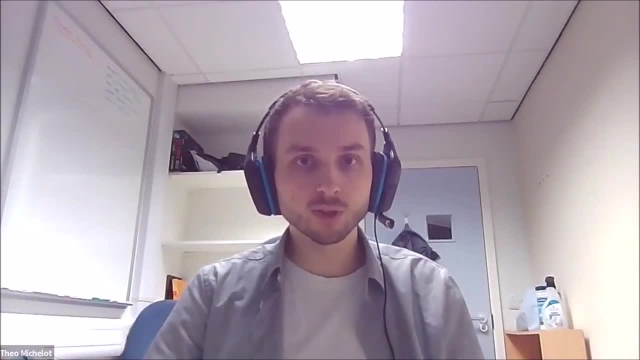 I think it's best for people to know of all the different tools that are out there And potentially now you can go and read the papers and read the vignettes to kind of find out exactly what the differences are. They use pretty from a mathematical perspective. 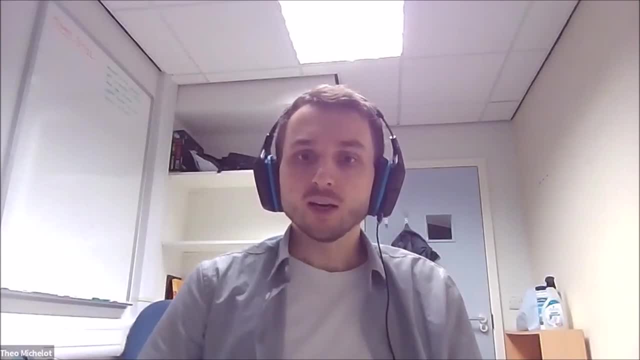 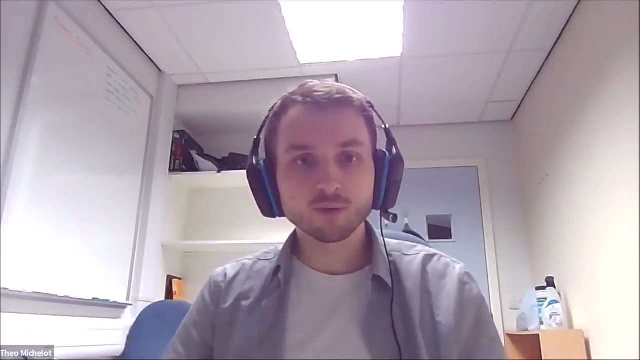 they use pretty similar methodology. Maybe I shouldn't say too much about my personal experience because it might not apply to you. In my personal experience I think I found that crawl was a little bit more fiddly from a numerical perspective. Sometimes it's just a little bit harder to fit. 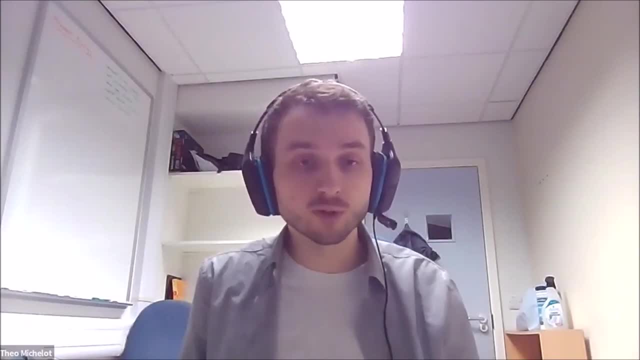 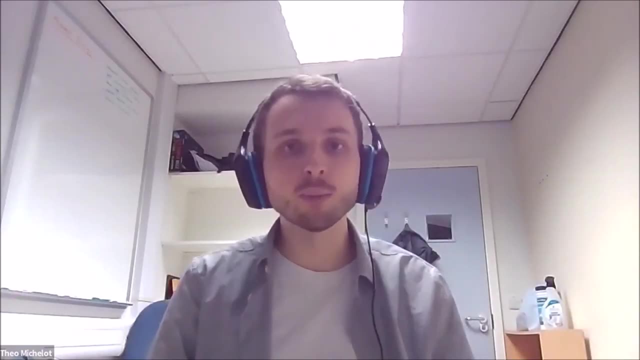 a crawl model to your data. Yeah, Yeah, If the crawl model doesn't fit well or if for some reason it doesn't converge or something, then you're not going to be able to get those predicted locations, or maybe those predicted locations. 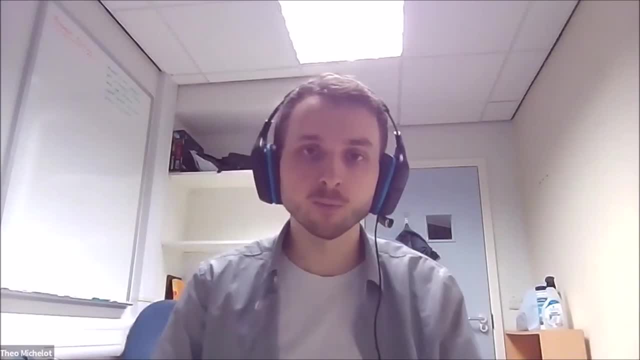 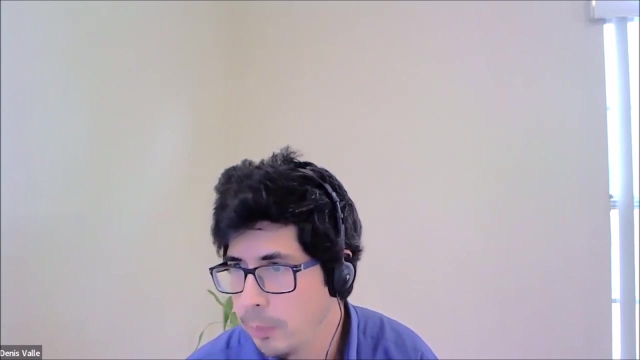 won't make any sense at all, because the model will not make sense at all. So not really, But you might want to try both. All right, Great, I got that. you suggested to split individual trajectories into long gaps, So you artificially create multiple individuals. 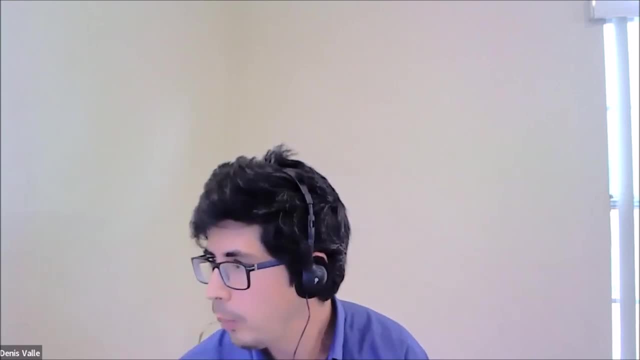 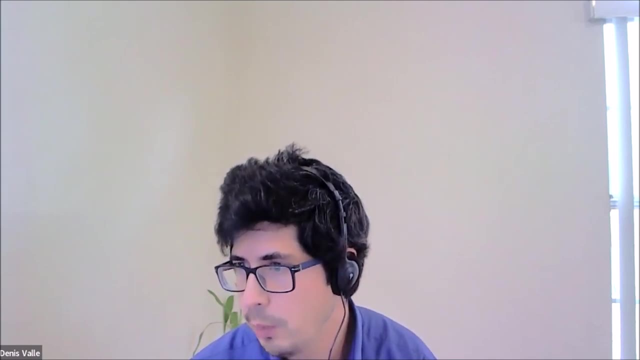 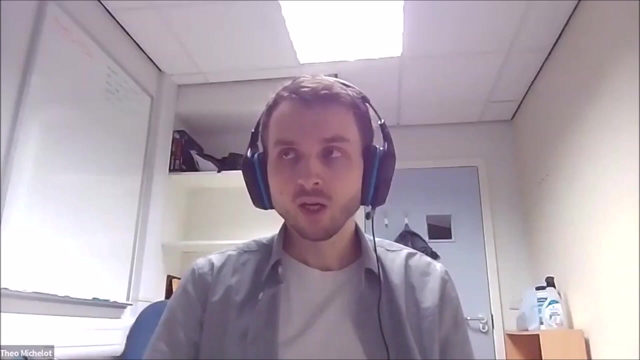 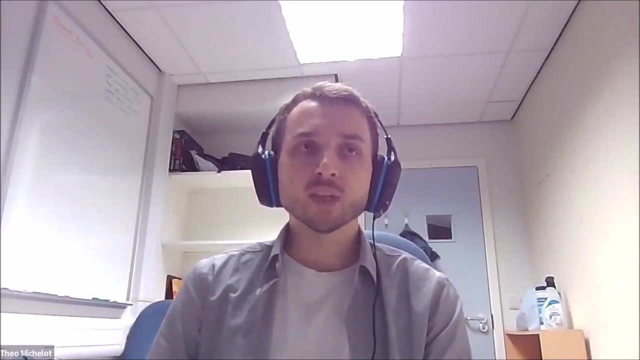 that are actually just one. How would it impact your estimates? How would we account for the nested structure trajectories nested within individuals? Is it possible to include some sort of random structure? OK, So one thing that I maybe haven't emphasized enough is that the way 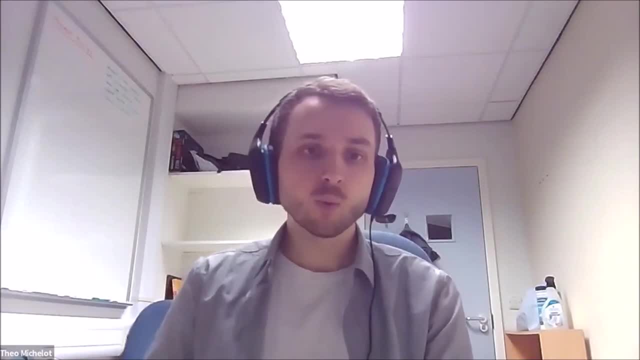 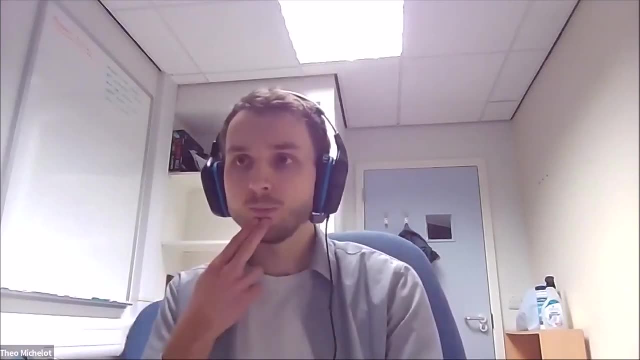 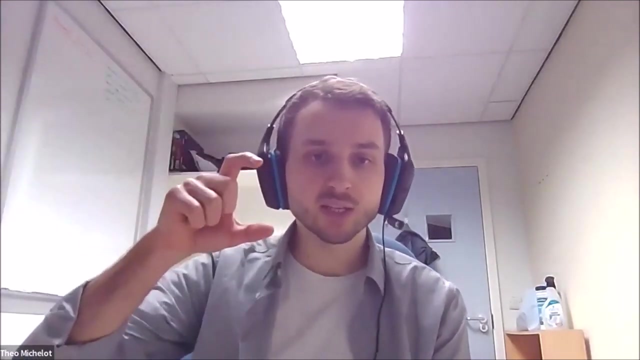 These models work by default is that when you pass your data set with that ID column that tells you which track or which individual or something it is actually, the model doesn't really use that almost at all, except just to know that there isn't actually. 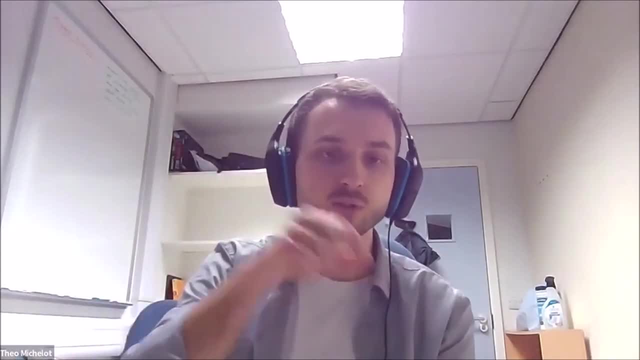 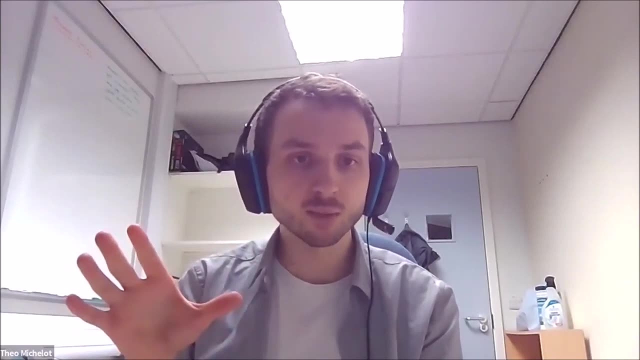 a step length between the last observation of the first individual and the first observation of the second individual, But the model is still going to fit just a common shared model to the particular data set. The package is still going to fit a shared model to all individuals by default. 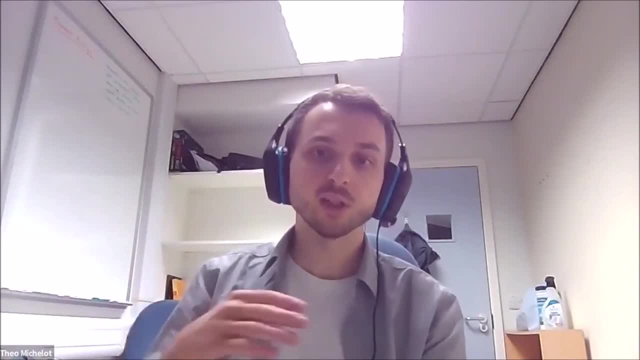 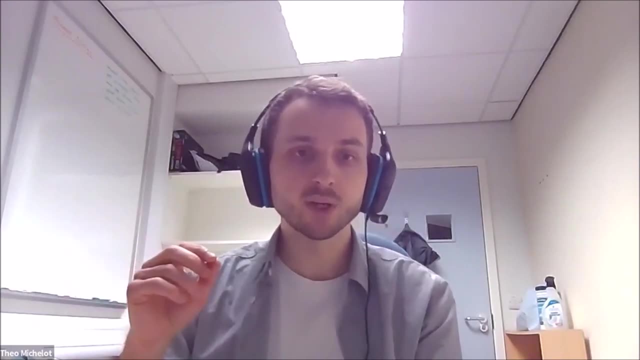 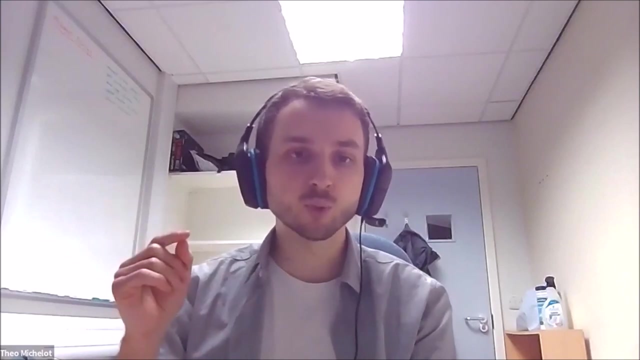 And so you'll get what we call pooled parameter estimates, because they're the same parameter estimates for all individuals. So those parameter estimates that I was showing in R before they were estimated from two different individuals and from nine different subtracks And it just returned one mean speed in state one and one. 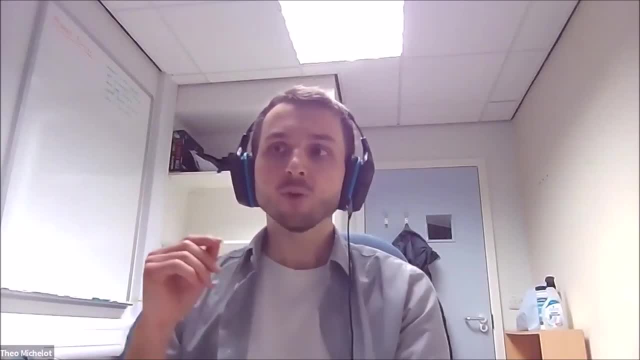 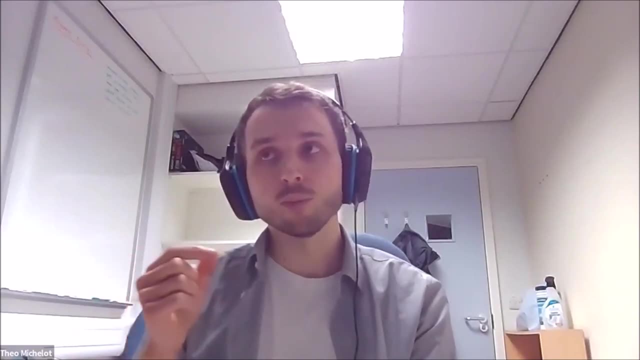 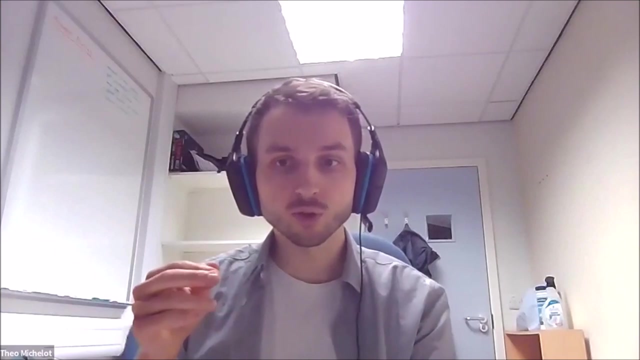 mean speed in state two et cetera. If you want inter-individual kind of heterogeneity, the kind of simplest way or the main way to do this in Momentum or in MoveHMM is to just use fixed effects. So you could include something like a fixed effect of ID. 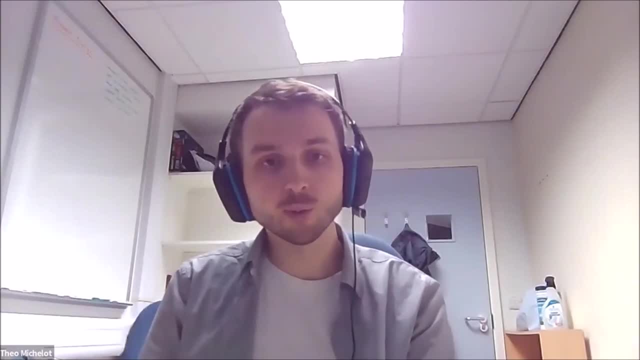 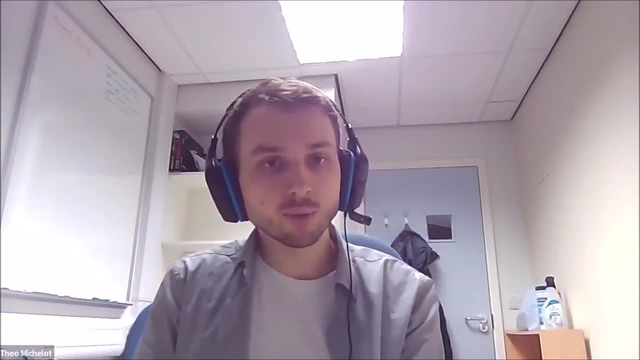 on the transition probabilities, And then you would be saying that the probability of switching between the different behaviors depends on which individual you're looking at. It's a little bit tricky to implement random effects, sorry, in the context of hidden Markov models. 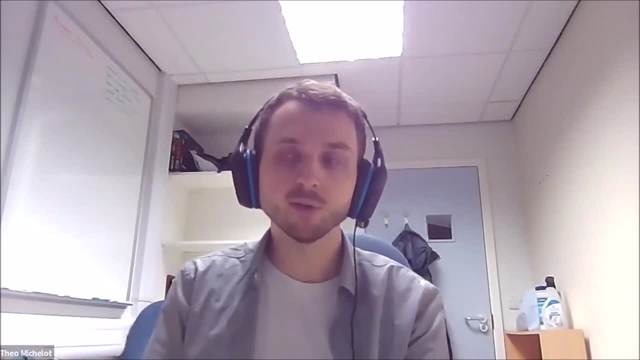 So that's why those packages don't allow for them by default. I've been working with someone else in St Andrews. We've been working on a package called HMMTMB that implements hidden Markov models with random effects, And so then you can specify pretty flexible formulas. 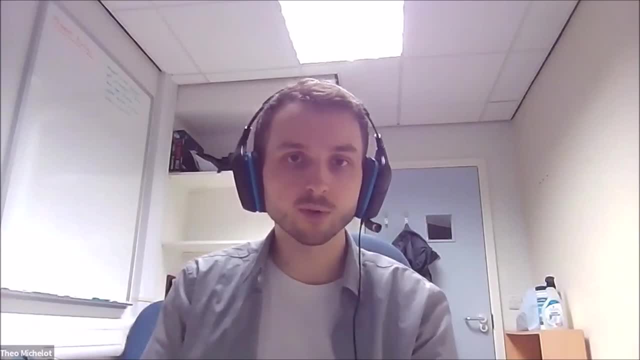 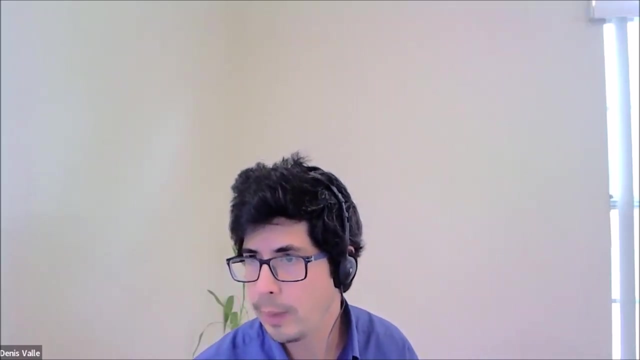 where you could have a random effect of individual or random effect of whatever you want on the transition probabilities. But that's still a little bit more kind of work in progress, Right? So we'll have to wrap up soon. I'll just put one more question and then we'll wrap up. 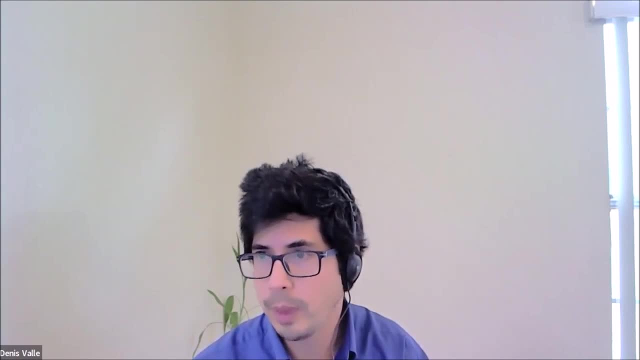 There are many, many more questions, But unfortunately I think we won't be able to go over them. Does MoveHMMM, does the package, have instructions on how to model movement parameters like step lengths and turning angles as a function of covariates? 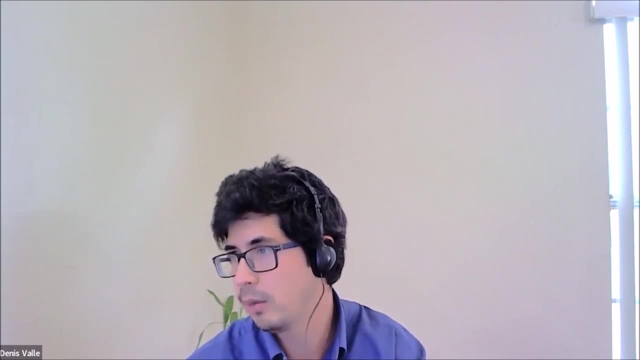 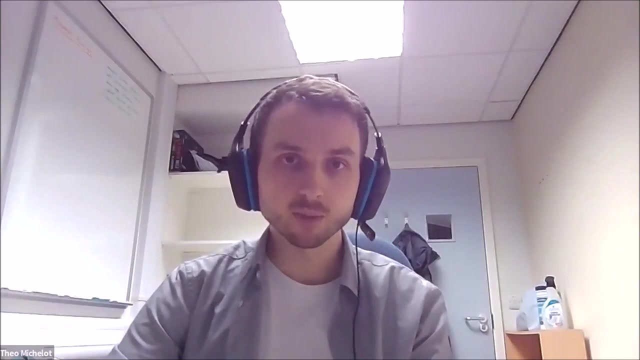 Just like you showed with the transition probabilities. but instead of the covariates influencing the transitions probabilities, they are influencing directly step lengths and turning angles. Yeah, So MoveHMMM doesn't allow for that, but Momentum does. Momentum has a way to do this. 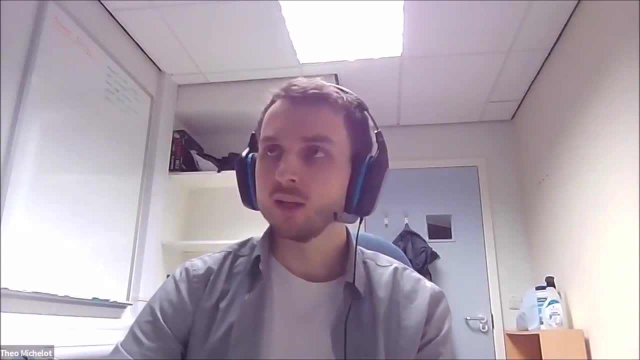 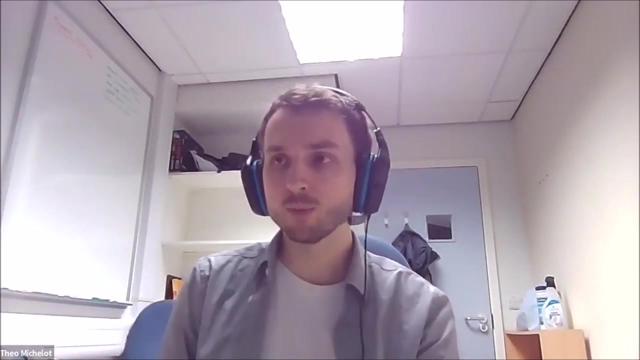 I think it's an argument called DM in FitHMM, So you'd have to refer to the documentation. Momentum has a pretty long vignette. It's a lot of examples of different data sets analyzed with HMM, with the code, And so you can look into that yeah. 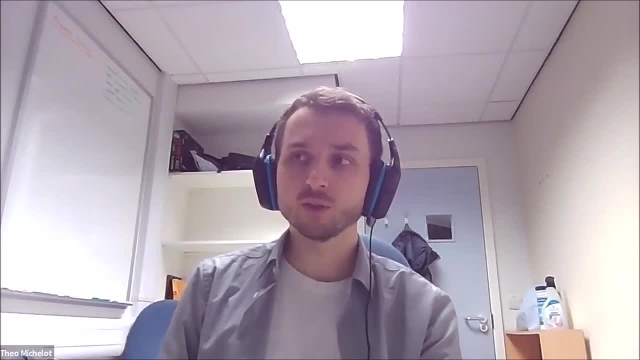 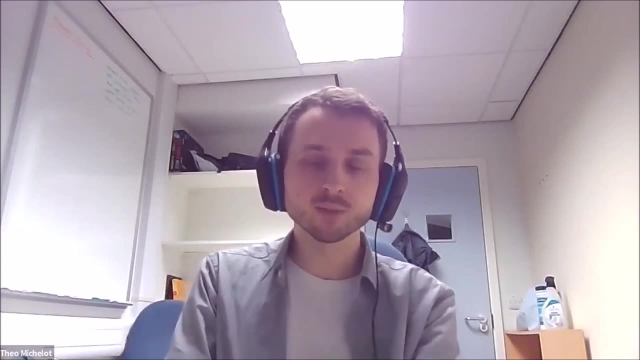 So Momentum allows for it. The reason that MoveHMMM doesn't allow for this and the reason that I think it's a little bit less useful in practice than putting covariates on the transition probabilities, is that when you include covariates, 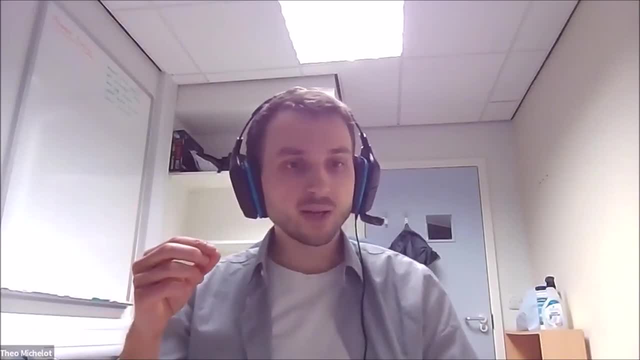